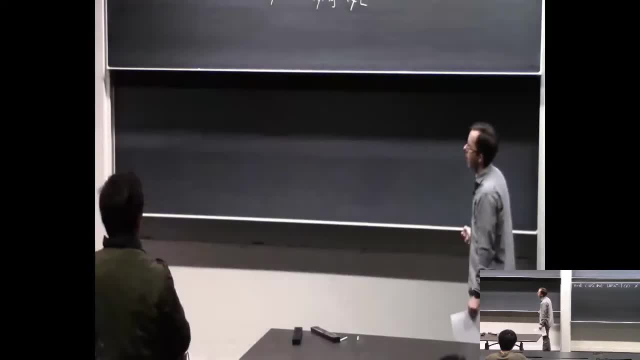 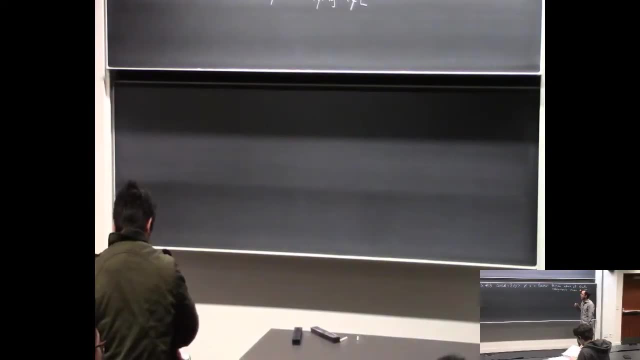 It's just inverting yes or no, But it'll lead us to some very interesting questions. So I want to start by recalling for you a problem that was on homework: five number zero. It was about this language. It came up in one of our earlier lectures about NP. 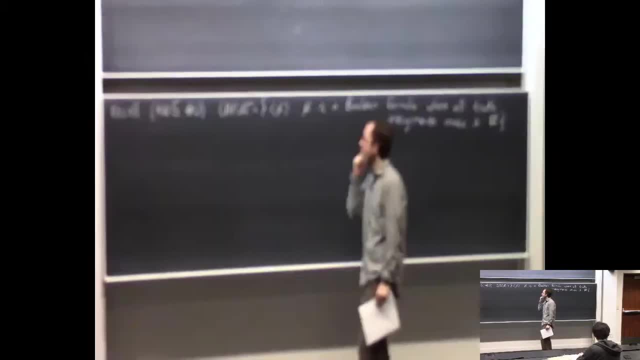 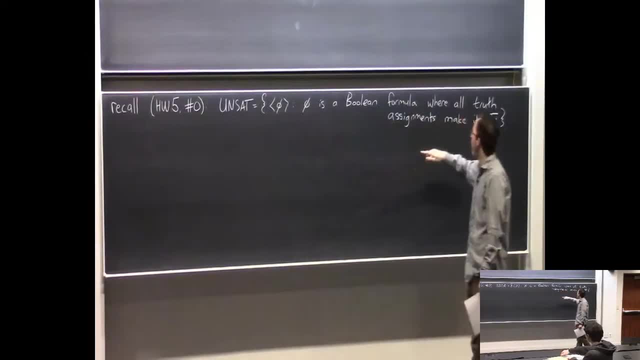 So this is the set of all completeness. And it's unset. So this is the set of all completeness. Now I could have written this as strings that are representations of Boolean formulas where every truth assignment makes them false. I could have also just written this as there: 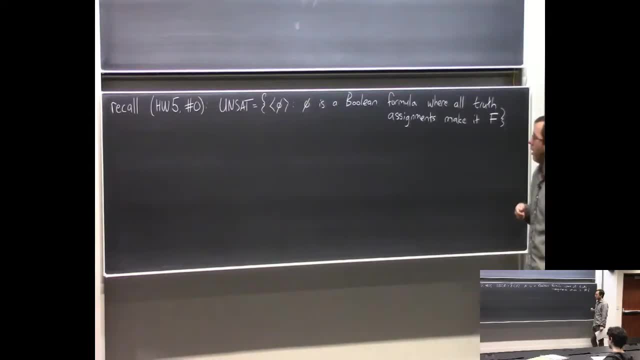 does not exist a truth assignment making them true. So they're not satisfiable. So it's just all the formulas that are not satisfiable. And today, in this lecture, I'm going to start using this notation, which normally I don't like that much, But I'm going to use it. I'm 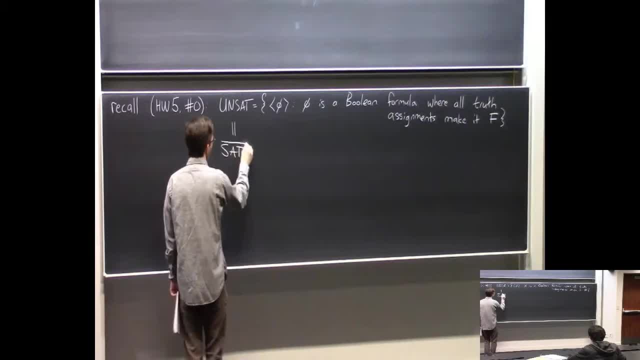 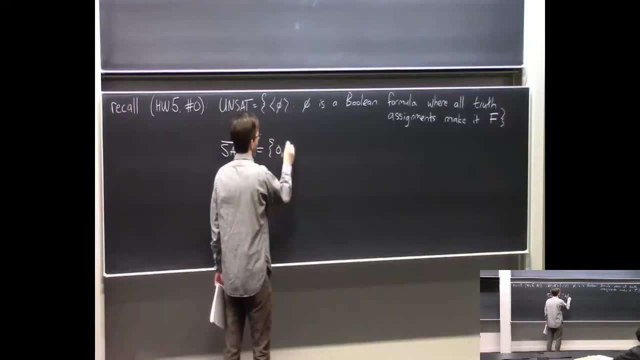 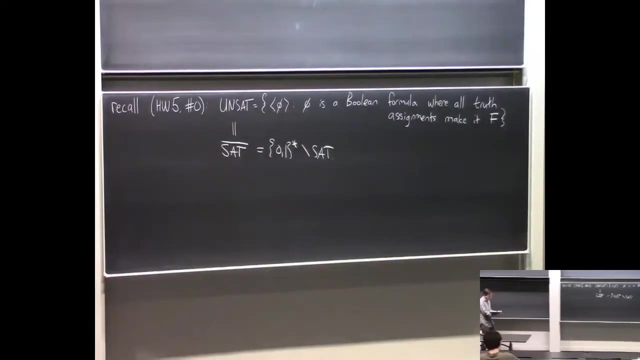 going to use the overline for complement. So this is literally all the strings that are in the complement of the language set. so it's just literally every string except those that are inset. so just all the unsatisfiable formulas and the question that this discussion of this classical NP that we'll talk about, 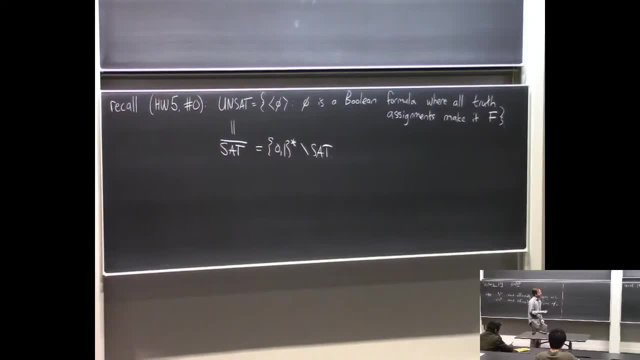 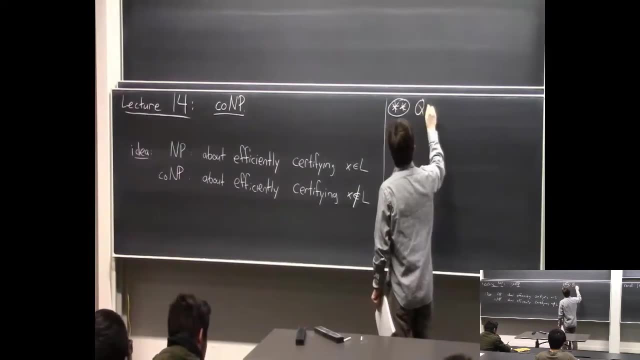 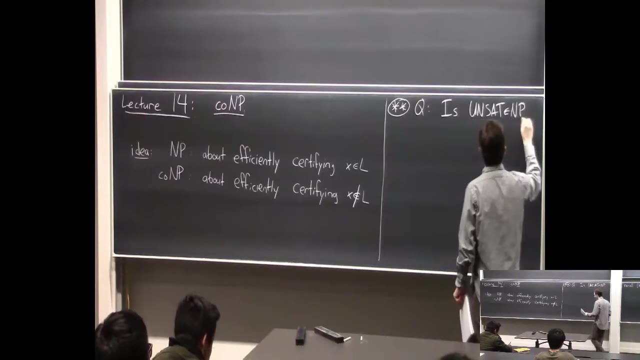 will lead us to is quite simple. it's actually even a simpler question than this homework zero question, which is this. it's quite interesting, so I'll put some stars around. it is unset in NP, and let's just think about it for one second. I mean see if we could imagine if it could be, or not. 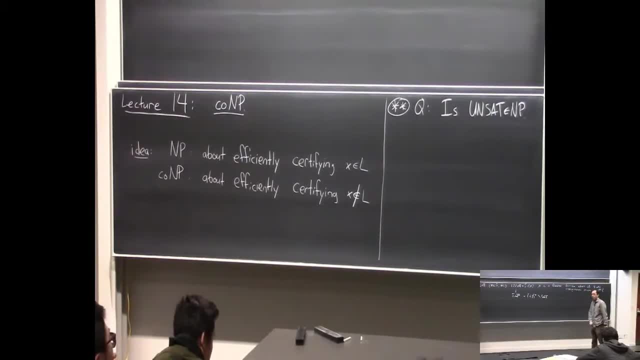 so we're trying to decide if this language- all the unsatisfiable formulas- is NP, kind of have to imagine how, like a prover might convince a verifier, or you might convince somebody that a given string was in unset so that a given Boolean formula did not have a satisfying assignment. 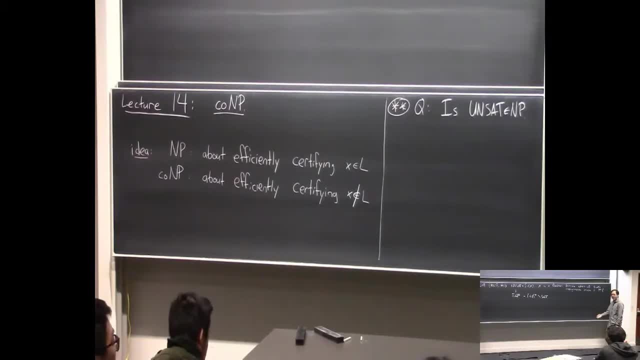 so you see if it's set, if it's unset. if it's unset, if you're trying to convince somebody that has a satisfying assignment, you can just tell them the satisfying assignment and the verifier can check it. but like how can you convince somebody that there's no satisfying assignment? 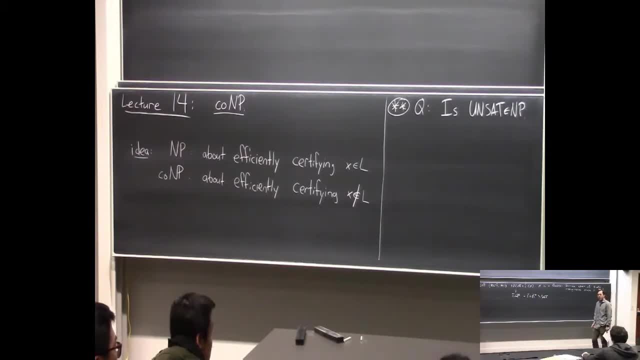 I mean it's not so clear, right? I mean you can tell them some assignments and say like check it out, these ones don't satisfy it. but in order to check that you're really in unset, you have to somehow know that no formula, sorry, no truth- assignment satisfies the formula. 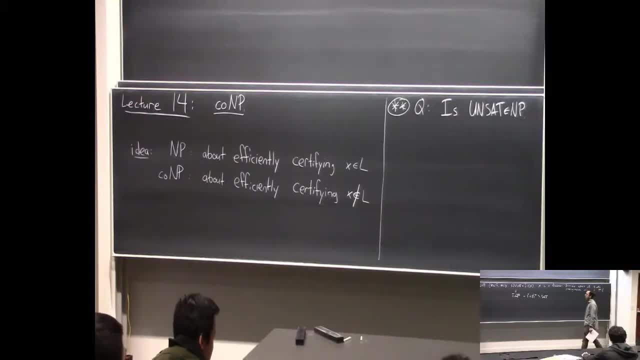 then it's just not clear how, like you know, a wise person could help you figure out how to do it- and you can figure that out- even if they gave you some kind of certificate, had the ability to give you some kind of proof. so this is what we're going to think about today. 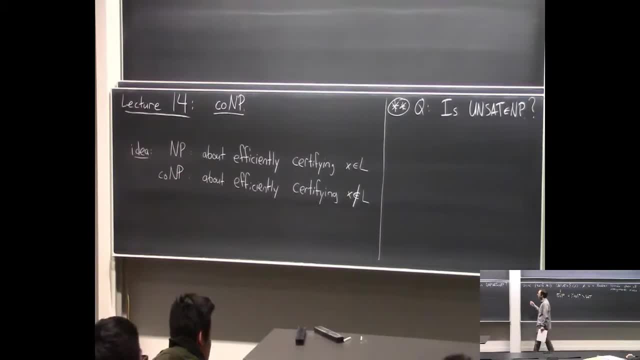 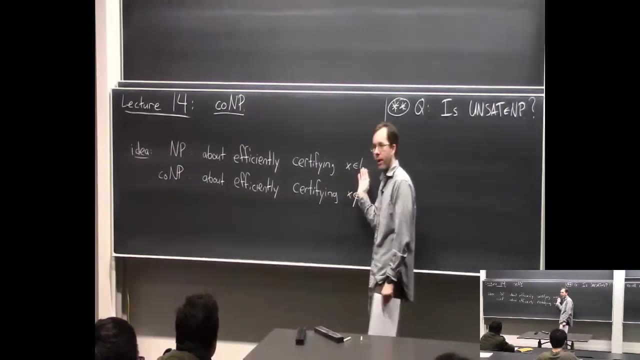 and it kind of arises as a question because you know, if sat's in NP, why is unset not in NP? well, there's sort of an asymmetry in the definition of NP. I've mentioned it a few times before, but it's because of this. I mean NP is all about certifying when a string is in the language. 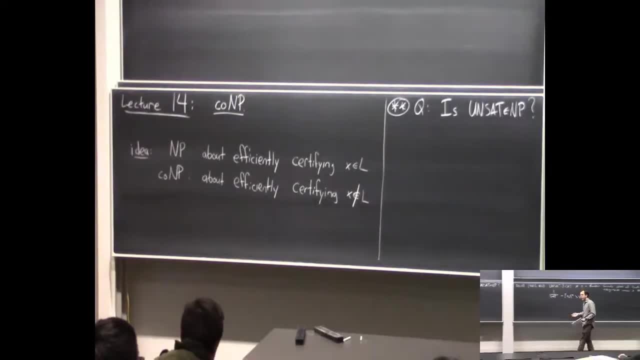 and you know if the string is not in a language, you don't have to have the verifier you know become convinced that it's not in the language. the verifier only has to get convinced when the string is in the language. so maybe, if that's not fully clear, 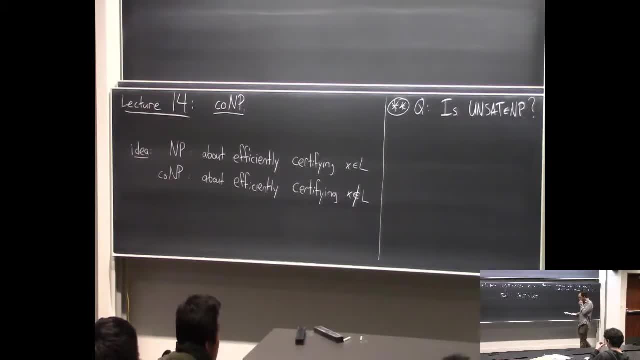 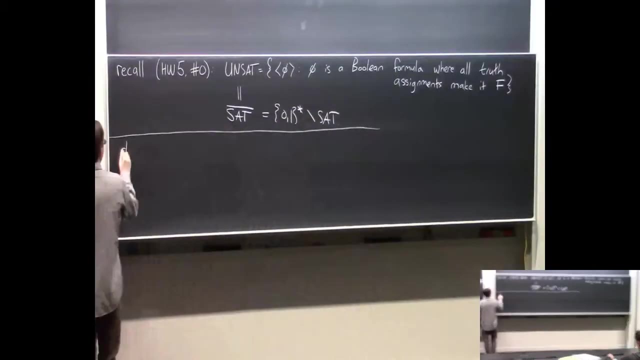 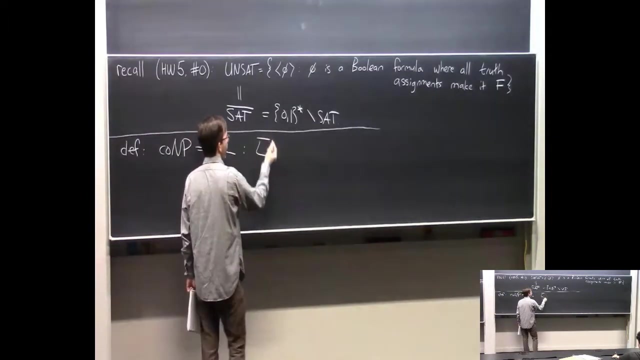 we'll understand it a bit better by the end of today. okay, so I want to just make the formal definition for coNP, and it's extremely simple definition motivated by this problem. so coNP is just literally all the languages, such that the complement of the language is in NP. 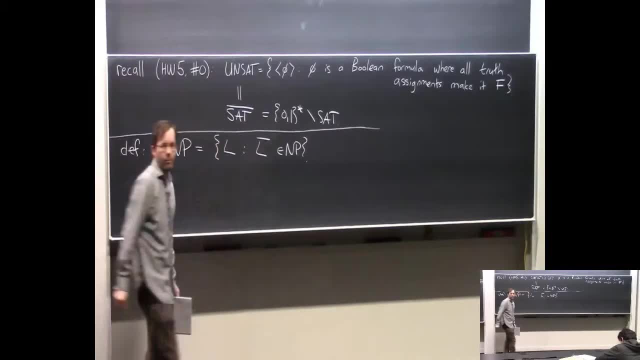 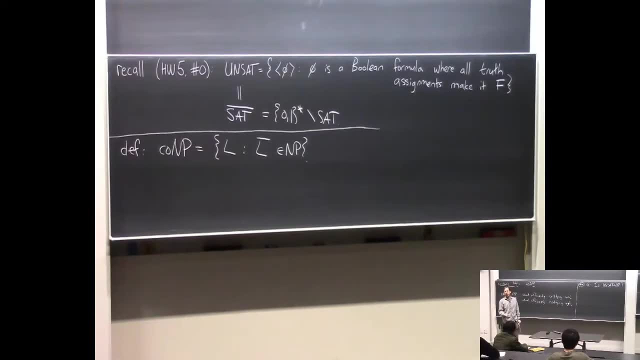 okay, remember, this is all the strings that are not in L. so that's it. that's the whole definition. so you can get the languages in coNP just like by taking any language in NP and take its complement. take all the strings that are not in that language. 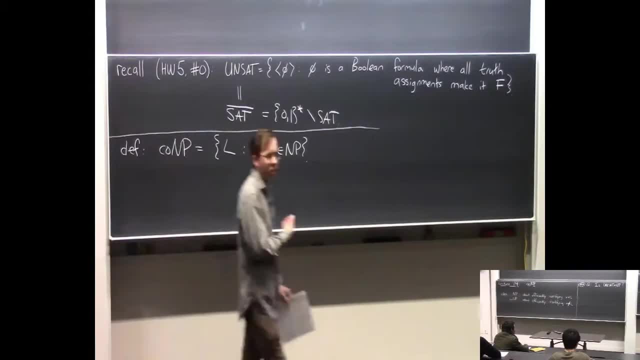 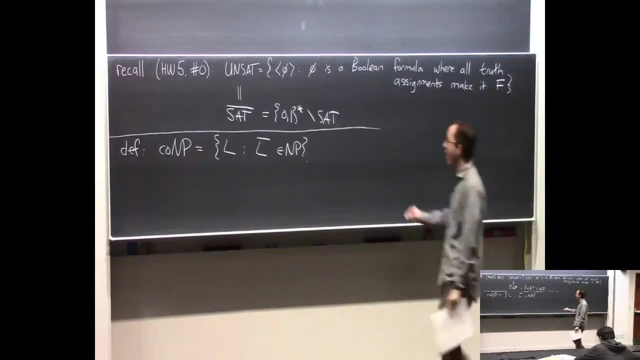 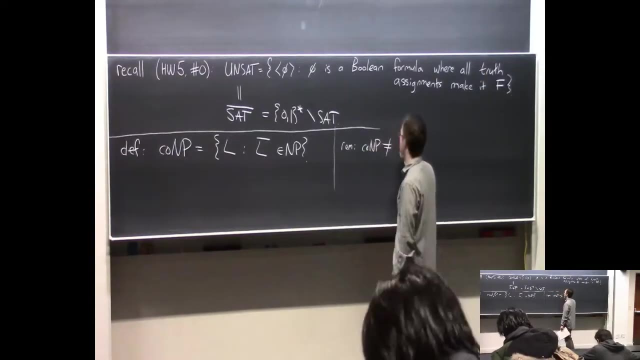 so, as I said, at first it's going to look like it's such a trivial definition, like what is the point of this playing around? but hopefully you'll see. let me also just remark that I mean- don't make this mistake- coNP is not the complement of NP. 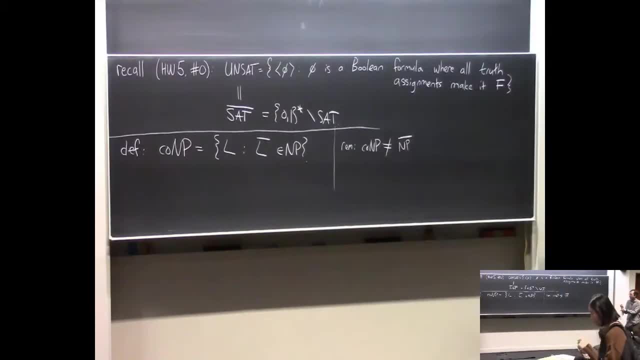 okay, so it's not all the languages that are not in NP. the negation is somewhere on the inside. and when you're talking about the language, can anybody prove this? there's a language that's in both of these classes. yeah, any language in P should be in both. 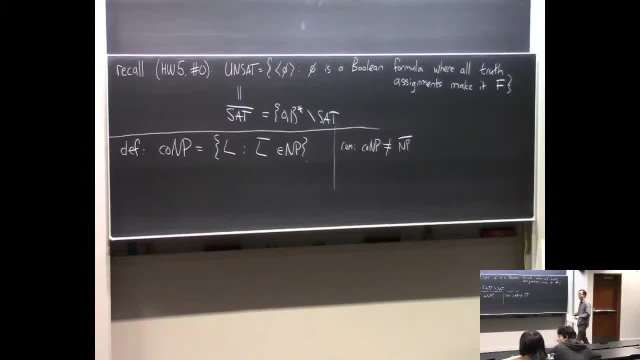 because the negation is also in P and in NP. you don't need the. that's true. we'll see exactly that. in particular, like the easiest language that's in P is the empty language. so the empty language is in NP. I mean, you don't even need the power of NP. 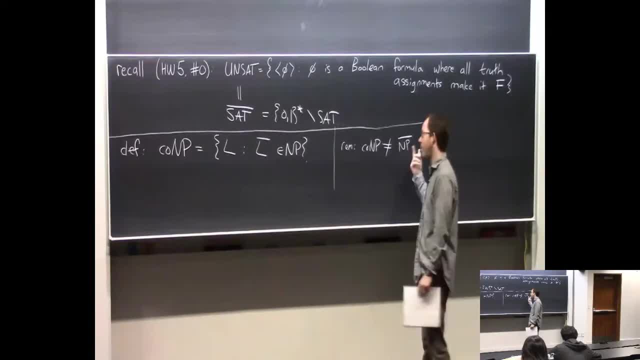 and its complement is the language of all strings which is also in NP. I mean, these are both in P, so that's in both languages, both classes. so anyway, we never consider this object. we don't care about this. great, okay. so I mean straight from the definition. 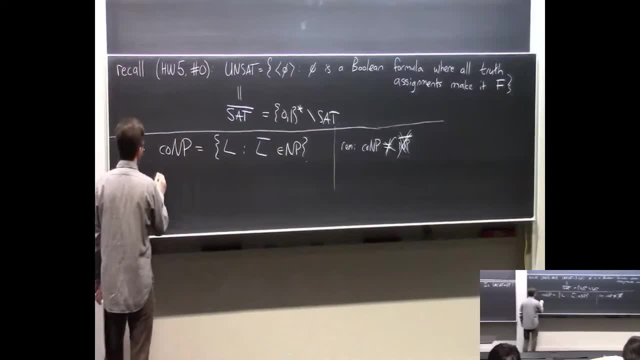 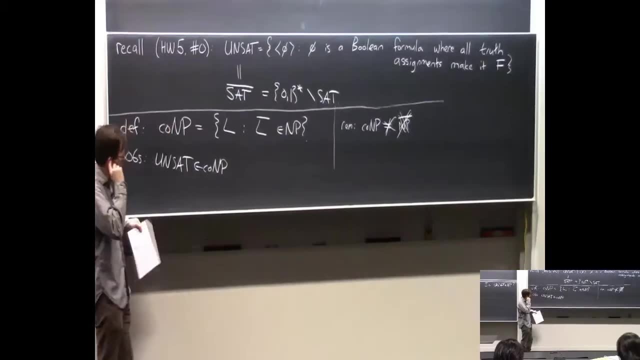 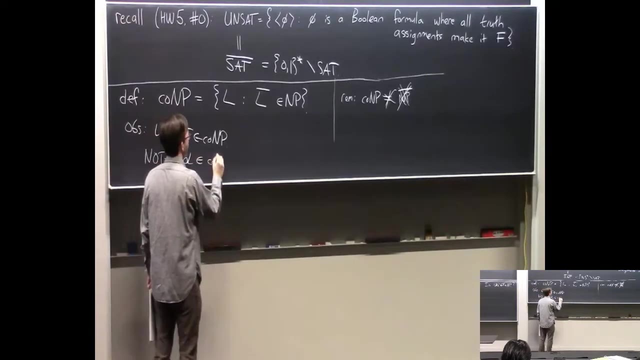 I mean, it's basically cooked up this way. so I mean the unsat problem is in coNP, okay, and also, for example, like the- I don't know, like the not three colorable problem is in coNP. this is like you're given a graph and you want to know: is it true that? 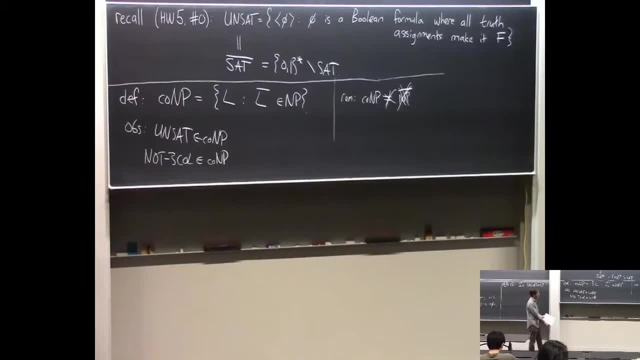 it cannot be legally colored with three colors or like the no Hamiltonian path problem is in coNP. so again, at first it looks like we're just making sort of trivial observations here, but let's roll with it. uh, okay, and the interesting question you know here is: 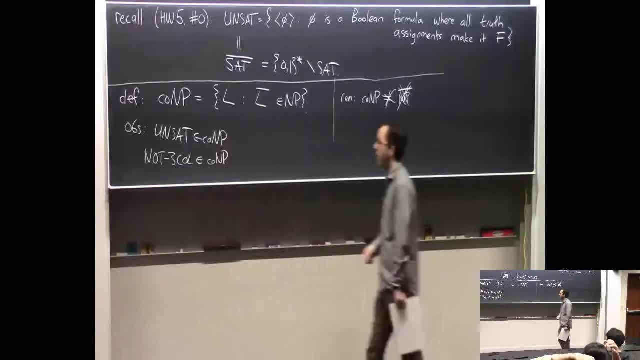 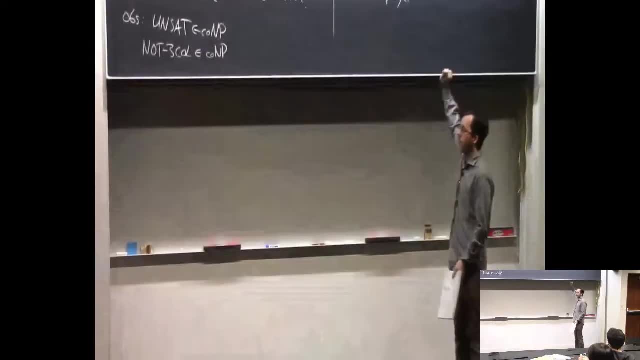 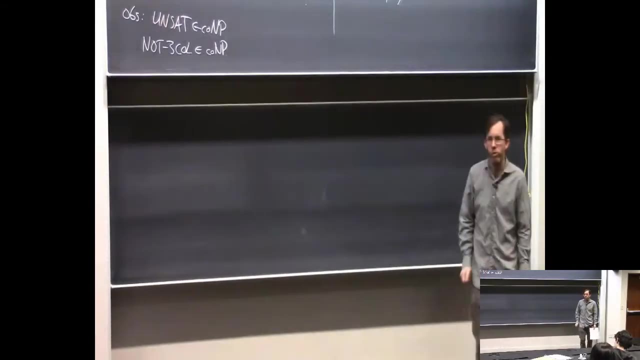 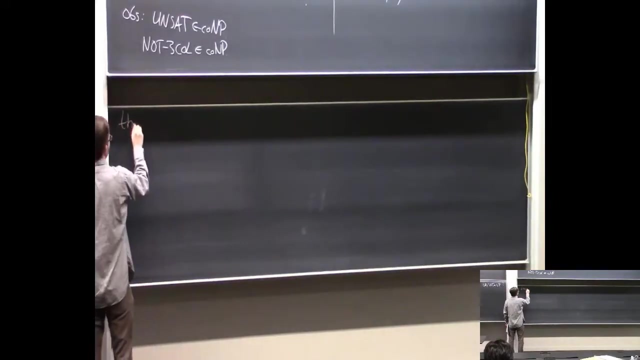 is this one? it's not. it's in coNP, but is it? is it in NP? uh, okay, let's make some, uh basic observations about this new complexity class we invented actually. are there any questions at this point? all right, um, okay, here's the first basic observation. 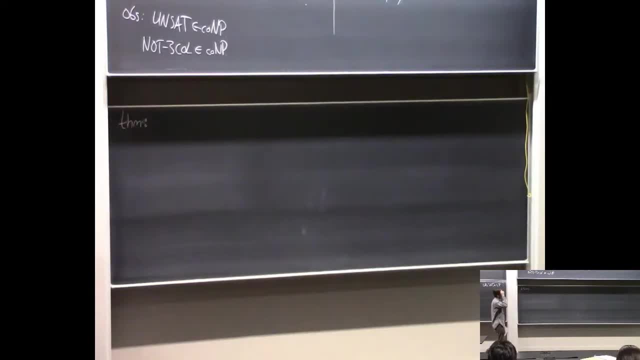 about the complexity of this problem. um, unsat, let's think about unsat a little bit more here. so, um, I claim that if sat is in P- which we don't really believe, but it could be true- then unsat is also in P. uh, can somebody say the proof of this? 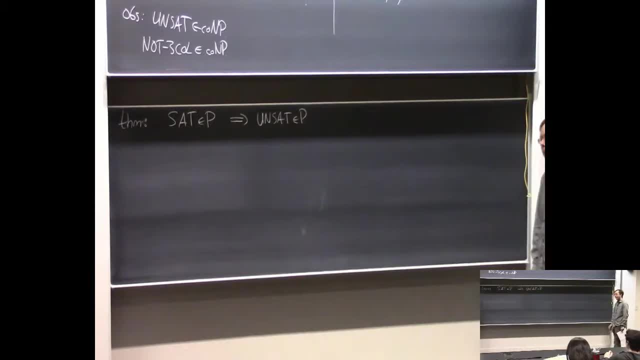 yeah, if sat is in P, then we know there's a polynomial time algorithm that can solve unsatisfiable and just reverse the. that's right, everybody get that. so I mean, let me not write it. but if, uh, sat is in P, that means there's a polynomial time algorithm. 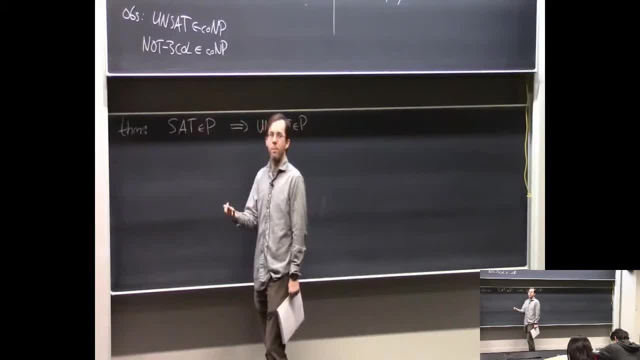 like a normal one that, given a Boolean formula, accepts if it's satisfiable and rejects if it's unsatisfiable. so just take that and reverse the accept and reject states, if you want to even think of it as a Turing machine. so then you'd have a polynomial time. 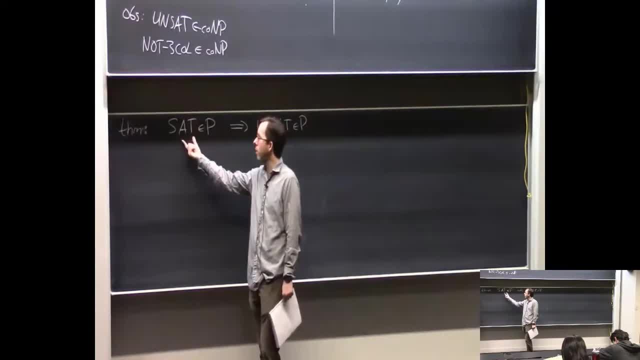 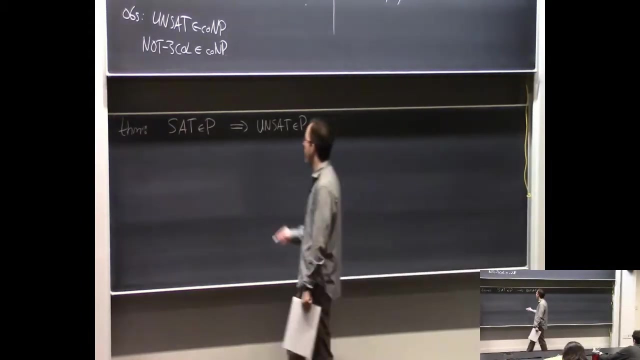 Turing machine that you give it a Boolean formula. it accepts if the formula is unsatisfiable and rejects if it's satisfiable, which means that it's deciding this language, unsat, is it okay? um, great, and what about? uh, this? this is also true if unsat is in P. 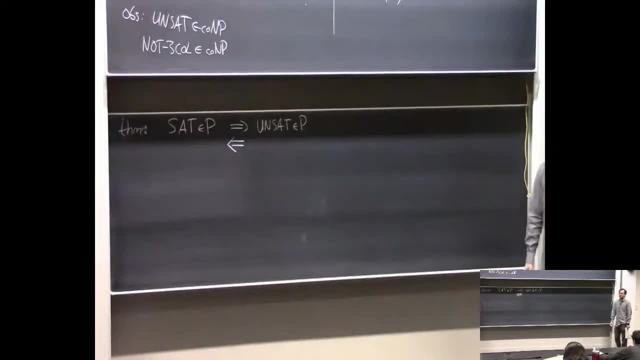 then sat is in P. well, it's the same proof, right? I mean, uh, yeah, if you have a, an algorithm that solves unsat, just take that algorithm and reverse its answer, and then the resulting algorithm solves sat in the same amount of time. so I mean, from some point of view, 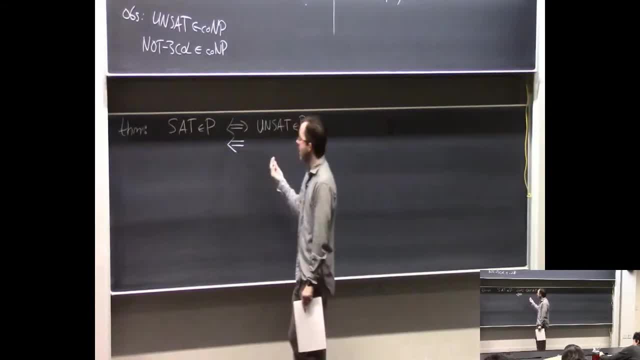 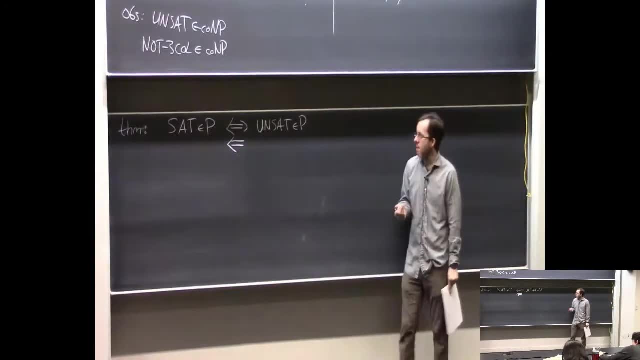 okay, based on seeing this, you might say: well, these two problems therefore kind of have the same complexity, right? I mean, you know, if you want to know whether one of them is solvable in polynomial time, then it's the same as asking whether one is solvable in polynomial time. 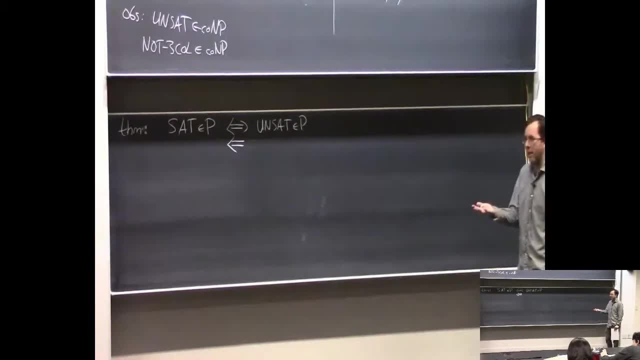 and usually you might say: well, what are we interested in in life? we're interested in, like, taking interesting languages and deciding. you know what is their computational complexity. so you may feel, therefore, that, like this theorem kind of tells you all you need to know, maybe, about the complexity of 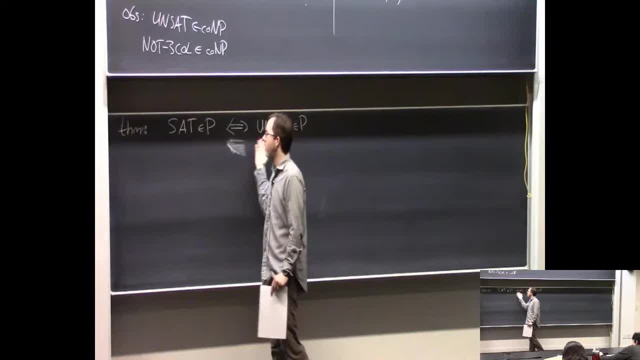 let's say unsat. I mean, you know it's in. it's the same question whether it's in P is whether sat is in P. it's the same question as whether P equals NP. so then why am I making a big fuss about it? I mean, if it kind of has. 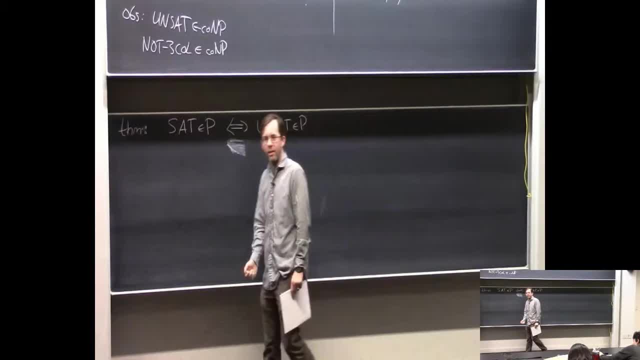 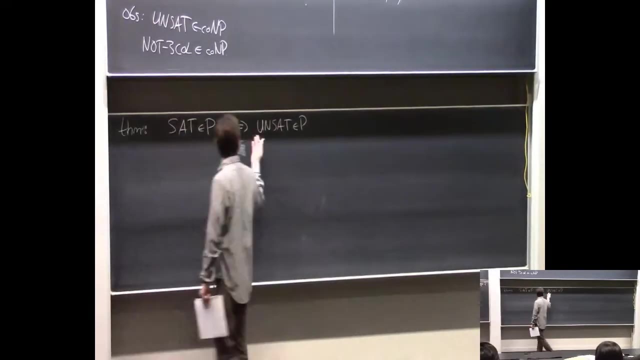 seemingly like sort of the same complexity as sat. what's the why are we studying it? and again we'll see. but basically I'll just return to this question. I mean, even though we know this fact that whether or not this language is in P is the same question as whether or not sat is in P. 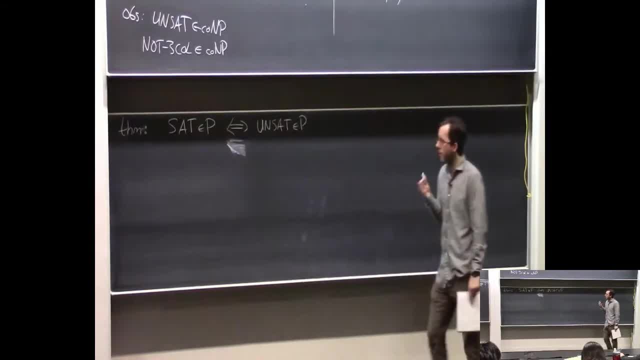 I wouldn't say that means we fully understand the complexity of the problem. I mean we really want to for every problem like really understand everything there is to know about it, and this is like one extremely interesting question. I'll state a more interesting version of this question a little bit later. 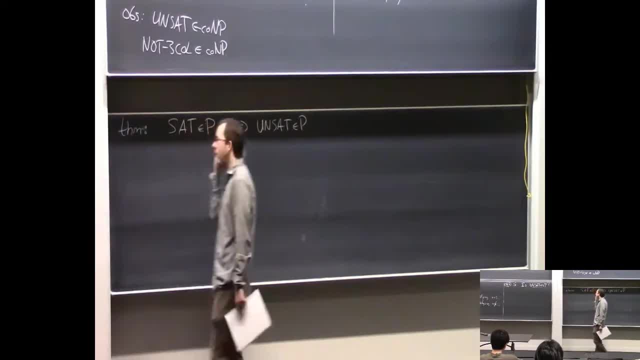 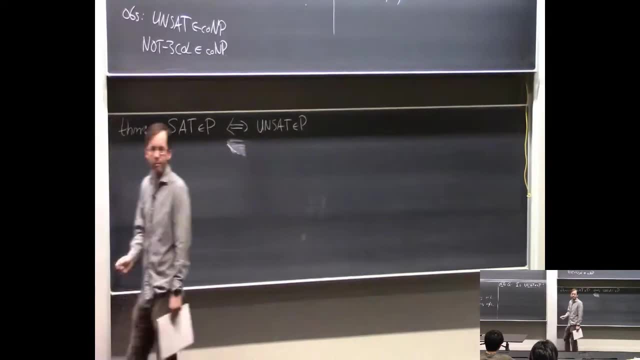 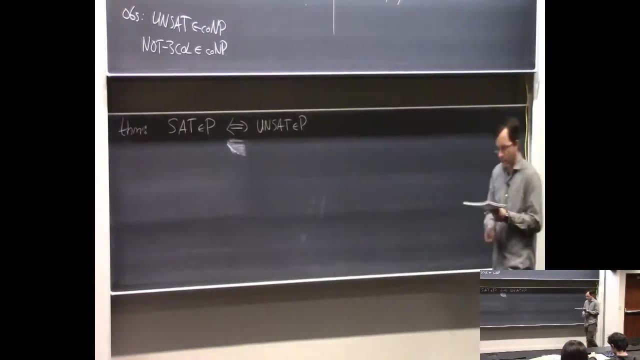 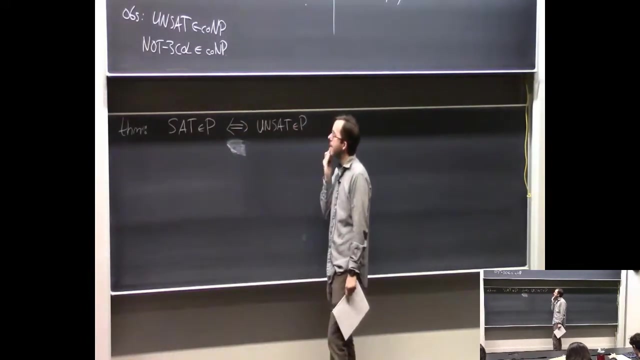 that we we don't know the answer to, and if we just kind of say, well, these are the same problem, sat and unsat, then it kind of takes away our ability to even ask this question. okay, all right. um, actually, while we're on this subject, this is the typical. 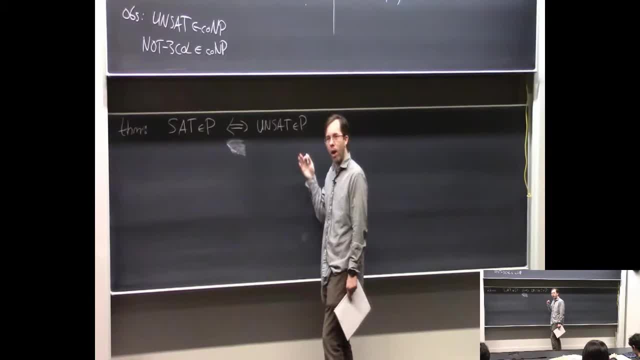 one typical reason why we try to show languages reduced to each other to try to derive conclusions about: like well, if one language is in P, then another language is in P. so I've tried to stress a couple times that's not the only reason we try to prove one language reduces to another. 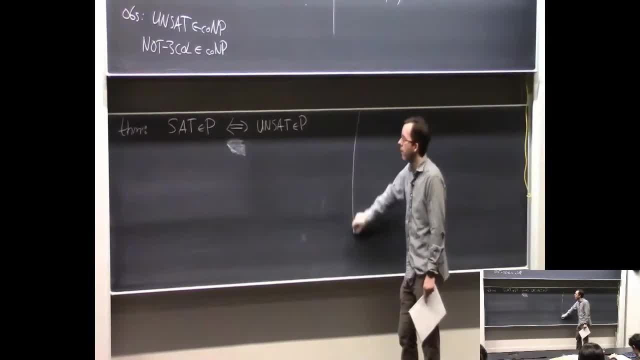 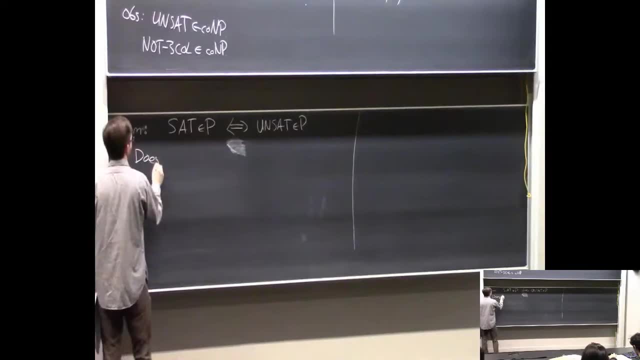 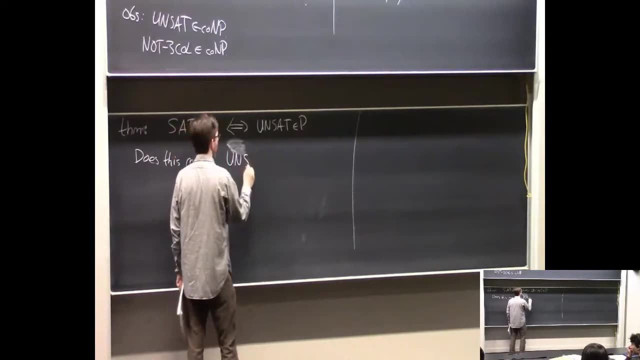 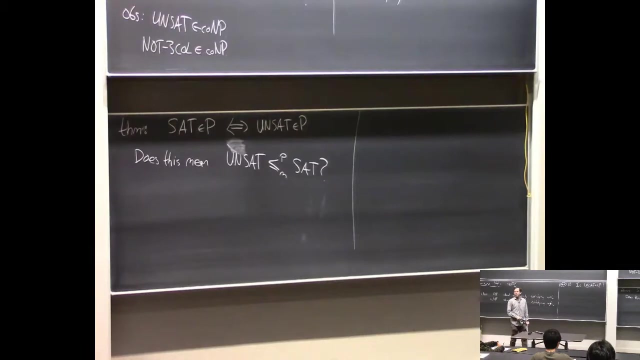 but like that's a common reason. so, for example, you know once you, you uh know this. you might ask yourself like, well, does this mean, let's say that, um, unsat reduces to sat, does it? Yeah, Well, that would mean that unsat was in P. 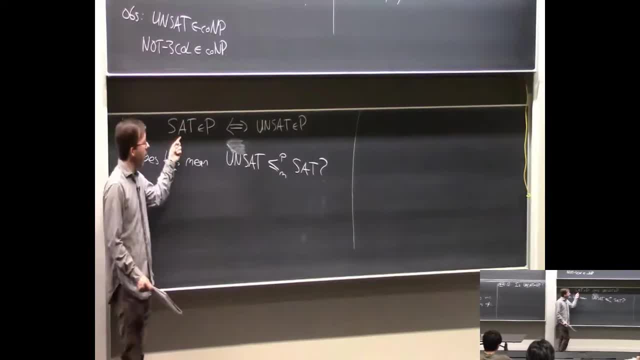 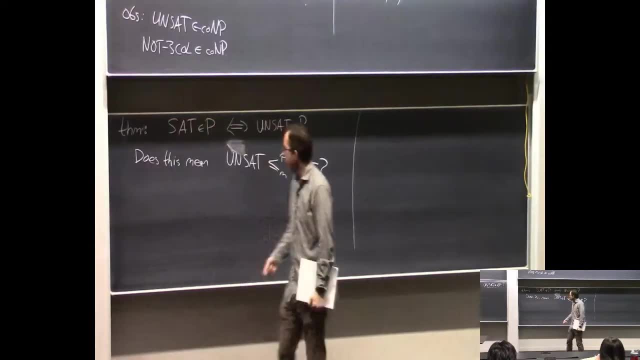 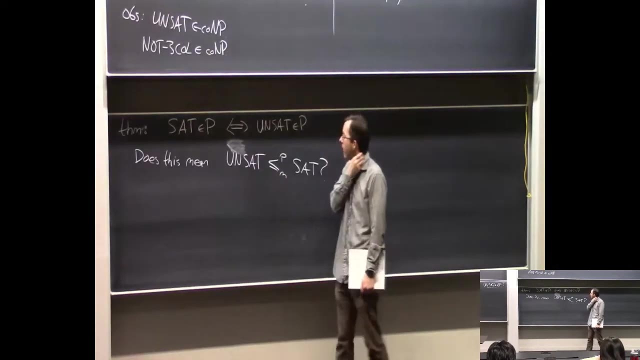 That's right. yeah, I mean. uh, this is not, like you know. this implies this is not the definition of this. so this does not obviously imply this and, in fact, remember, one reason why we care about reductions and, in particular, this particular kind of reduction, mapping reductions, is we have a theorem that says: 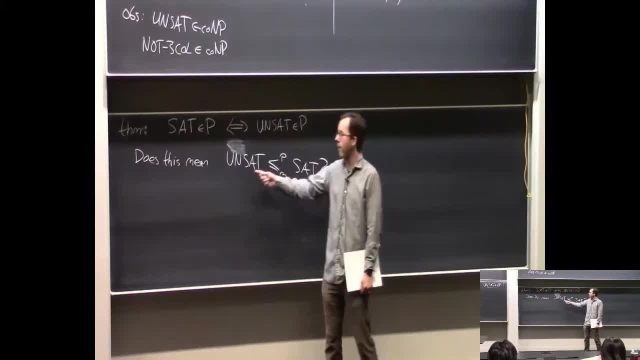 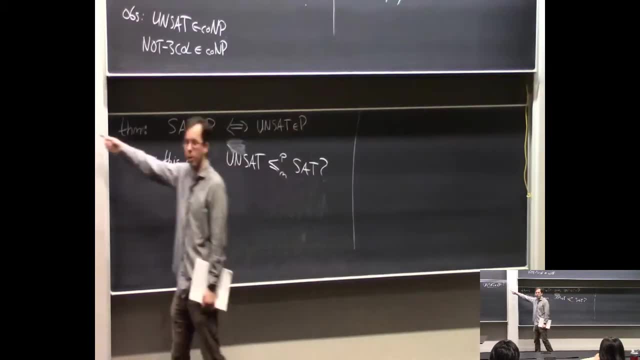 when this happens, if you know this side is in NP, it follows that this side is in NP. so if this were true, we know sat is in NP. we would conclude that unsat is in NP. which is this motivating question that we have for ourselves, that we actually don't know the answer to. 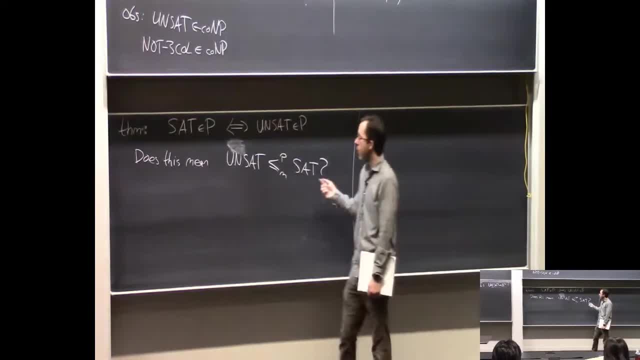 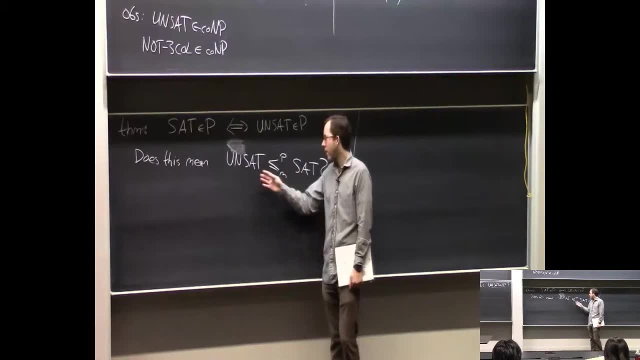 Okay, and again, just to emphasize this one more time, it is true that for a different notion of reduction, I think, one that you even talk about in 251, when you're proving like undecidability and stuff, there is a sense in which this language reduces to this one. 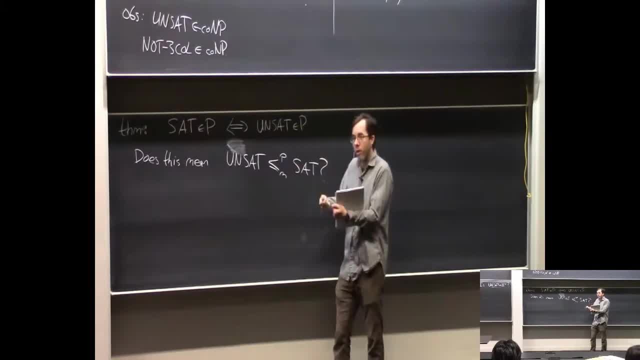 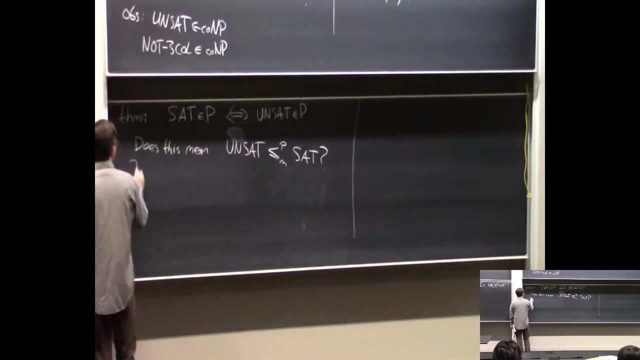 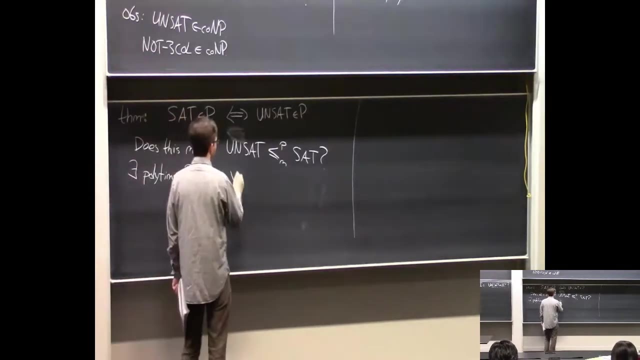 if you have an algorithm for this one, you run it and reverse the outcome. you get an algorithm for this one, but remember, let's literally write down what this means, right? this means there exists a polynomial time r such that x is in unsat if, and only if. 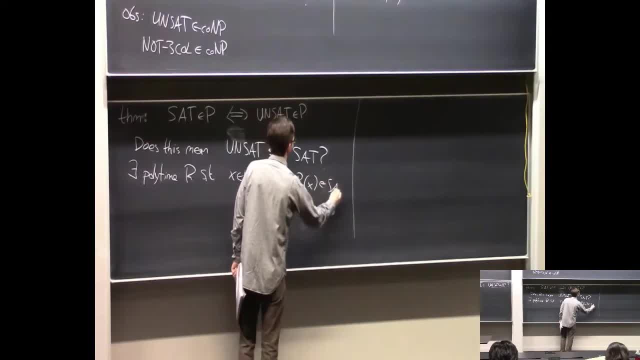 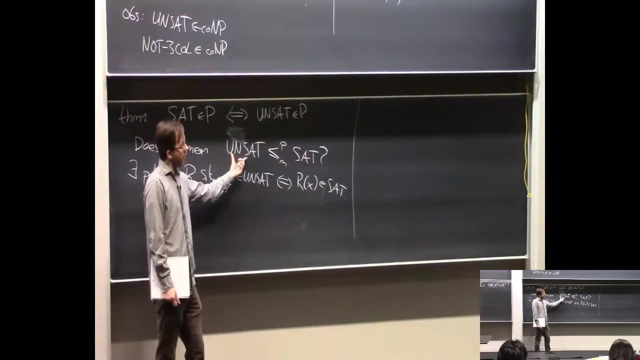 r of x is in sat. okay, so like the algorithm is not allowed to like, let's say, try to decide if x is in sat and then reverse the answer, the only thing our notion of reduction allows you to do is take a string over here where you want to know if it's in this language. 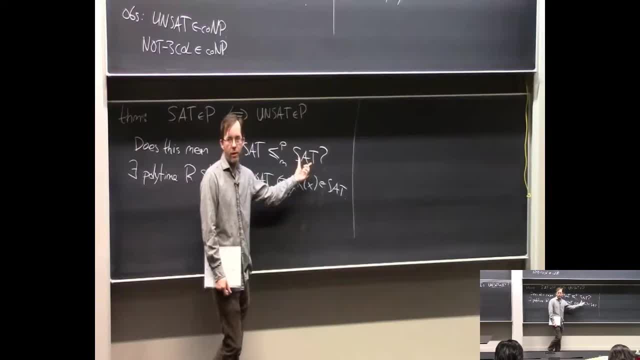 and try to convert it to a new string which has the same answer regarding whether it's in this language, and it's not clear how to do that. right, let's say I give you a Boolean formula and you want to know if it's unsatisfiable. 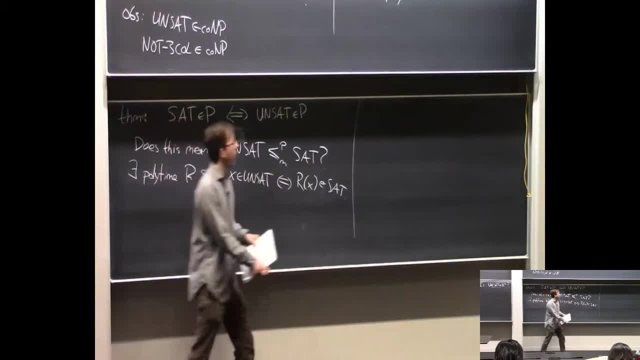 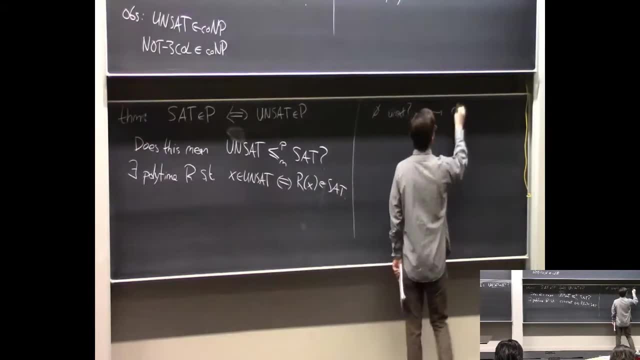 how could you convert it into one, a different one? you know you want to know, is this unsat? so you're like, well, can I convert it into a different one? where, like, the answer to whether or not this one is satisfiable is the same as the answer to whether this one is unsatisfiable? 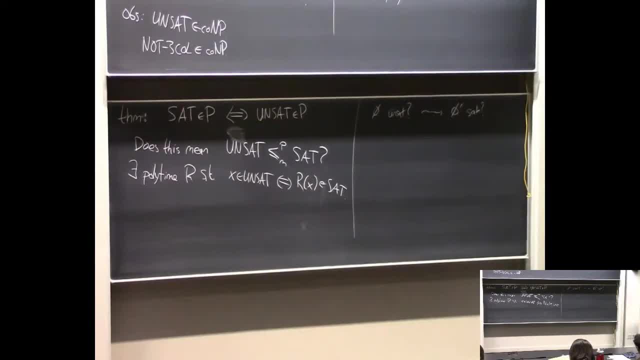 hmm, it's not clear. I mean your first instinct. my first instinct would be like: oh, what about? I'll just make phi prime to be the negation of phi? that's certainly a polynomial time reduction, but unfortunately it doesn't work. so what is a? what is a particular phi for which this reduction fails? 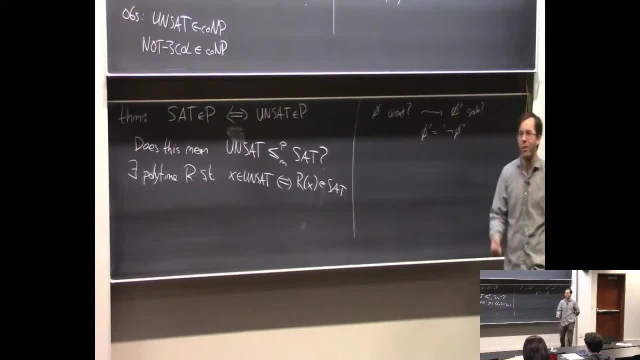 practically any answer will be correct. so just like throw an answer out there: yeah, x or y, sure x or y. so like, if phi is x or y, is that unsatisfiable? no, it's not unsatisfiable, it's quite satisfiable in fact. so this is: 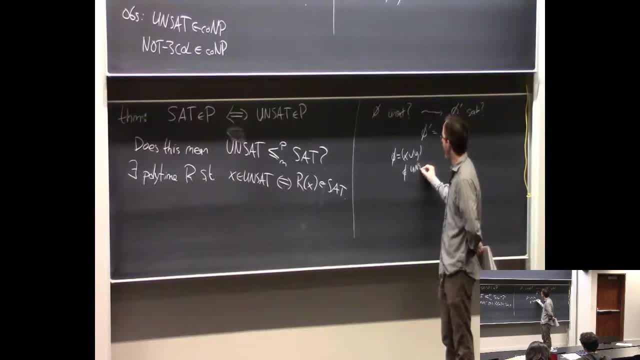 not in unsat, and then we can look at: not phi, which is negation of x or y. is that satisfiable? yes, you can make them both false and it'll be satisfied. so it is insat. okay. so this reduction is broken. we got a different answer here and here. 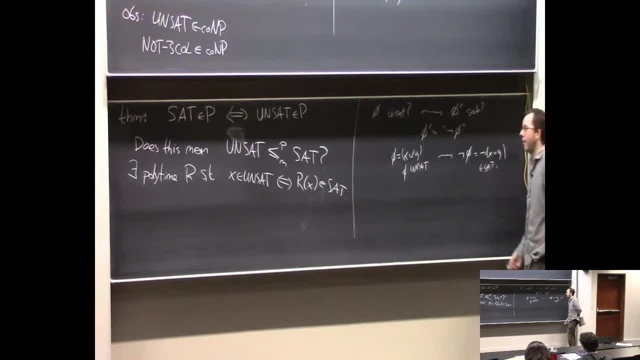 so like this doesn't work and we don't know if anything works and we kind of believe that nothing works. by the way, here's like an interesting okay, any question about that? yeah, do we know? that's, I'll talk about that in a little bit. 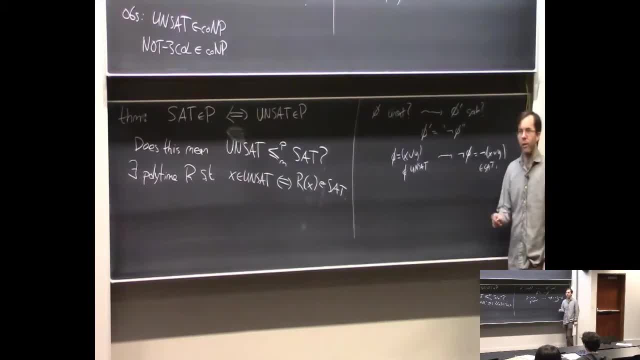 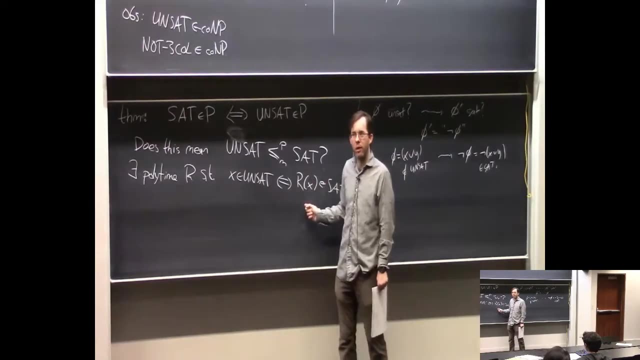 yeah, just hold on to that question. here's an interesting fact actually, whether or not this, okay, I just this is literally the definition of this right and you know, if you have like p, if and only if, q, that's the same as negation of p, if and only if. negation of q. 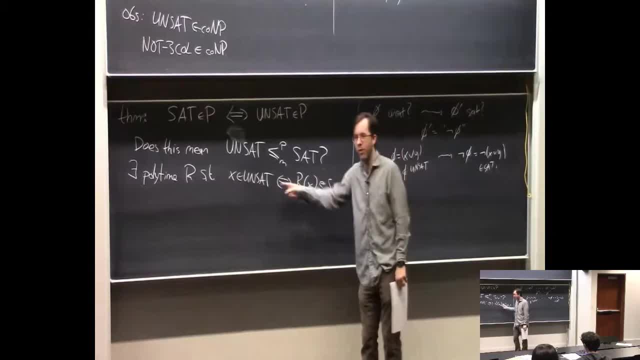 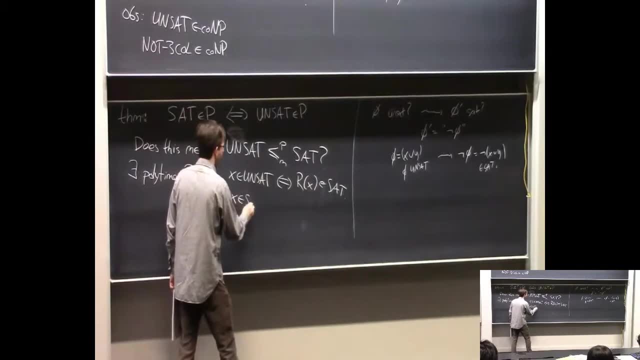 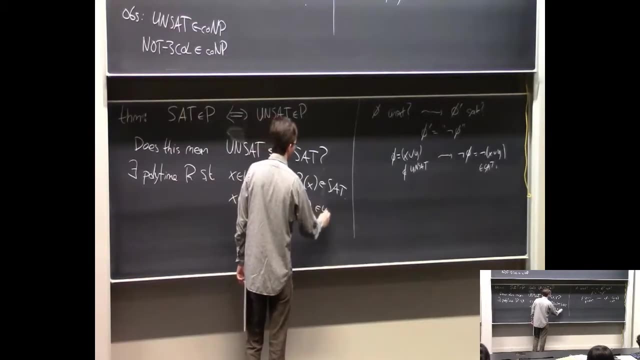 right, like that's some 151 stuff. so let's take the negation of both sides to get an equivalent statement. what is the negation of x in unsat? it's x insat. and what's the negation of rx insat? it's rx in unsat. 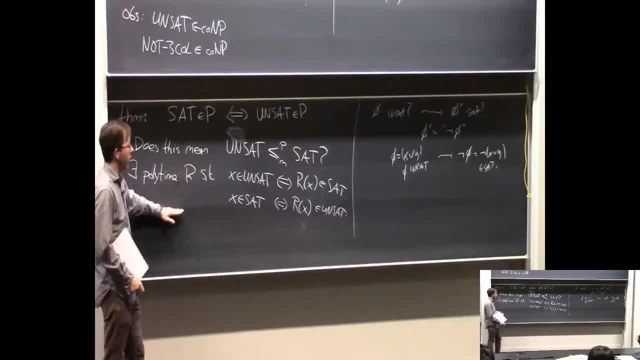 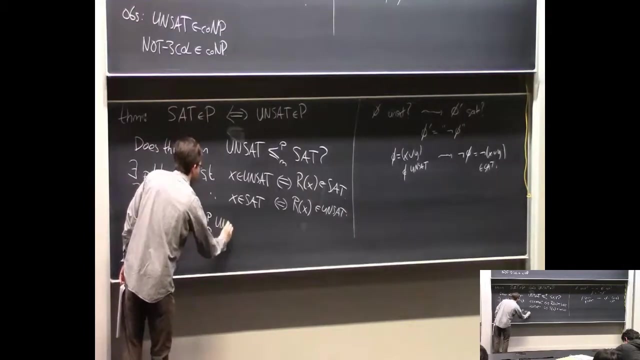 so this statement, the definition is this first line, which is equivalent to. I mean, it's the same as this line and this line is saying that. what does this line say? something similar to this, but a little different. yeah right, this is the definition of sat: reduces to unsat. 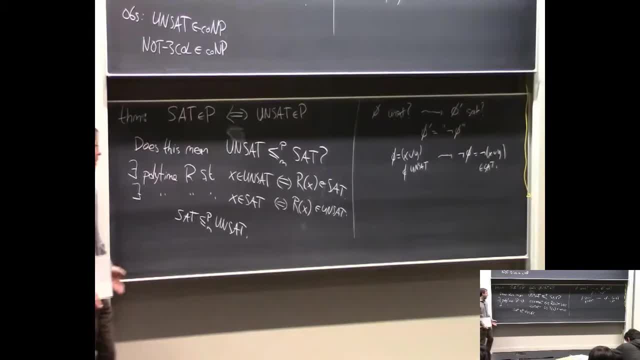 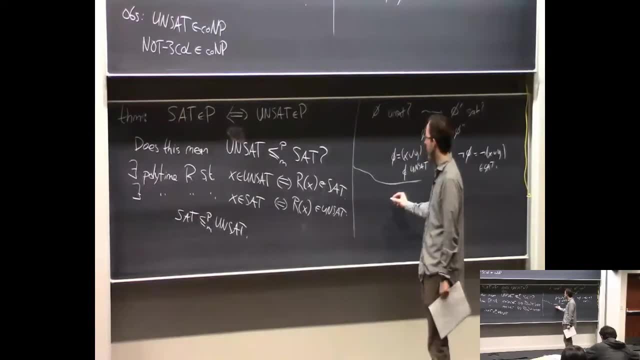 so that's a little magic trick. I mean, just write down the definition. this is true if, and only if, this is true. actually, that's just I could have asked you this like on you know homework, three or something: a reduces to b, if, and only if, the complement of a reduces. 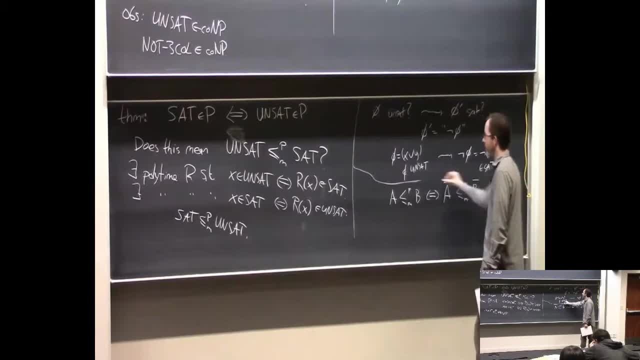 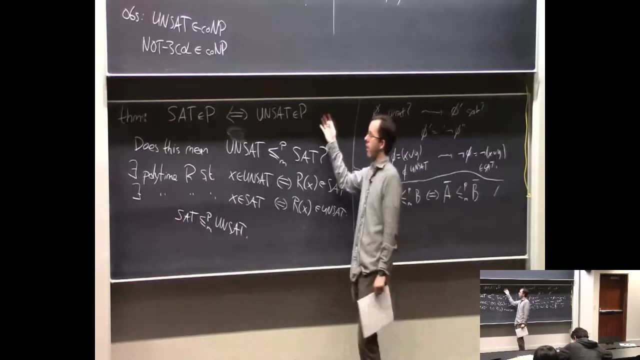 to the complement of b. that's a funny fact, but it's true. just remember this for five minutes from now, okay, so it is true that in some sense, the question of whether or not they're in p is the same, but you shouldn't. and it's true that their definition. 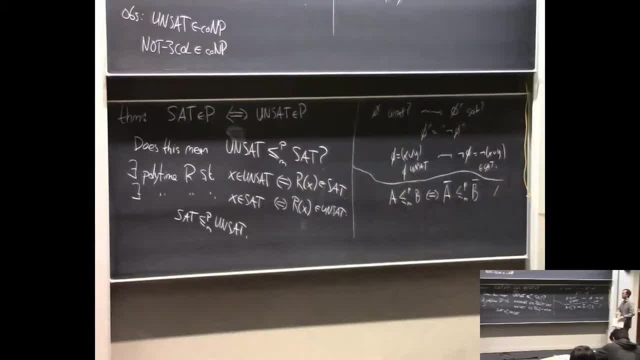 looks practically the same, but it's very helpful to view these as different problems. okay, so I keep asserting that fact to you and we'll get to the explanation why. but yeah, wait. so just to be sure. the problem with the production is that, like if you have x in unsat. 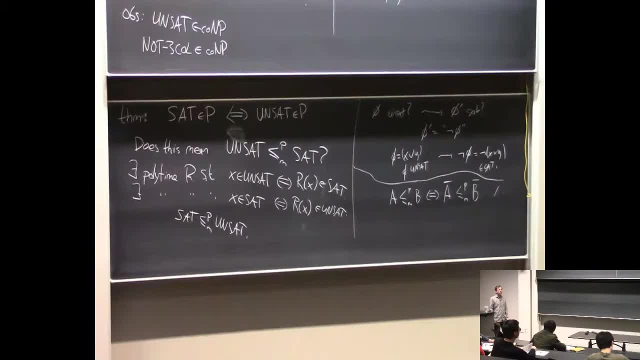 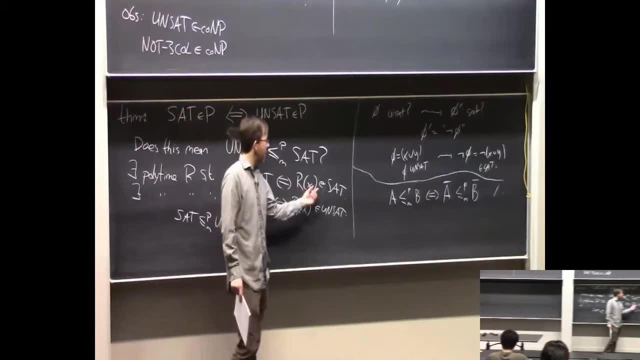 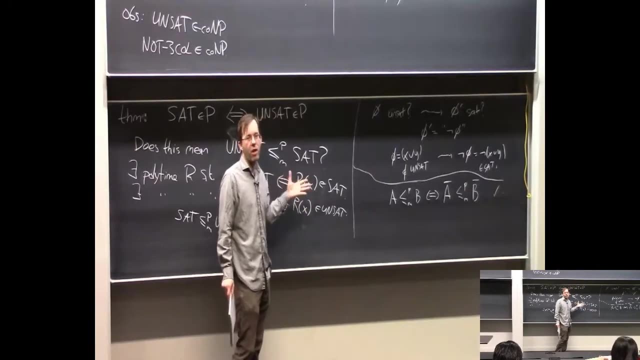 you're actually taking r of x, not insat, which isn't allowed. well, that's right. in some sense you kind of wish this said: r of x, not insat. if that were true, then r could just r, of x could just be x. I mean it could just do nothing. 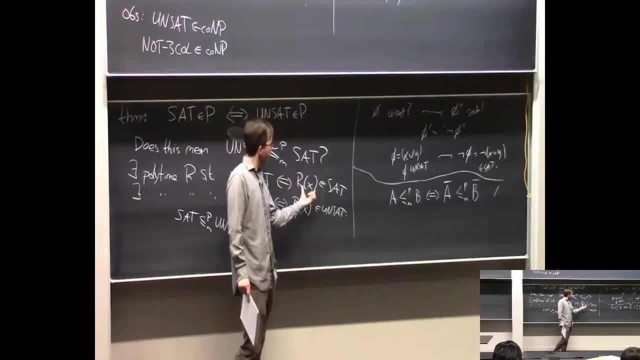 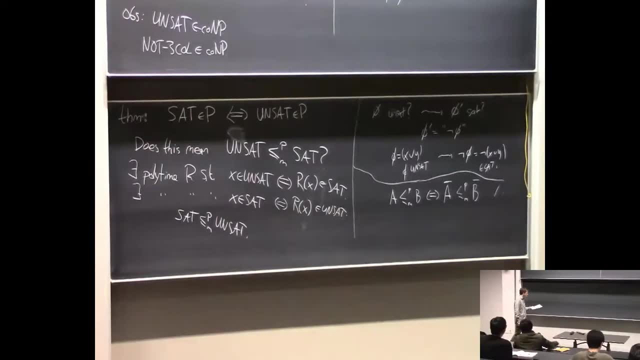 but like somehow you're not allowed to kind of reverse the condition at the end in the definition of mapping reduction. okay, so before we get into like why it's interesting, some more. I nevertheless want to play around with some definitions. it'll look like just playing around. 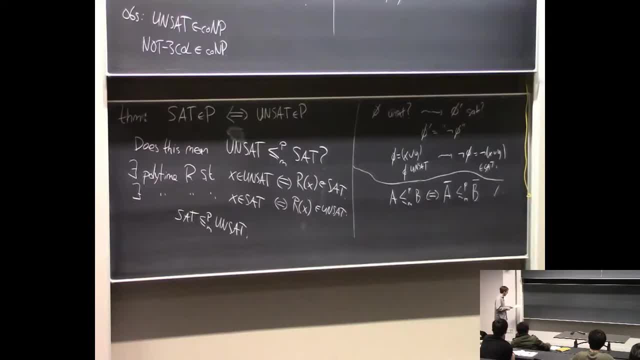 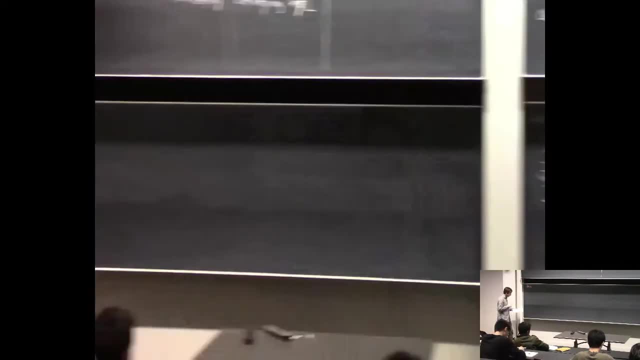 but it's good practice in complexity theory to to do these things and we'll learn a little bit more about how it works. so I just want to make like a series of simple theorem statements. first one I want to say is: actually, you proved this exact statement on the homework. 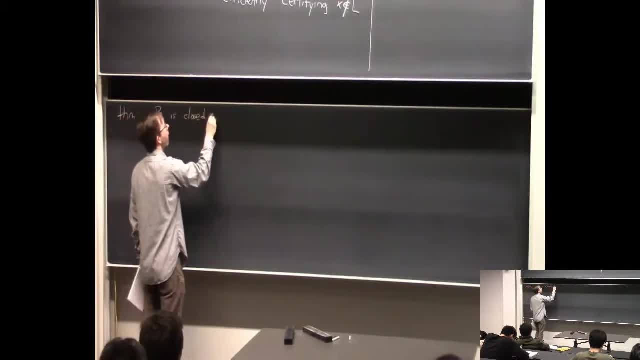 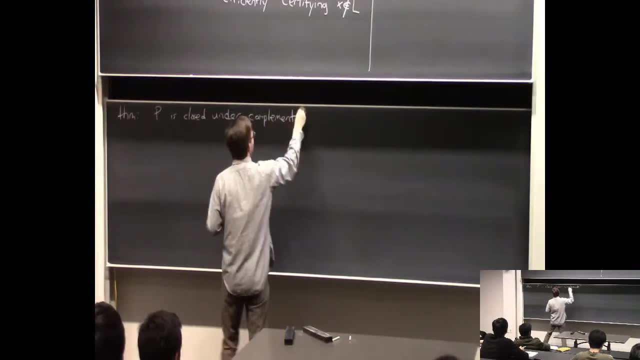 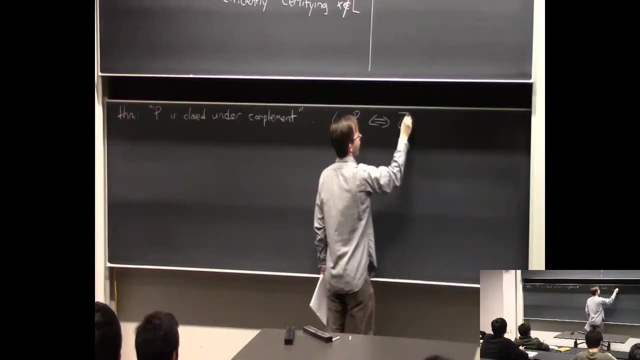 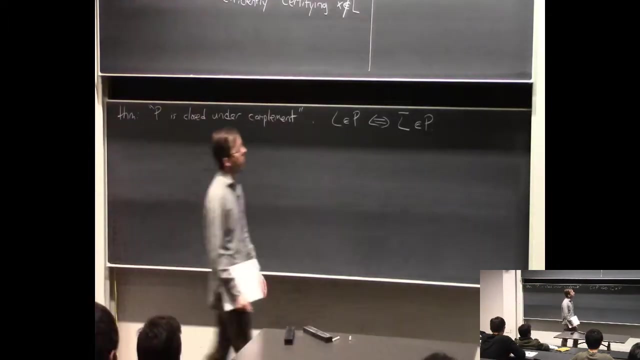 which is that p is closed under a complement. it was literally problem 3a on homework 2. what it means is: l is in p if, and only if, l bar is in p, the complement of l. okay, and let me not write the proof, because you already wrote the proof, but 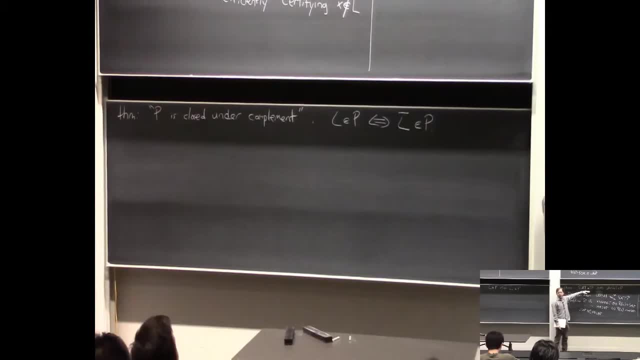 it's literally also the same as this fact. I mean, if you have an algorithm, a normal algorithm, a polynomial time algorithm solving l, just reverse it, except in reject states, and you get a polynomial time algorithm that solves complement of l, and some people write this as a 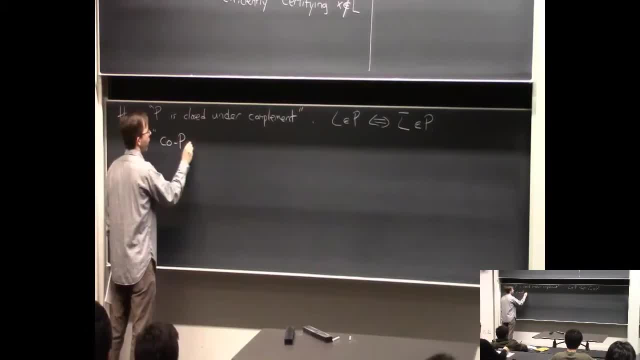 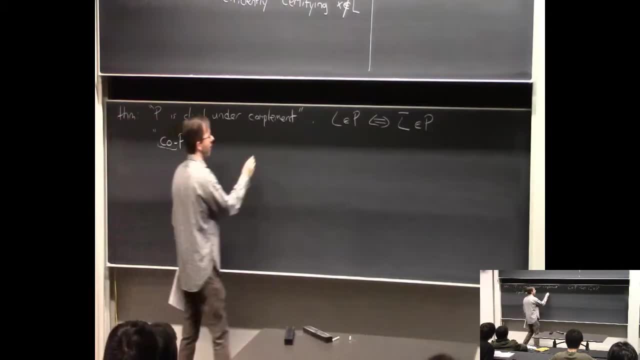 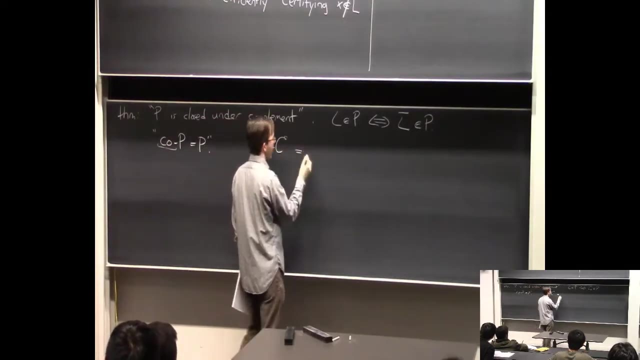 or could write this as: co p equals p. so actually in general this doesn't only show up in co and p. so there's like a little. if you want to be like a cool complexity theorist: co c- if c is any complexity class, this means all the languages l. 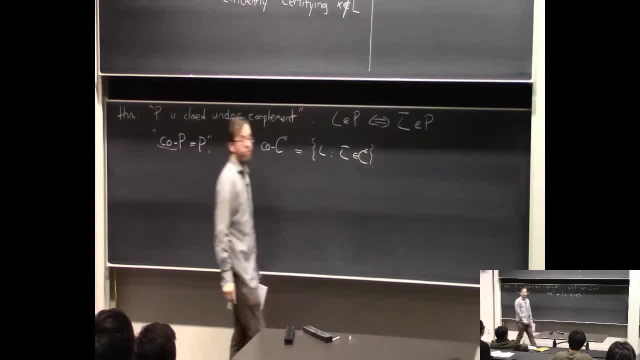 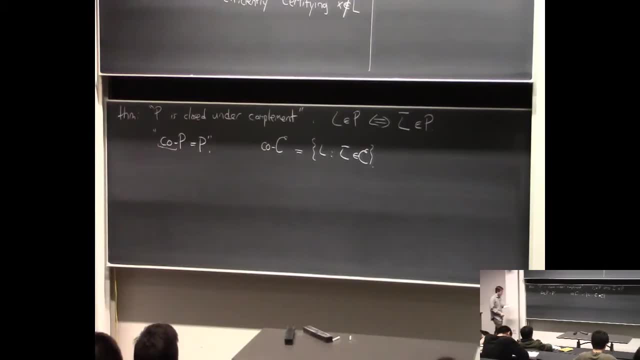 such that the complement of l is in c. okay, but you never hear people talk about co p because it's just the same as p. but for example, we also have that like co exp equals exp. it just says if you can solve a problem in exponential time. 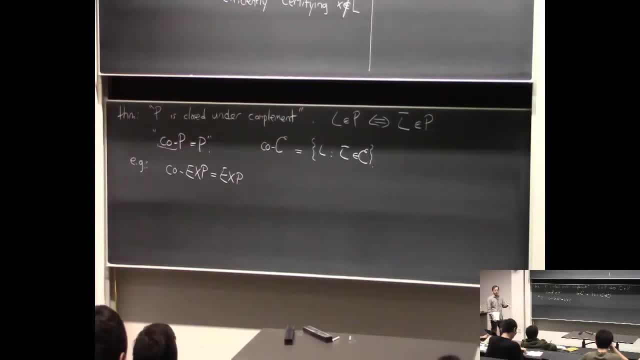 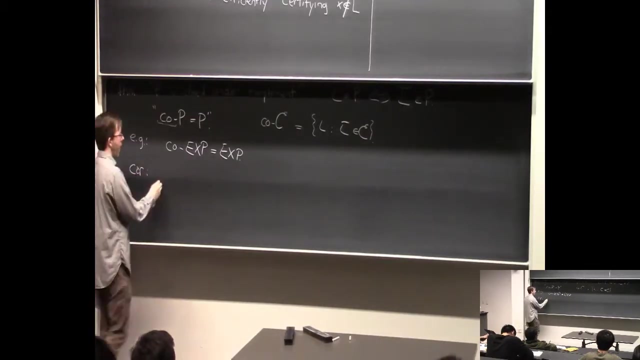 you can also solve, like the negation of that problem, just reversing yes or no, also in exponential time, because it's the same proof. you just take the algorithm and switch its accept and reject states, okay, so let's make a corollary of this. a corollary of this is that 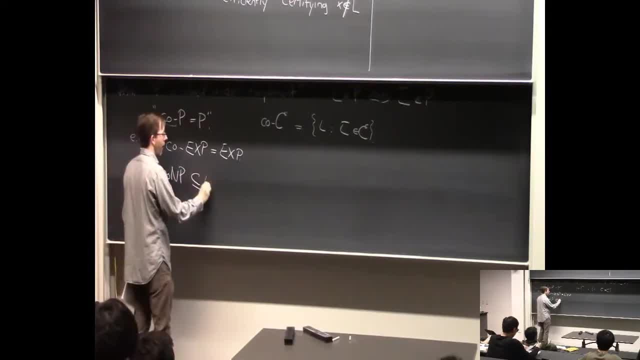 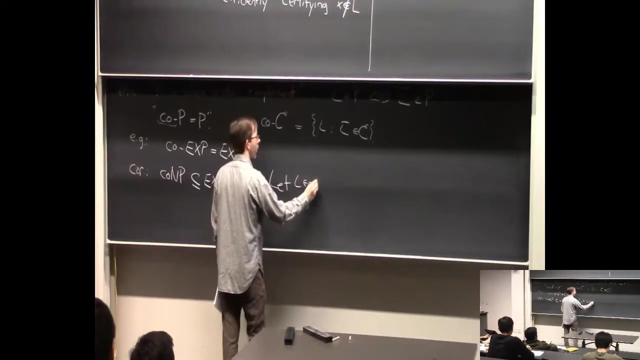 co n p is a subset of x. why is this true? well, let's prove it. it's one subset of languages contained in the other, so I'll take a language in here and show that it's in here. so let l be in co n p. well, the definition of that is basically that l bar is in n p. 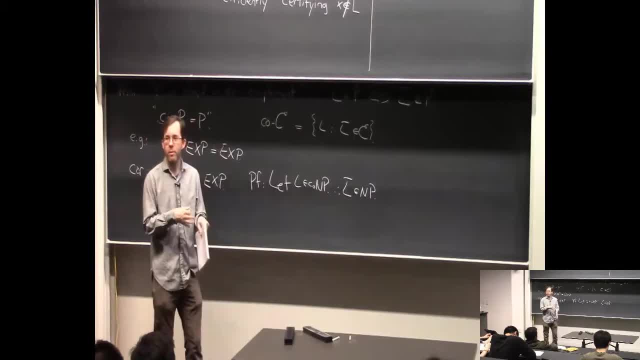 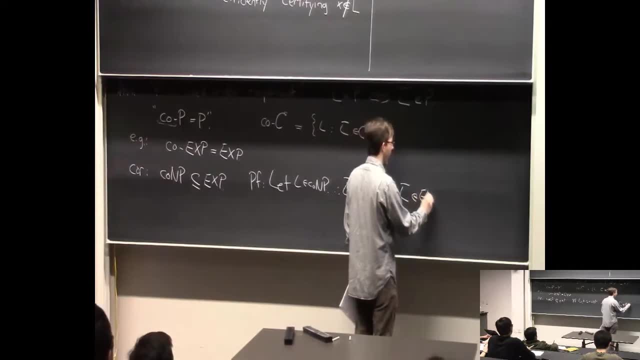 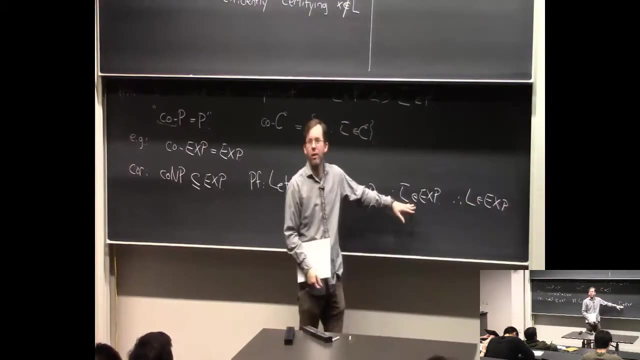 and we know that n p is a subset of x. maybe that was also a homework problem. so therefore l bar is in x, okay, and therefore l is in x. I mean, if I wanted, I could say this means l is in co x. but anyway, if you can solve, yes or no is a string in l in exponential time. 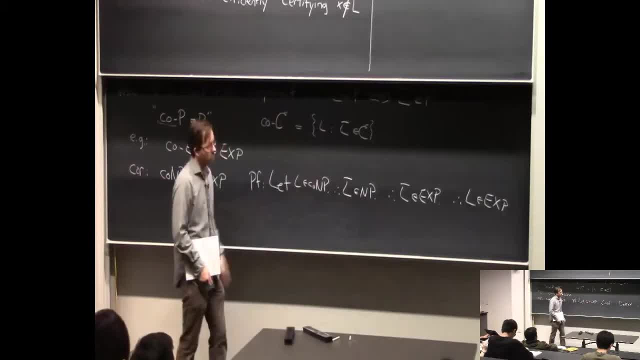 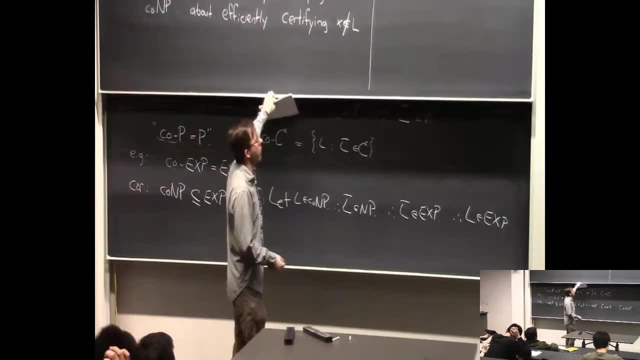 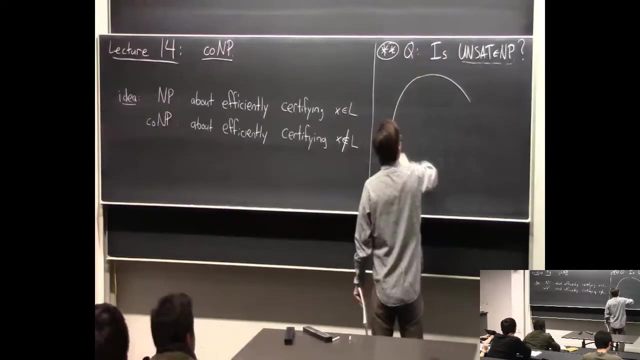 then you can solve no or yes. is the string in exponential time? is that okay? so I bring this up so that I can start drawing a little picture of some complexity classes we know. so you know it's always a little weird with these classes like n? p and co n p. 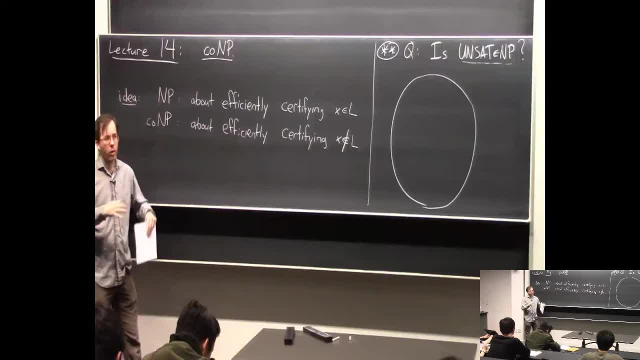 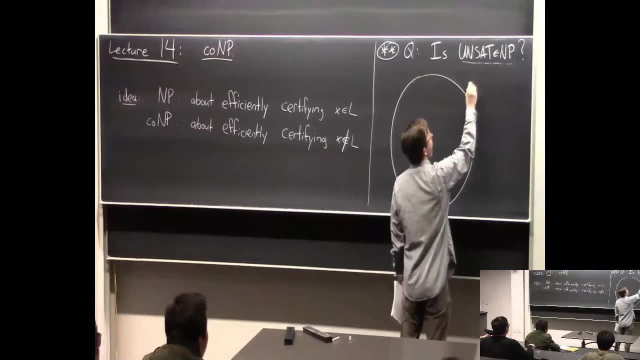 that involve nondeterminism or verifiers or whatever like you kind of want to get a handle on them in terms of just like normal computation. so exp is a good class to put everything inside of any language that's in these classes: n, p, co, n p, etc. 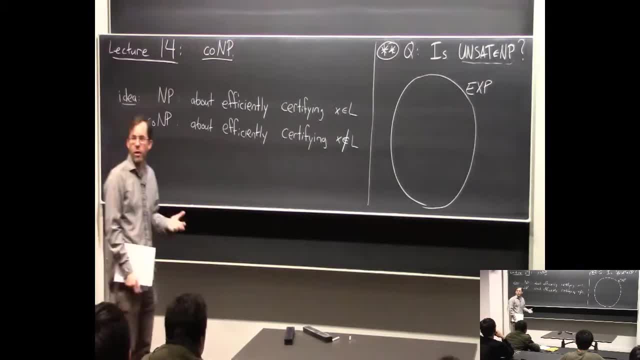 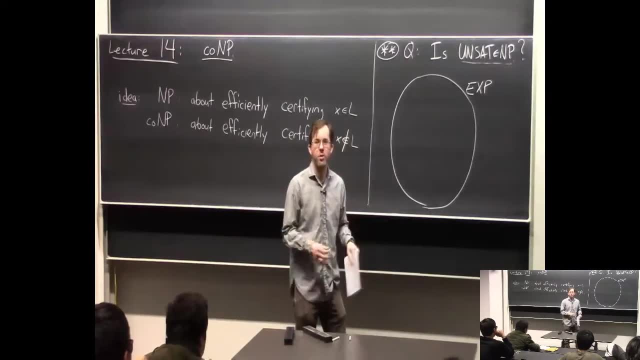 at least you can solve it in exponential time on a normal computer. so let's put n p and co n p in here, and so far we don't know anything about the relationship between them. so we have to draw the most general venn diagram, which is like this: 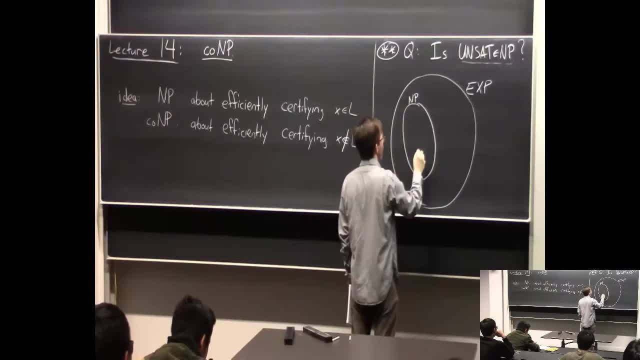 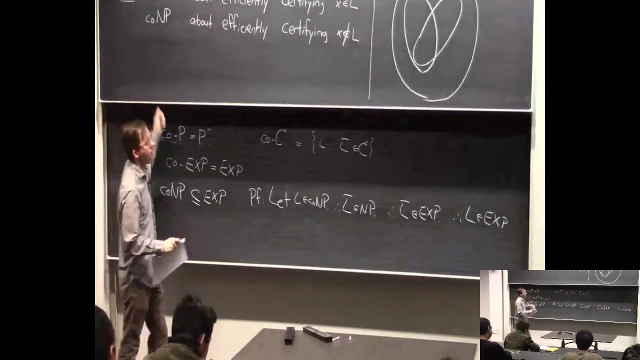 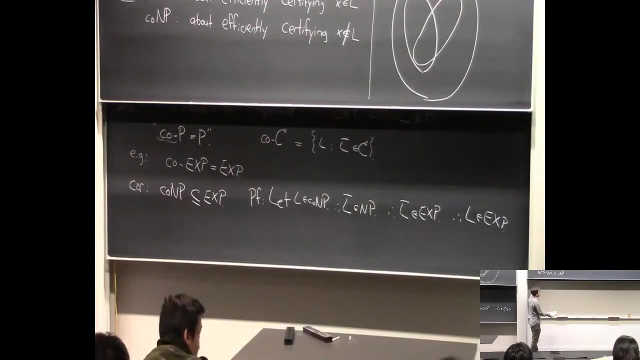 maybe this is n p, and then maybe there's some overlap with co n p, and then, well, we'll put something in the middle here in a second. here's another little theorem that'll help us fill out this diagram. p is a subset of co n p. 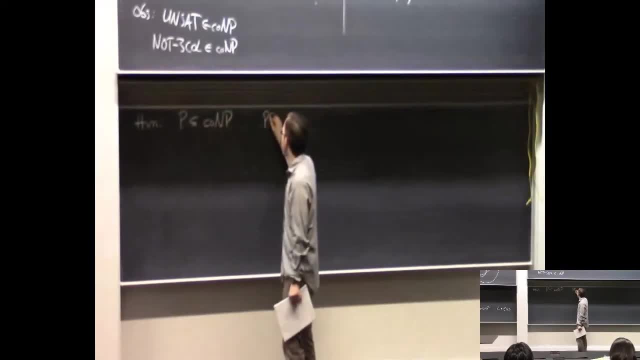 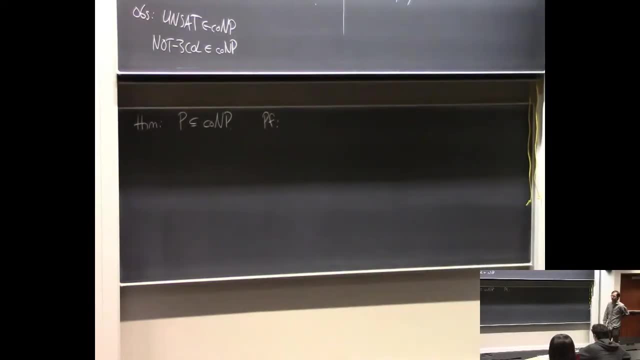 so somebody wanna say why this is true? we can do it straight from the definitions, plus the fact that you well combine everything that's written on the board. so if you know a language is imp, then it's confluence, and then that means the complement is in NP. 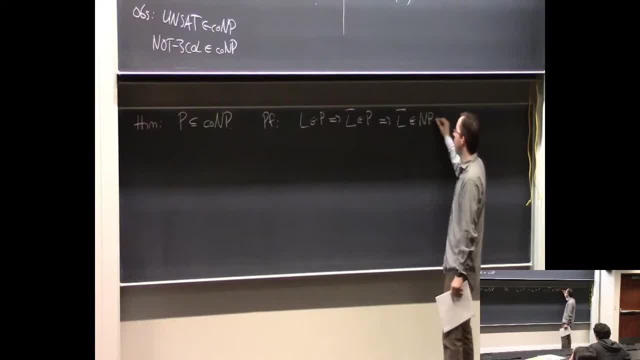 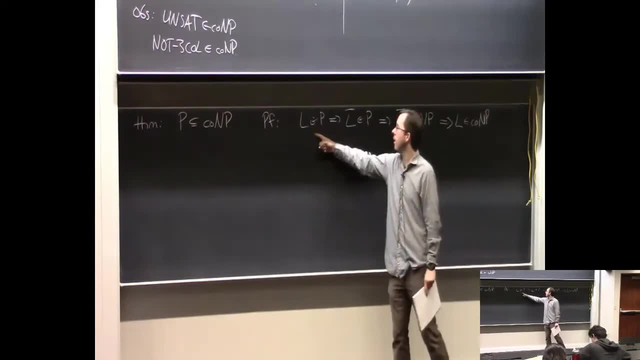 Right, because we know that P is a subset of NP. Right, this last step is okay. so this is our assumption. This is because P is closed under complement. This is because we know P is a subset of NP And this is the definition of co-NP. 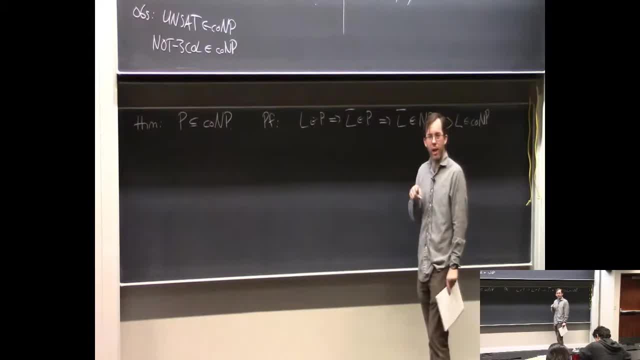 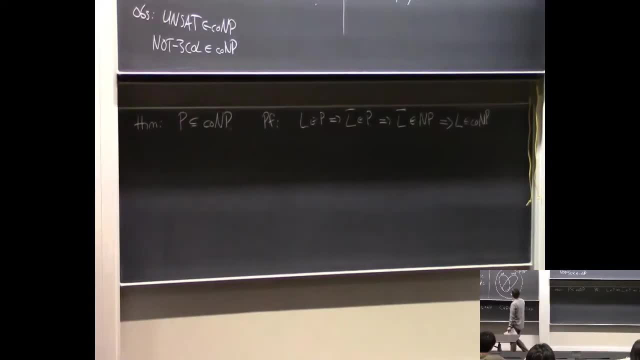 Yeah, you could sort of say, like: take the fact P is a subset of NP and co-both sides the way you could say it. Good, so we know that P is hiding in both NP and co-NP. So this is a picture of the world. 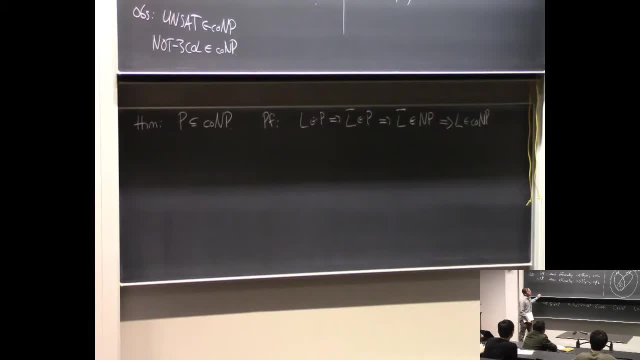 with four complex classes that we know. Now, the way I've drawn it is kind of suggestive that, like all of these you know, white spaces are possible. So we talked about, for example, whether well, in Ladner's theorem we talked about whether 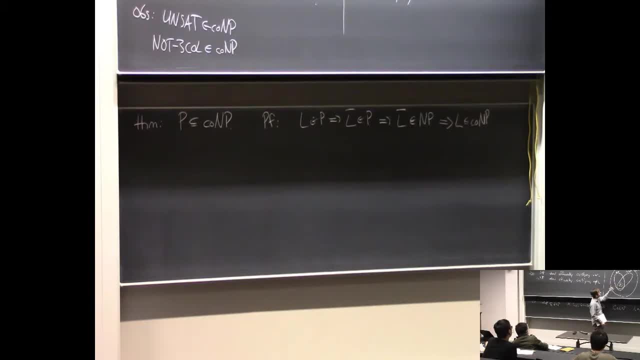 yeah, P is different from co-NP, I guess. or sorry, NP complete, I guess I should just say right. it could be that, like P and NP are the same, So this diagram would be misleading. We don't really believe that, but that's one possibility. 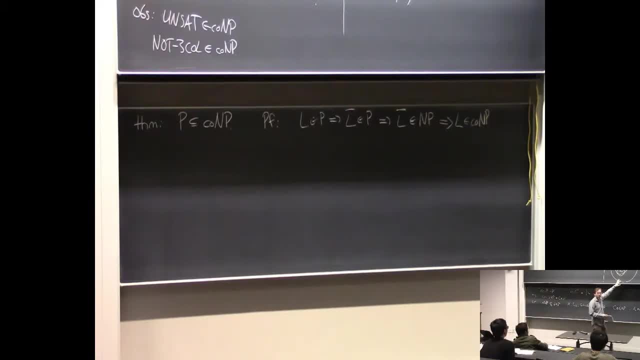 In general, it's believed that everywhere there's like white space. here it's possible that there are really languages there. So let me actually talk just about that. like what if P equals NP? What does that mean for this picture? 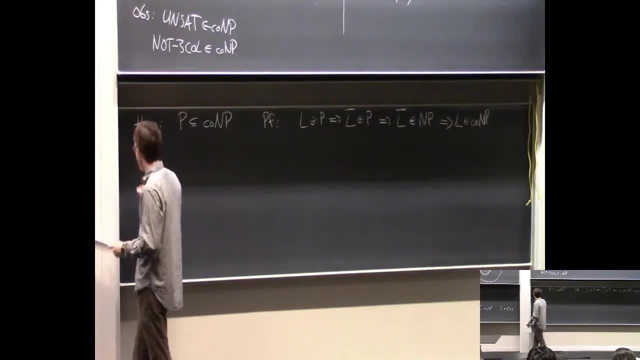 Good, So I claim that if P is the same as NP, then also P is the same as co-NP, And also let me say that NP equals co-NP. Well, actually I just said two different things there, so let me say the first one out loud. 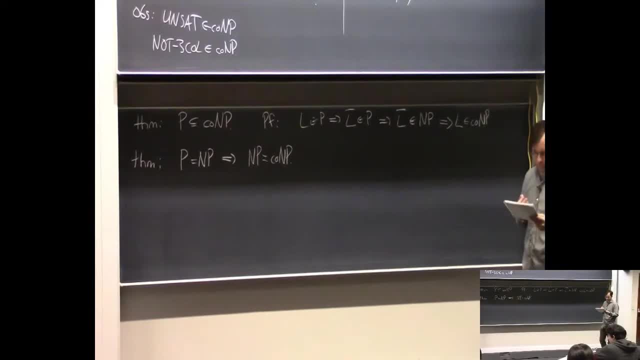 If P is the same as co-NP, then also P is the same as co-NP. So if P equals NP- am I going to say that later? Okay, if P equals NP, let me just write that- then P also equals co-NP. 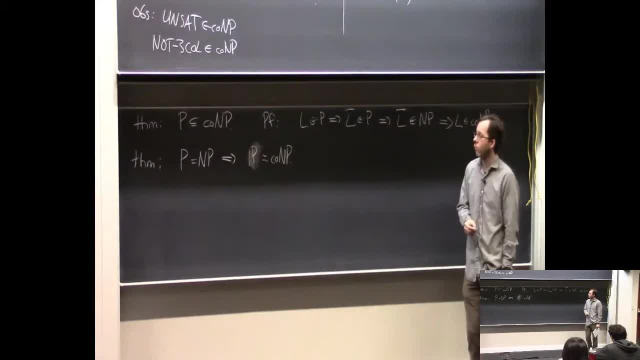 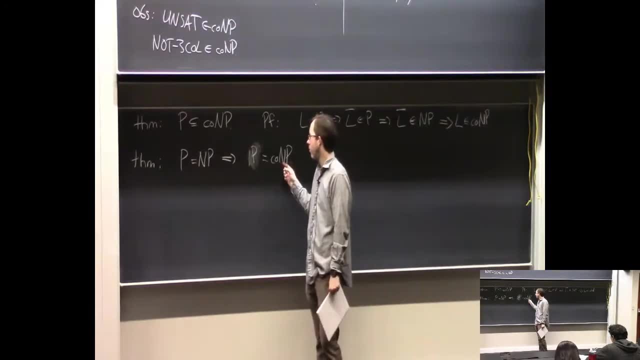 Why? Well, if you have a language in co-NP, its complement is in NP. So if P equals NP, that means the complement of the language is in P. That means the language is in P because P is closed under complement. 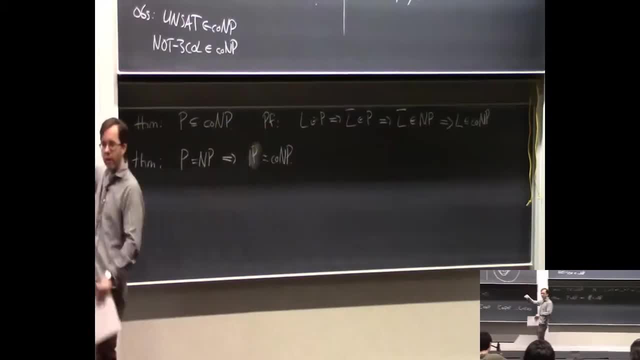 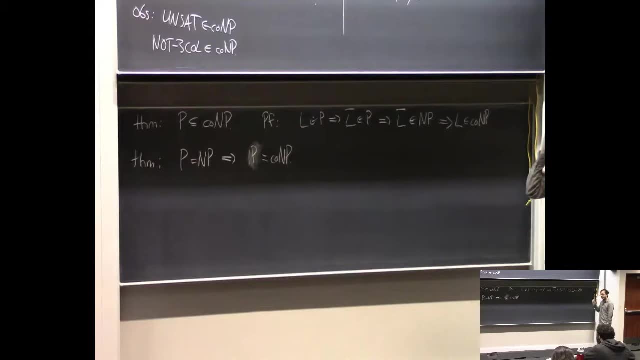 So if P happens to equal NP, then all these three classes on the inside are the same. They're all P. That's a state of affairs that we find very unbelievable, but it is possible. Okay, here's another thing that I want to say. 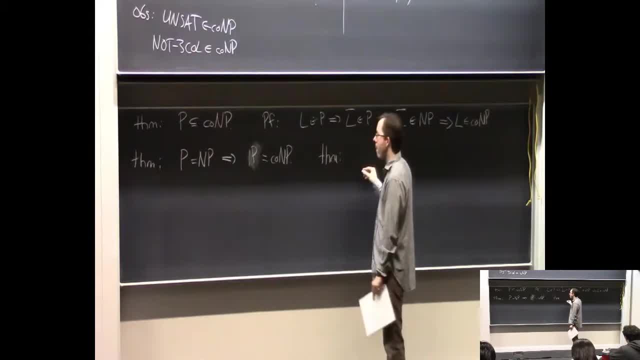 Okay, Oh, I guess that implies the thing I wanted to say. Well, I'll just write it again: If P equals NP, then also co-NP equals NP. Oh, I just sort of said that, right, If P equals NP, then co-NP equals P. 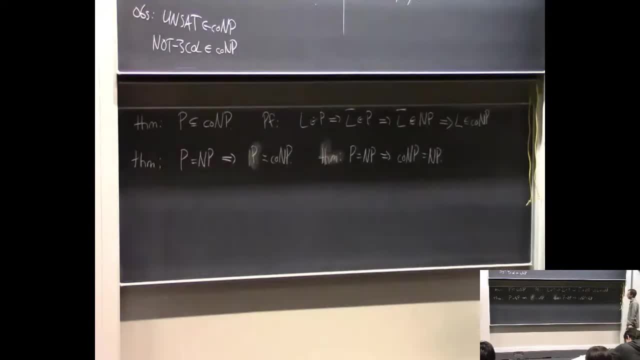 So, like all three of them are the same. What I like about this fact is the contrapositive. Let me just take the contrapositive of this, which is that if co-NP is different from NP, then P is different from NP. 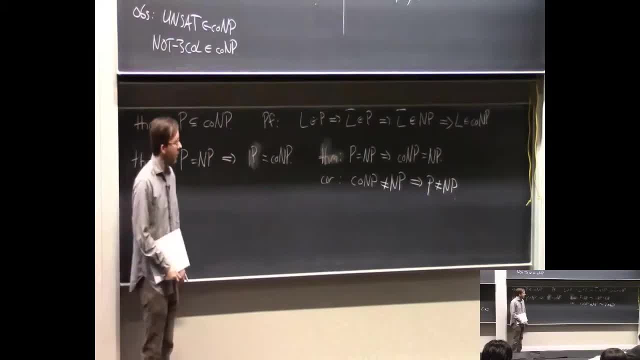 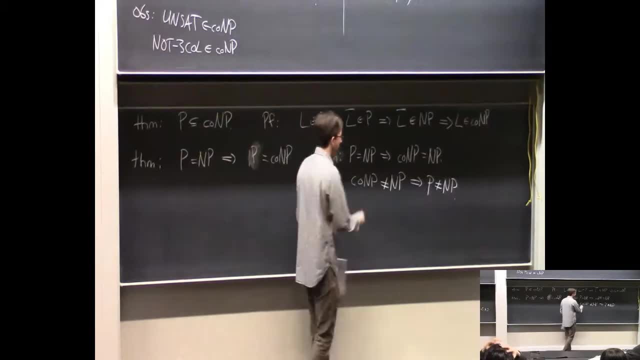 So I said earlier, like so far, it's going to just look like we're playing around with like trivial definitions, but it is worth it. So this is quite interesting. actually, What this says is that this is actually a stronger hypothesis. 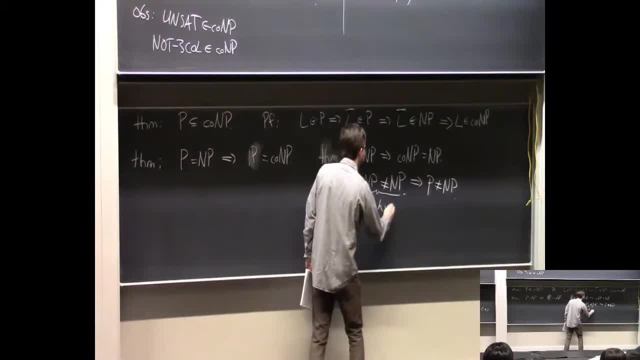 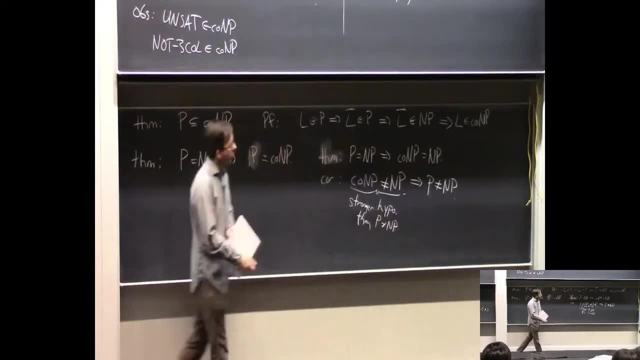 than P doesn't equal NP. Okay, so kind of our life-operating hypothesis in complexity theory, like our basic one is that P and NP are not the same, But we've talked about how it seems that even stronger things are true. 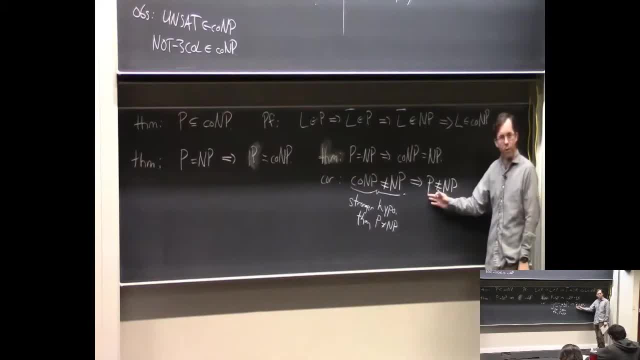 Like the exponential time hypothesis says: not only does SAT not have a polynomial time algorithm, like it doesn't even have, like it says actually that 3SAT doesn't even have a subexponential time algorithm. And this is like another example of an even stronger hypothesis. 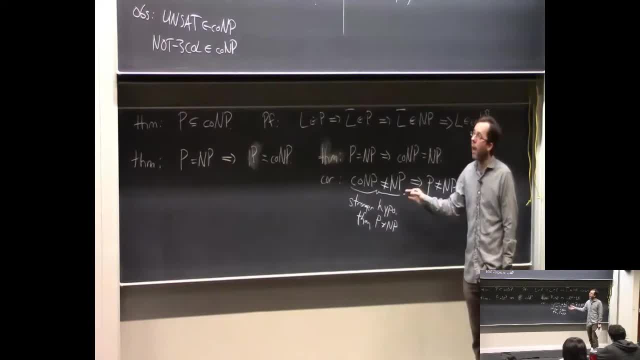 than P does not equal NP. So this is like another example of an even stronger hypothesis than P does not equal NP, A hypothesis that NP and co-NP are different, which, as we'll see in about one minute and it gets back to your question. 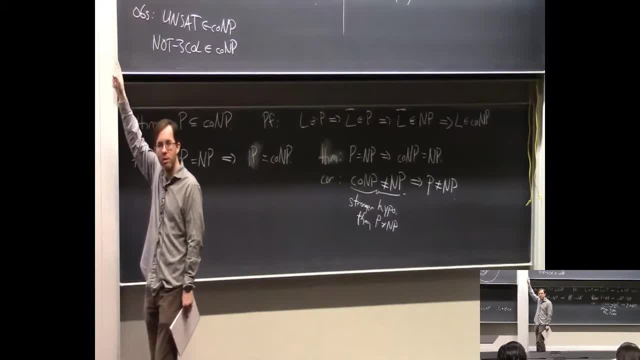 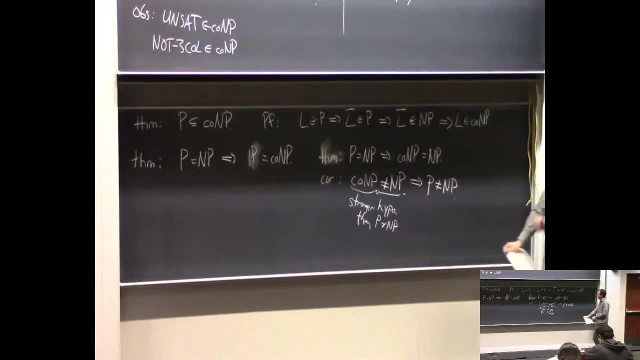 it'll turn out. that's the same as saying that the answer to this question is no, Okay. so I mean, if you believe this, you may or may not believe this. I think most people also believe this. So I mean, most people believe that NP and co-NP are different. 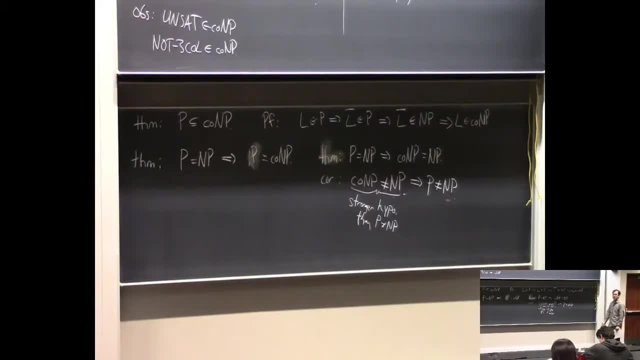 which, as we'll see, I guess basically now that the answer to that question is no, Okay, So let's in fact exactly do that, Okay, Wow, Wow. the same as co-NP is the same question. 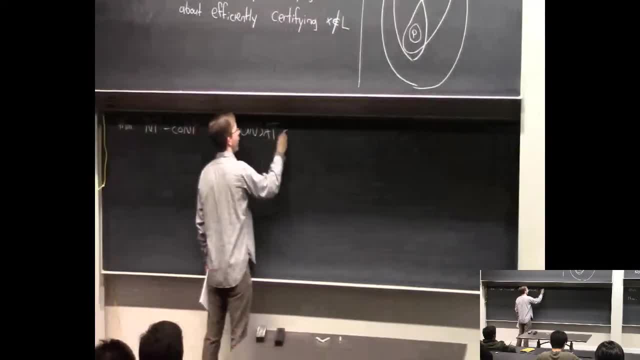 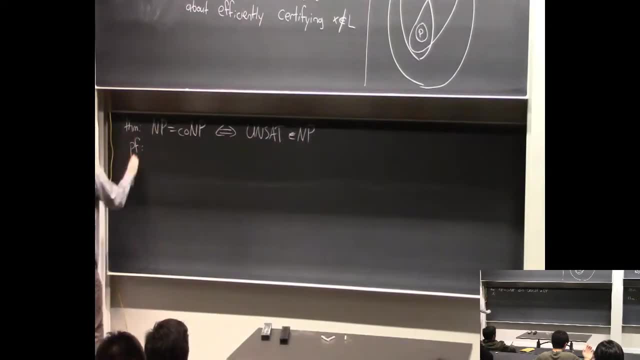 as whether or not unsat is in NP. Okay, so we have to prove two directions here. One of these directions is easy. Which one is easy? That's right. this one, yeah, From my perspective, stage left, it's this way. 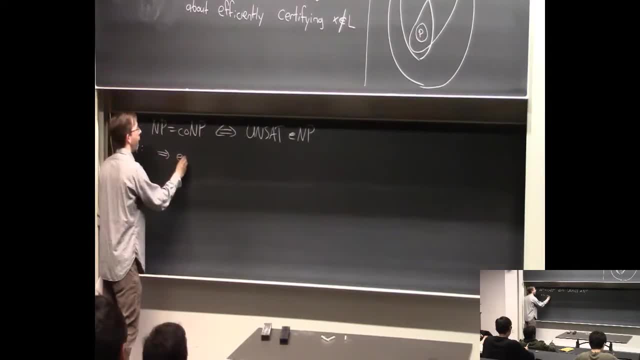 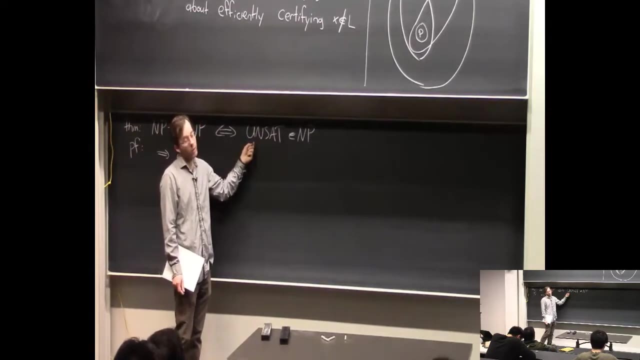 That's right. So it's. this way is easy. So why is that? Well, let's suppose co-NP equals NP. Well, unsat is in co-NP. It's practically how we define co-NP. Then, if co-NP equals NP, then unsat is in NP. 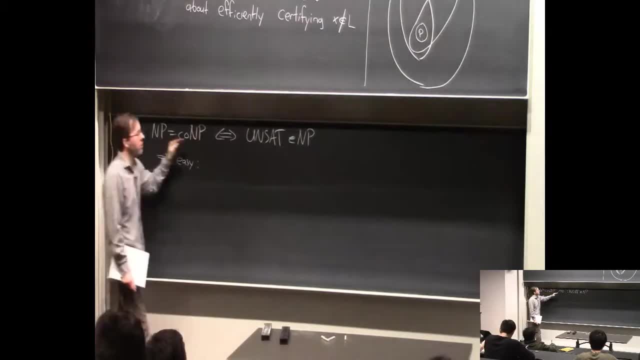 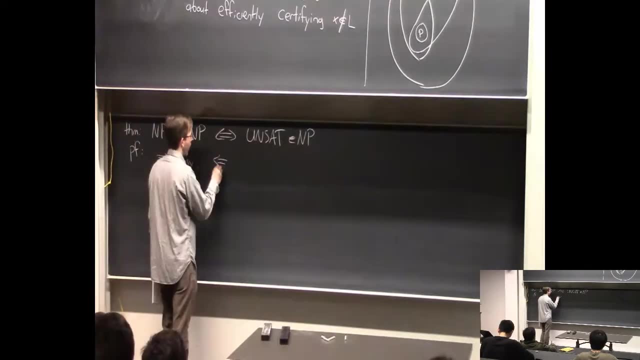 So the question is: how does it go down? Okay, So this is like the more general statement, This is the more specific statement, But the reverse is going to be true as well. And what basic fact do you think we'll use in proving the reverse? 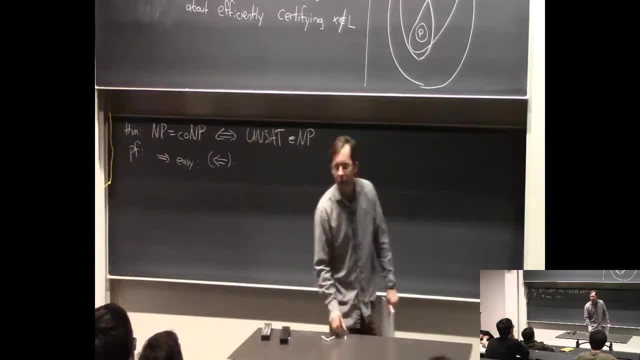 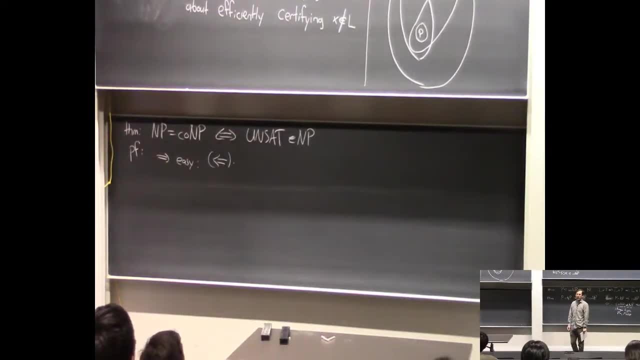 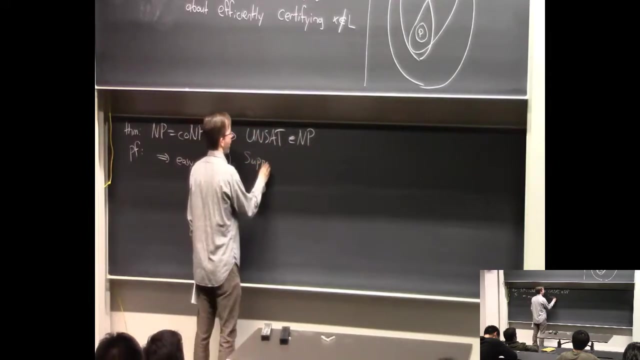 It's a theorem you learned in 251.. Yeah, All right, All right, All right. Well, we can also just start trying to prove it and see what happens. Let's just try that. Let's say: suppose unsat is in NP. 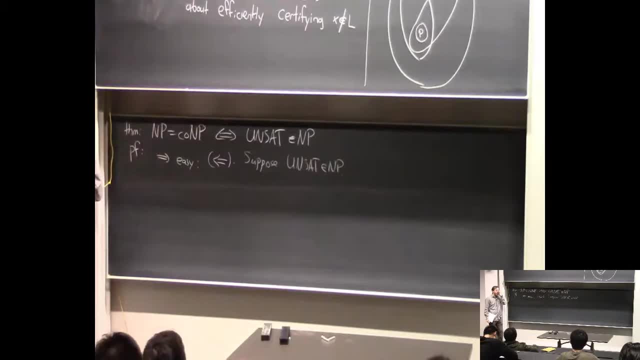 Now we have to prove that NP equals coNP. So actually you have to prove two things: Everything in NP is in coNP and everything in coNP is in NP. That's how you prove two sets are equal. Let's first prove that everything in coNP is in NP. 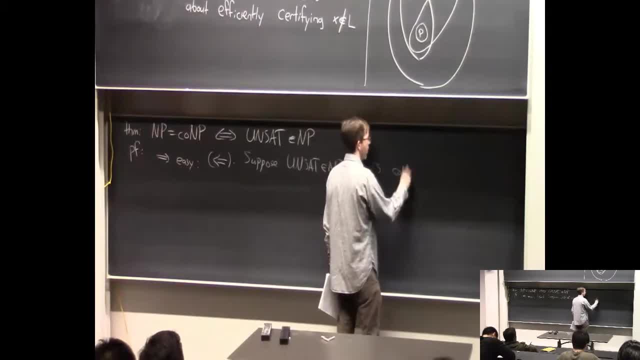 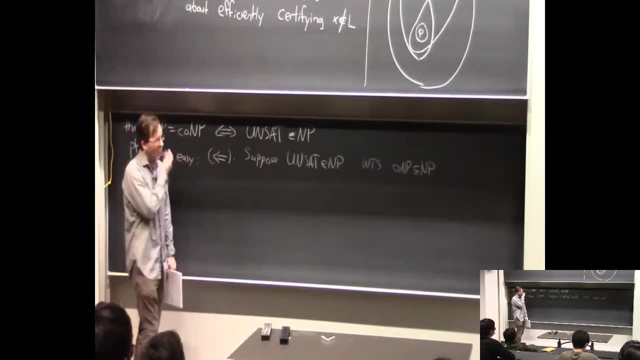 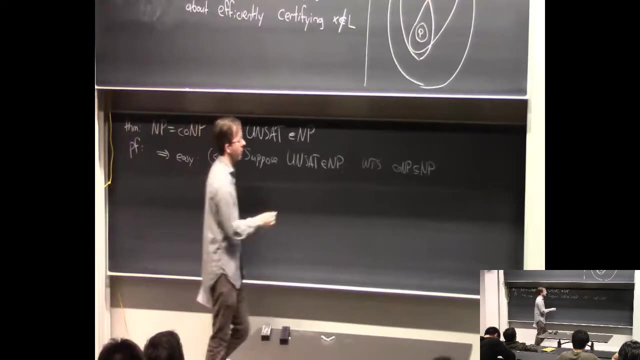 So say: we want to show now that coNP, among other things, is a subset of NP, The other direction is going to be basically the same. I can just co both sides, actually, after we're done proving it. So what we do is say: let L. 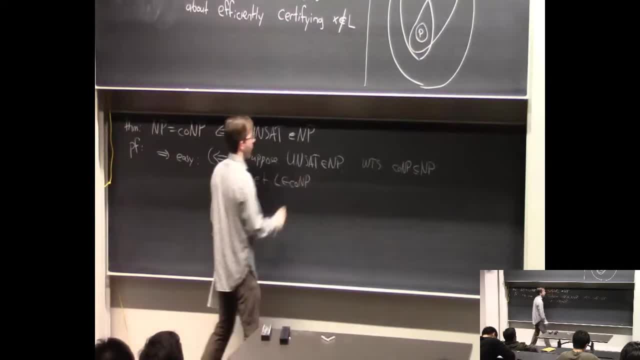 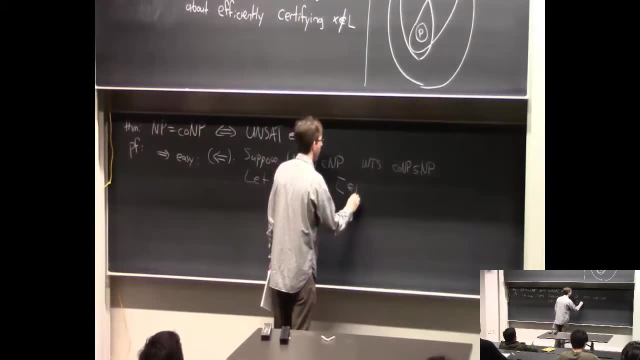 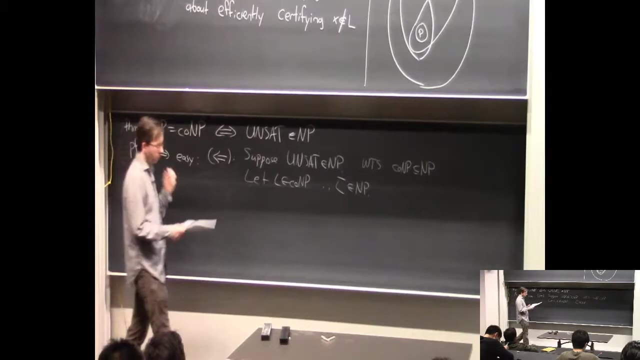 L be in coNP, You have to show that it's in NP. We can only take one step here. We'll say, therefore: L bar is in NP. Now what should we do? So we're working under this amazing assumption that somehow, unsat is in NP. 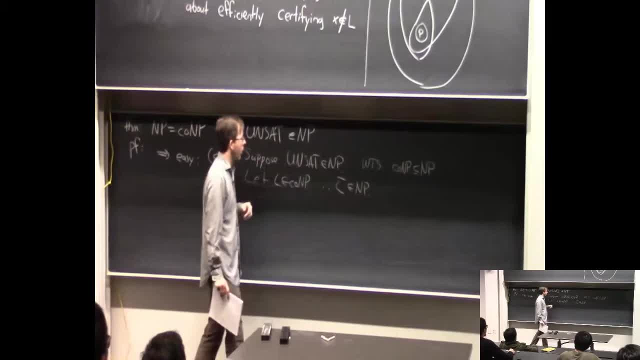 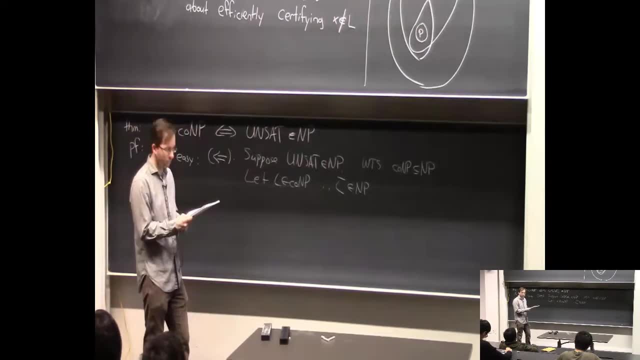 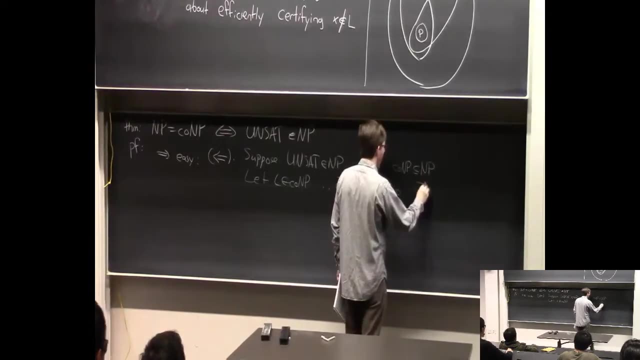 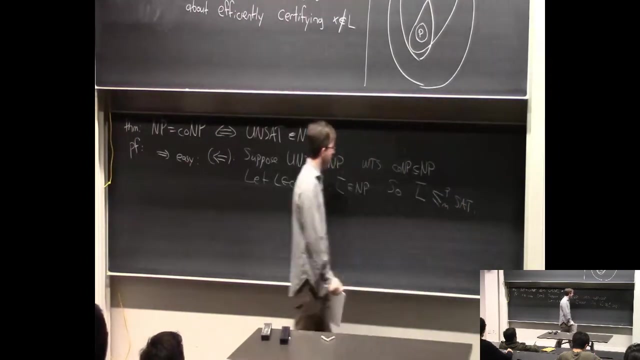 And what we have to do. we have to show that this particular L is also in NP. I'll keep going. So L bar reduces to sat. I mean every language in NP reduces to sat. That's Koch-Levin theorem, OK. 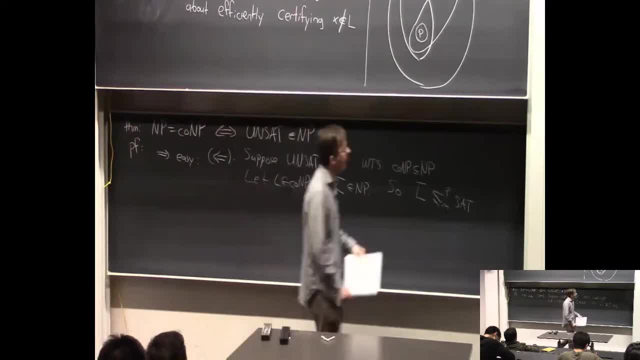 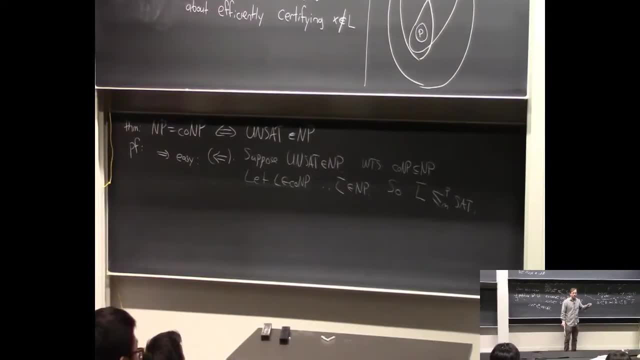 OK, OK, OK, Now let's bust out this one. Hopefully I still saved it. I mean, if you just write down the definition of this and then use this trick, that p, if and only if q is the same as not p if and only if not q. 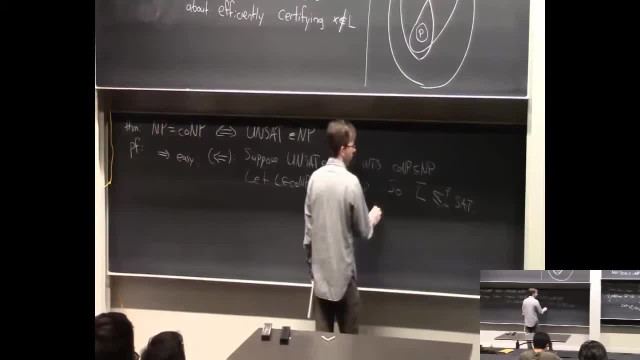 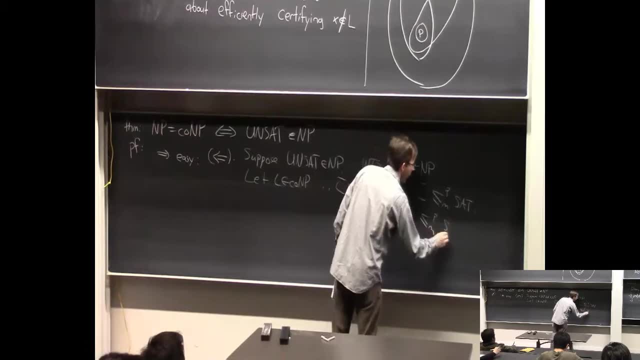 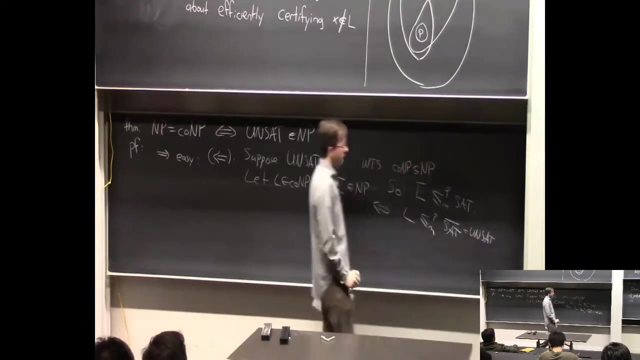 And you see that this is literally equivalent to L, H and P OK. L reduces to the complement of SAT, which is unsat. And now what? Yeah, Now we know that unsat. we assume that SAT is an NP, so L is also an NP. 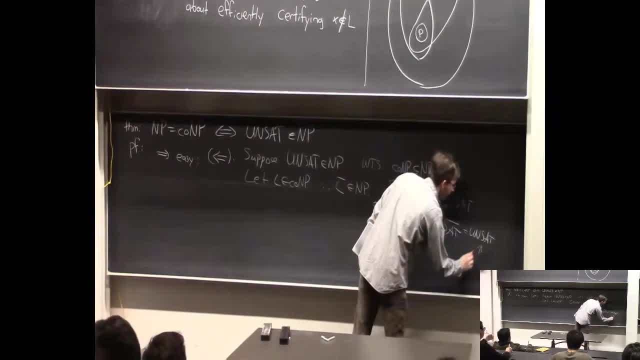 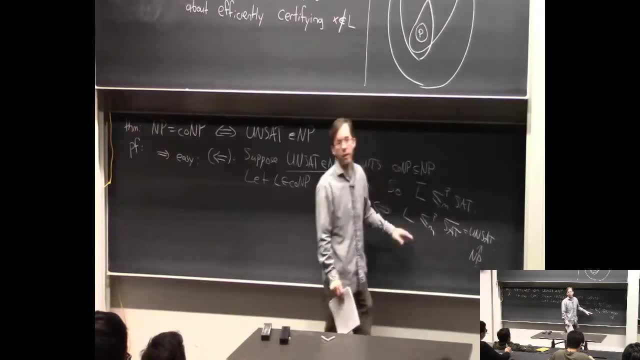 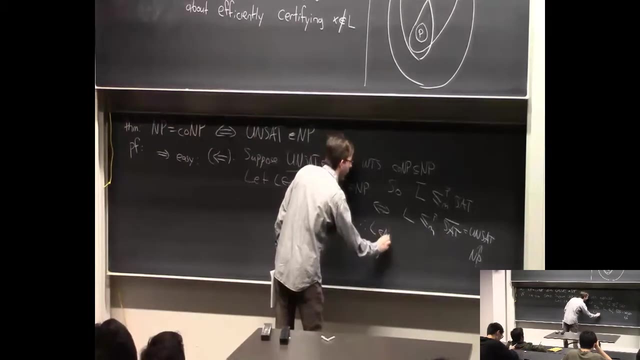 Right, So this is an NP. That's like the assumption we're operating under And we have this fact that if L reduces to a language in NP, then L is an NP OK. so therefore, L is an NP. OK, so that shows this. 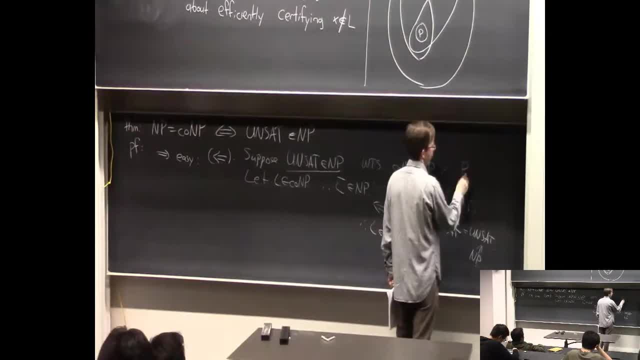 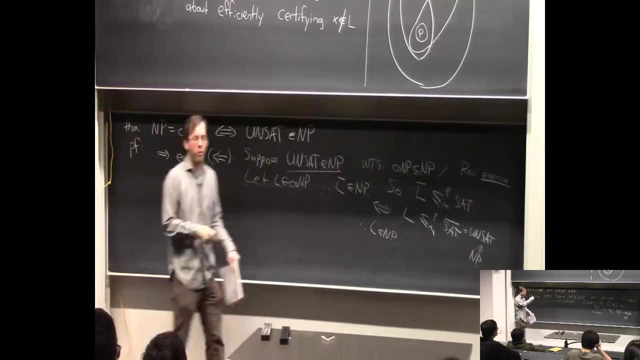 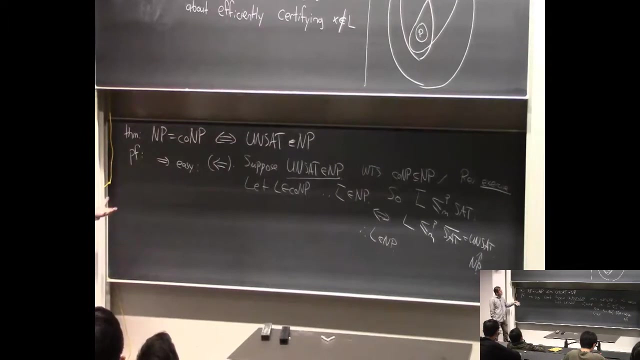 And let me say the reverse. I'll leave it to you. Basically, you just repeat this proof with negations everywhere, complements everywhere. So basically, I mean it's almost syntactic, this proof. It didn't really have much insight. 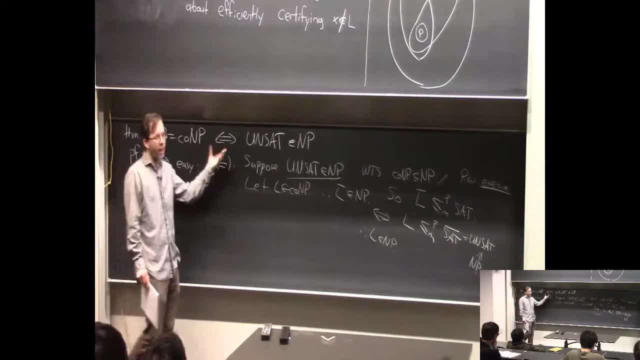 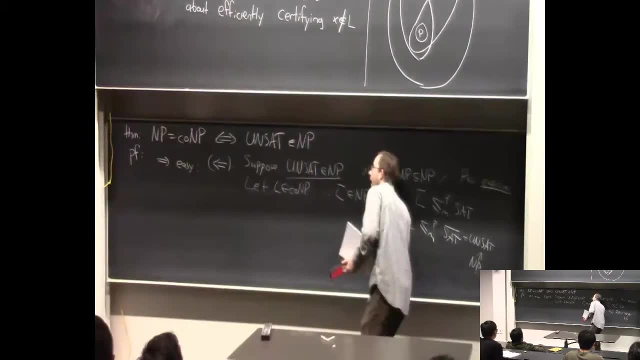 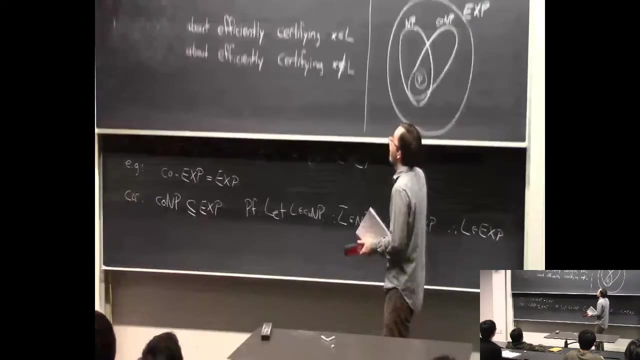 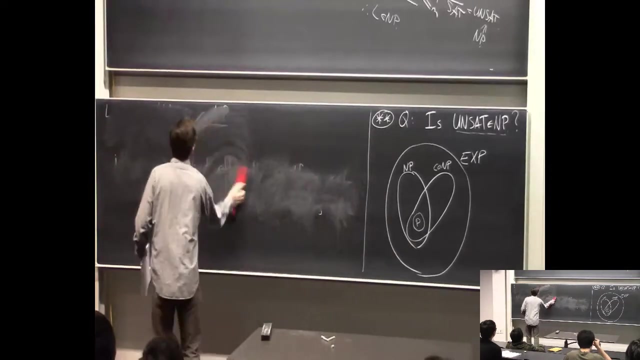 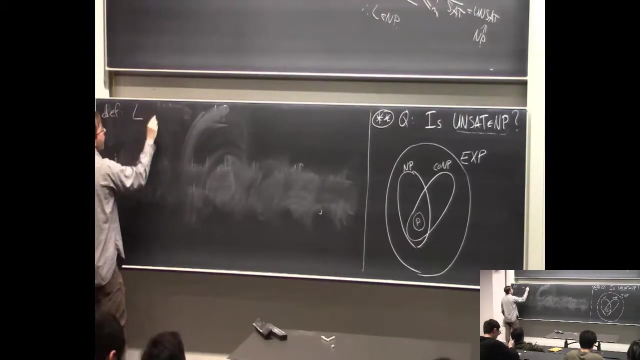 Basically what we proved, and I'll write this down. What we'll write this down just now, is that sort of unsat is co-NP complete. So unsat is like the hardest problem in co-NP. OK, So let me make this definition. 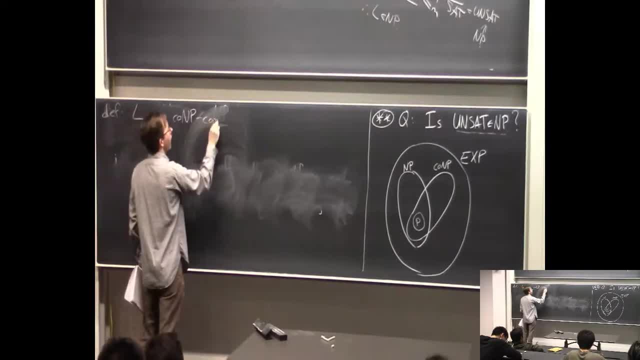 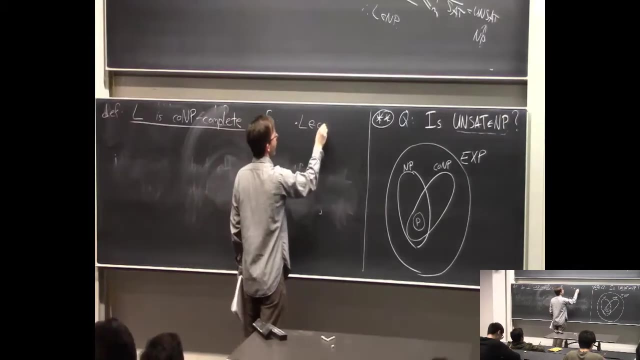 L is co-NP complete. It's the same definition, I mean it's the same idea as NP complete. Like you want to find the hardest problem in co-NP. So if two things, as always, L is in co-NP. 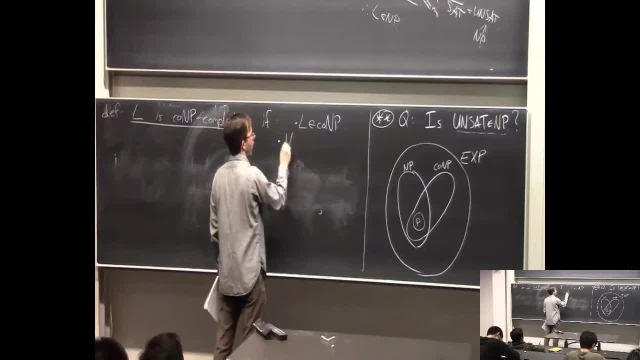 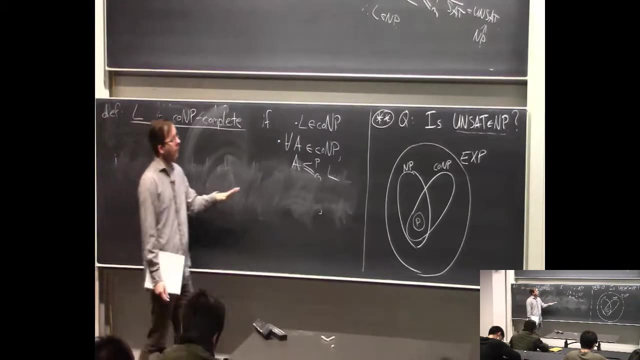 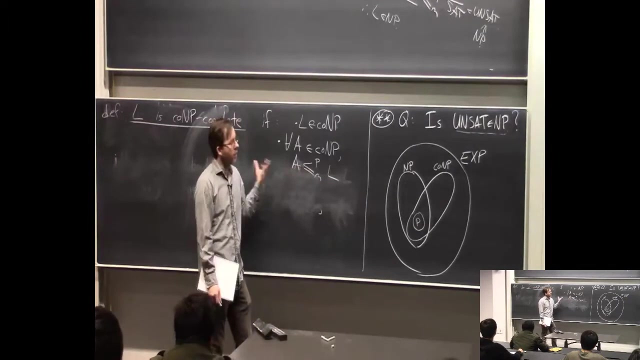 and also every language in co-NP reduces to L. I suppose for this definition to be reasonable, you should know that, like in the first case, we're going to look for the problem in co-NP. The problem: we know that if A reduces to L and L is in NP, then A is in NP. 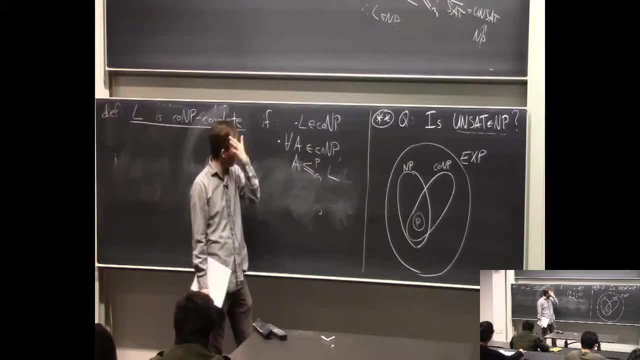 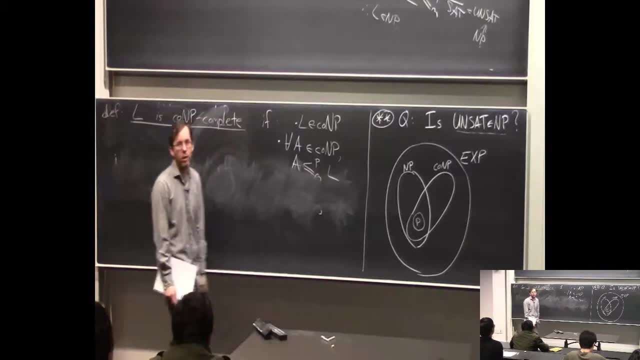 That's kind of helped us make sense of this definition of NP complete. And it's the same thing for co-NP. If L is in co-NP and A reduces to L, then A is in co-NP. It's the same proof. OK, So it's helping us look for like the hardest problem in co-NP, In other words, the problem that's in co-NP that's like least likely to be in P, and then it's the hardest problem in co-NP. 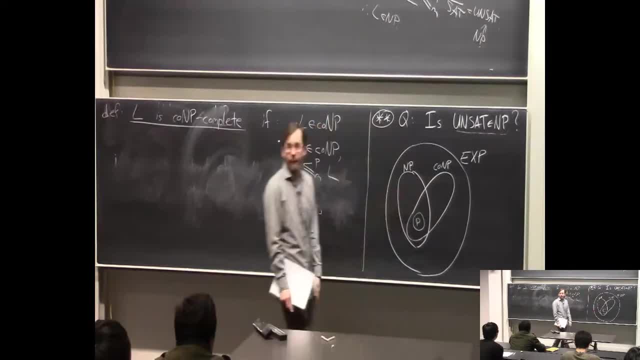 The problem is like the problem that's in co-NP And then it's the hardest problem in co-NP, And then it's the hardest problem in co-NP and also least likely to be an NP, So the one that kind of captures the true power of co-NP. 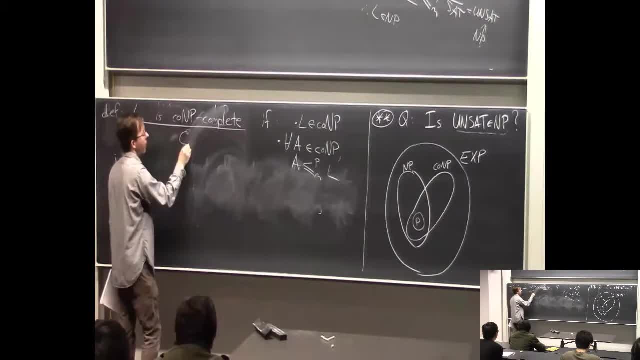 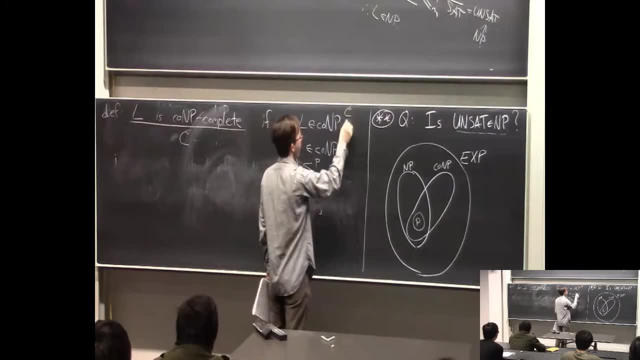 In general in life. by the way, again, you can also say they make a definition In complexity: L is C-complete for some class. if L is in C And for all languages in C, they reduce to L. So you can talk about completeness of other complexity. 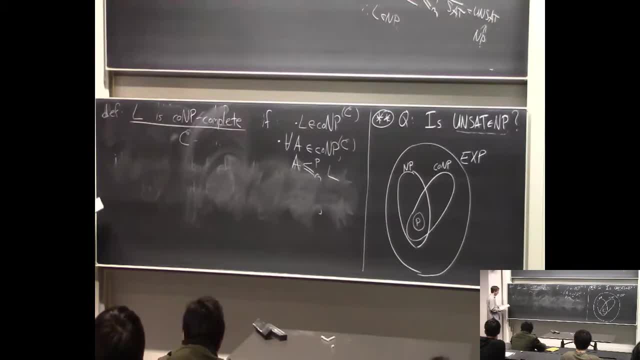 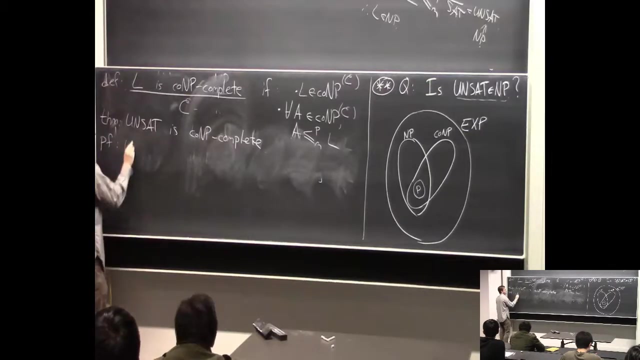 classes too, And indeed onSAT is co-NP complete. So let's prove this. Well, we have to check two things. First, that it's in co-NP, And that's definitely true. We started with that. 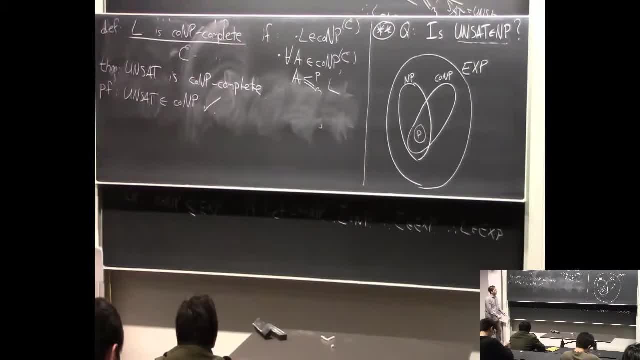 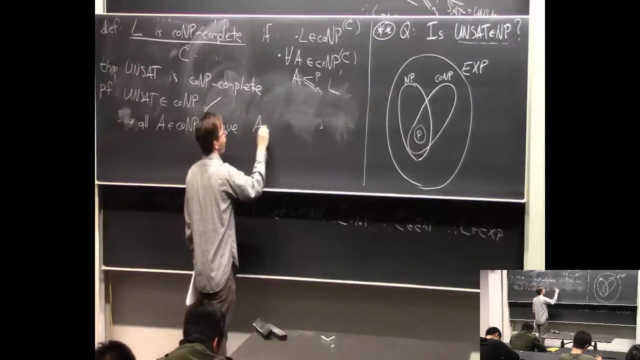 OK, now we have to check the second condition. But let's say: well, we know that all this is what we need to prove. all A and co-NP have A co-NP And we know that all A bar reduces to in polynomial time. 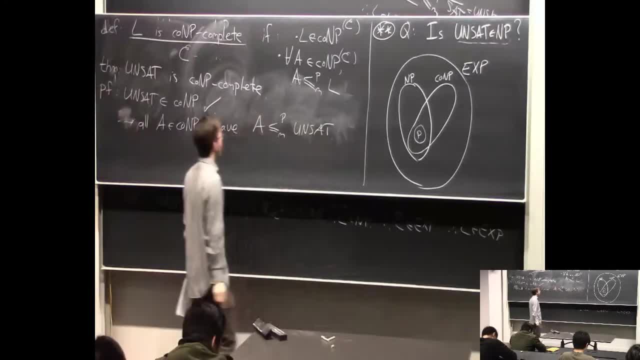 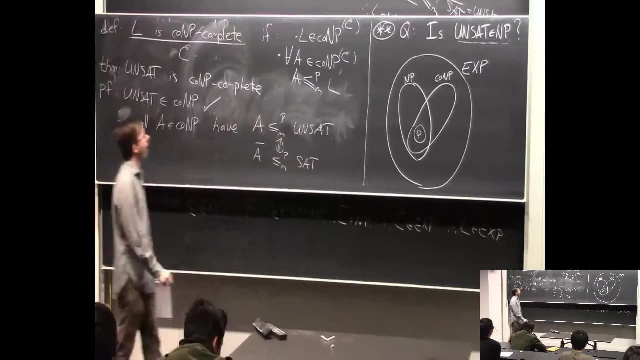 onSAT. Well, as we saw, with this little trick down in the corner and we used in the previous proof, this is literally the same as saying that A bar reduces to SAT And this is literally the same as saying A bar is in NP. 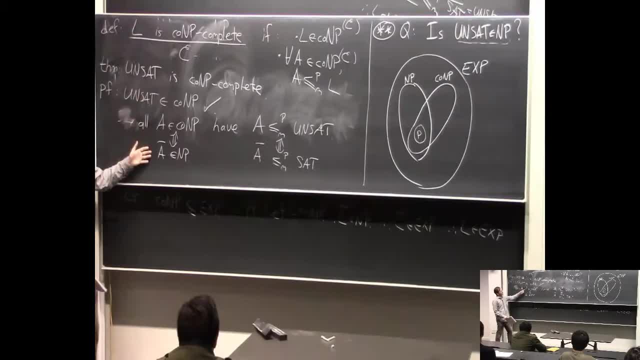 And indeed this statement which we're trying to prove in order to get the second condition of onSAT being co-NP complete, it's literally the statement that SAT is NP-hard. Every language which you can call the complement of some language, every language in NP. 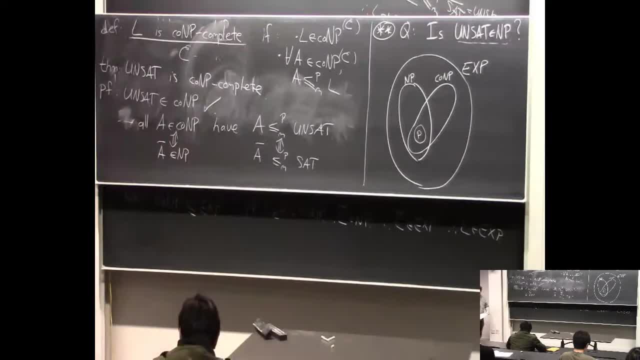 reduces to SAT. Any questions Again, you may still feel that it's like, well, we're just making a lot of definitions and syntactically reversing some things, But hang in there, OK, so in fact, the same proof, actually. 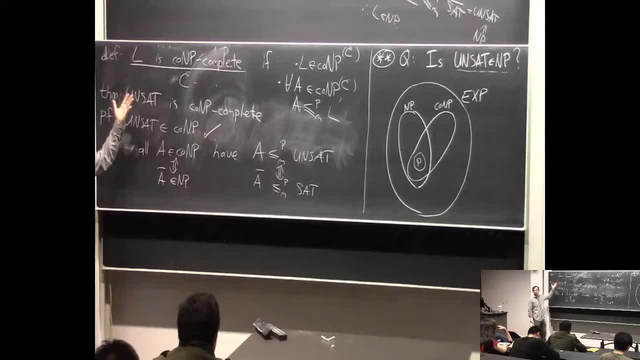 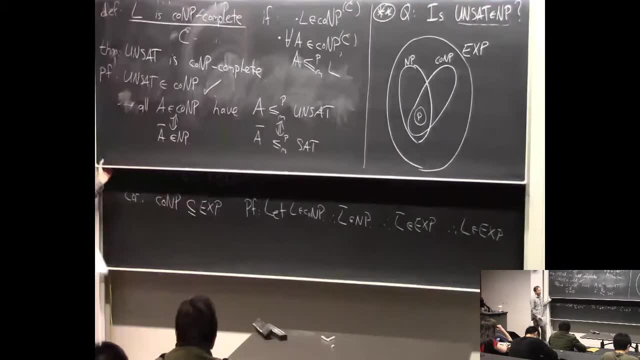 shows that if you take any NP-complete language, its complement is co-NP complete. It's not very surprising. So the problem of given a graph: is it not 3-colorable? That's co-NP, It's not NP-complete. 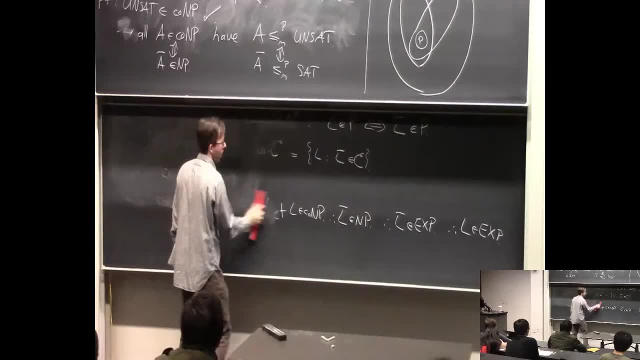 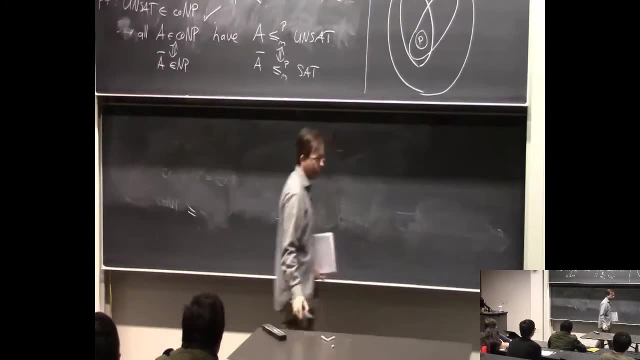 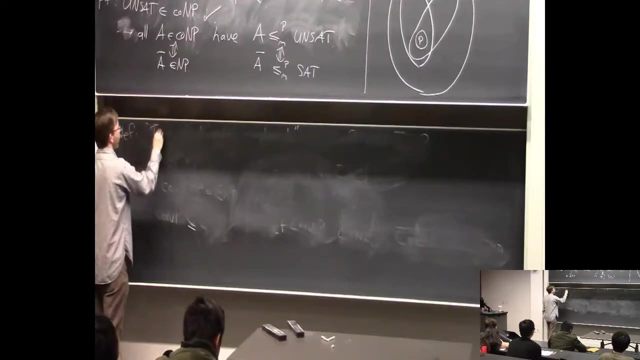 So now, just to test your understanding, I'm going to tell you another problem and ask you to place it in this picture. So here's a decision problem where a language is called tautology, And I'm going to stop writing the ology part. 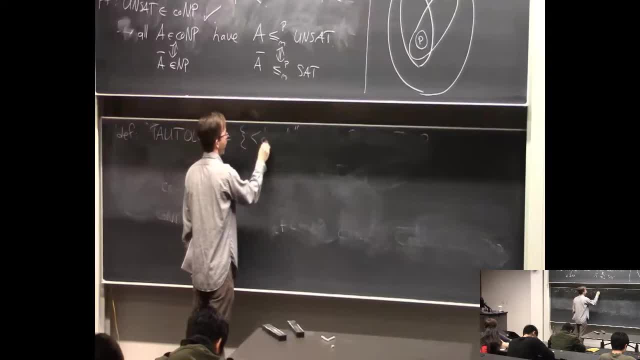 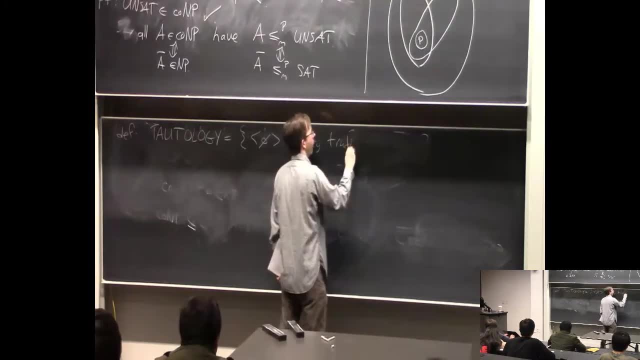 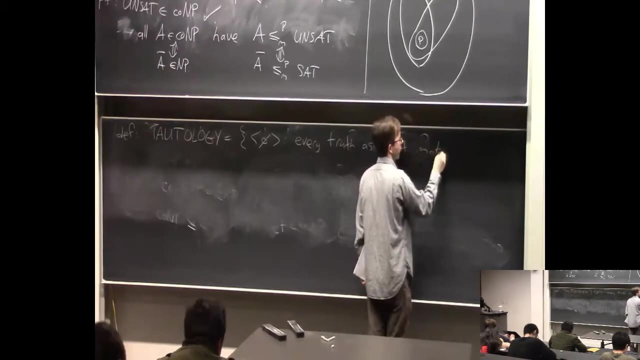 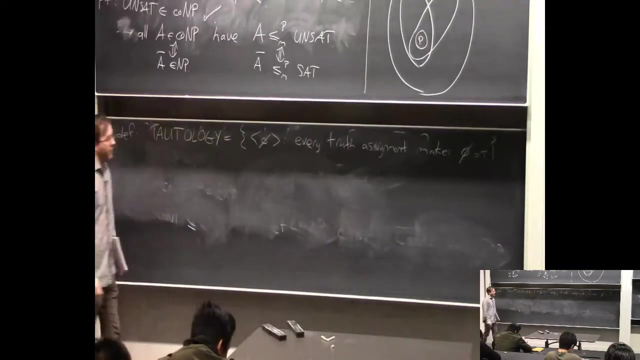 because it's very long. But tautology is the language of all Boolean formulas, such that every truth assignment makes phi true. No matter what you plug in true or false, you're going to get the same result. No matter what you plug in- true or false- for the n variables. 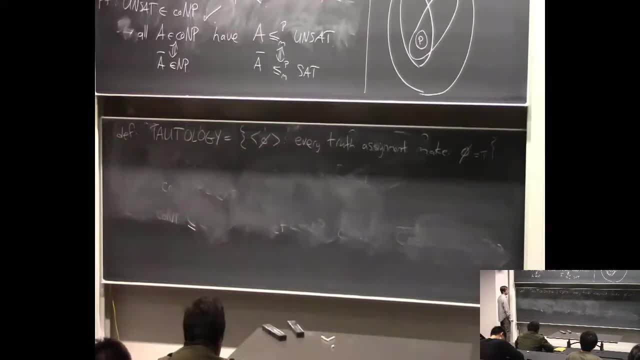 phi ends up being true. So an example string in tautology is like x, y applies whatever, not x or y. OK, you can probably put if and only if here. But no matter what you plug in for x and y. 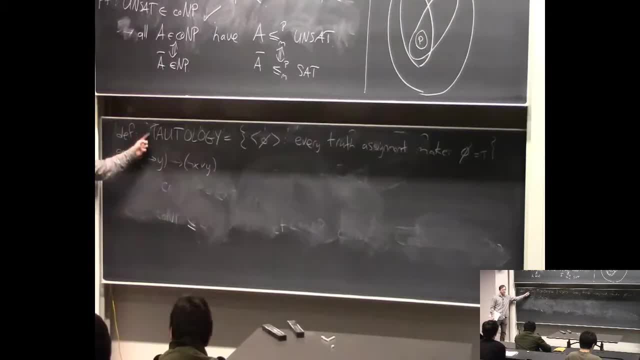 you'll get true here. So that's an example, So this is a string that's in this language. So it's kind of like the Boolean formulas that are sort of tautologically true, that are always true. They express fundamentally true facts about Boolean logic. 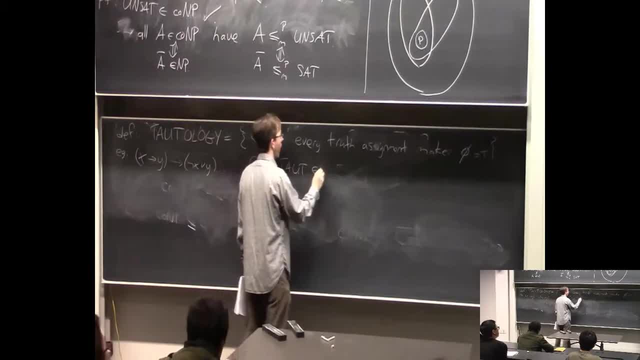 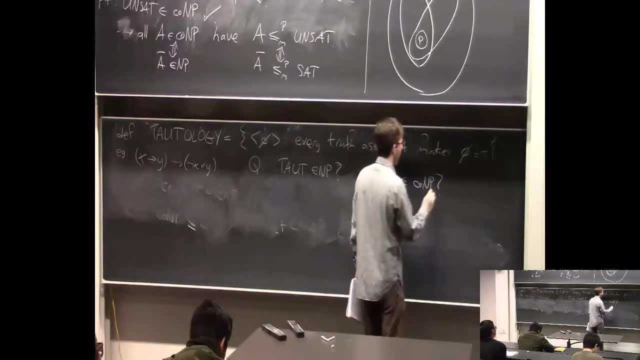 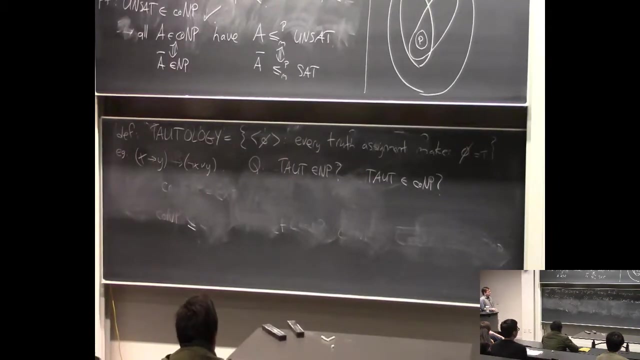 So here's a question: Is this in NP And also is this in co-NP? That is true, Correct? Somebody want to answer one of those two questions, Your choice. Which one to answer? Yeah, Right in the middle. 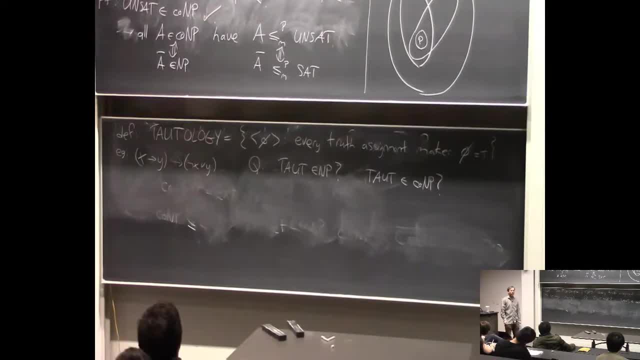 ANDY DOHERTY, The negation of the language definitely in NP, since you can take in a verifier that gets something that makes it false. So then that's just a in co-NP. That's right. If you didn't hear it, we got a proof that this is true. 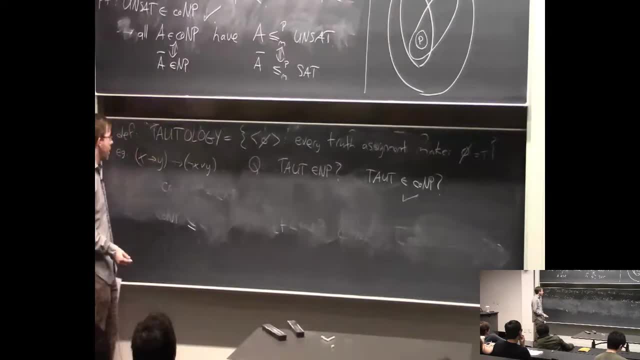 This is an example of a problem that's in co-NP. Why, Well, let's go straight to the definition, I suppose. What is the complement of this? It's all the phi's, such that all truth assignments. Wait what? 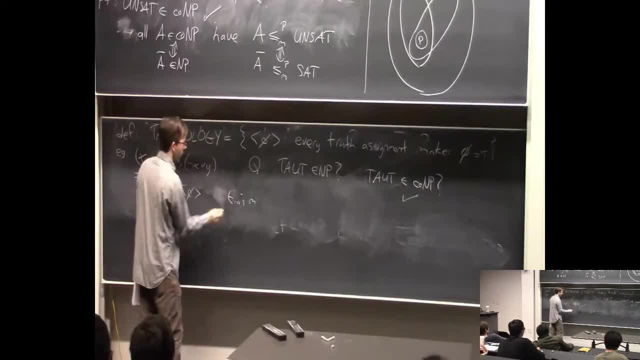 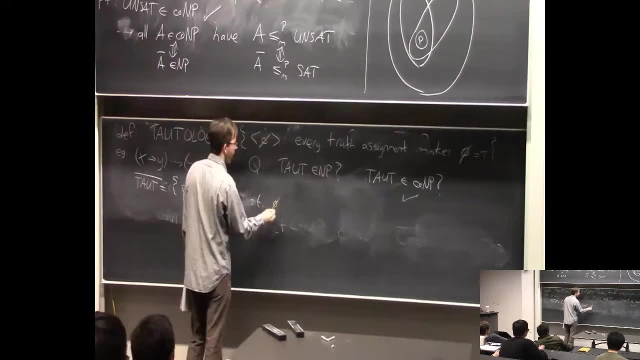 No, That's wrong. Failed to correctly negate There exists a truth assignment such that phi is not true. It's like all the Boolean formulas where there is a way to plug in truth values to get false. OK, And the claim was that this is in NP. 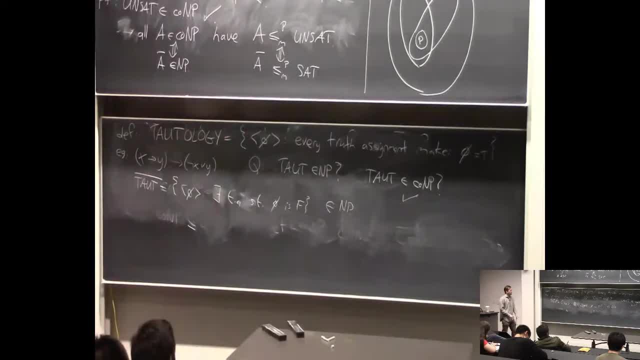 And that's kind of the statement that I mean. if you just think about it for a second, I hope you're kind of comfortable with. So all Boolean formulas where there exists a truth assignment that makes it false. So why would that be in NP? 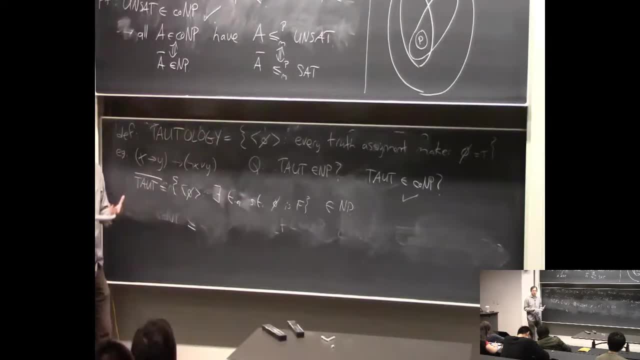 As mentioned, you could have a verifier that expects to get as a certificate a truth assignment that makes phi false. So the verifier, It takes phi and this truth assignment that expects to make phi false and then just plugs it in the truth assignment into phi and checks. 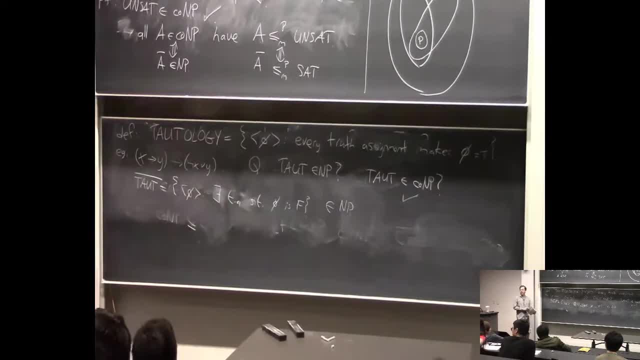 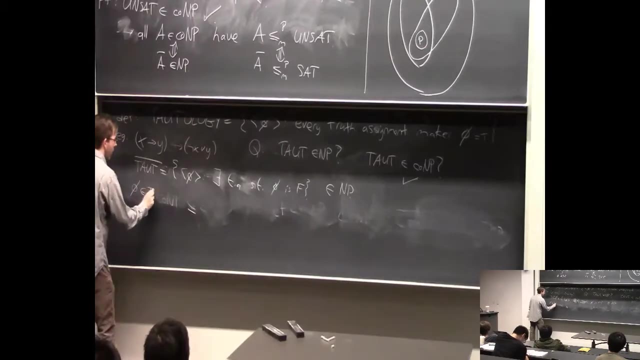 that the outcome is false. Yeah, It's like the dual: Every truth assignment exists. if there exists a truth assignment, Right, It's like the. so, for example, phi is in top far if, and only if, Negation of phi is in sat. 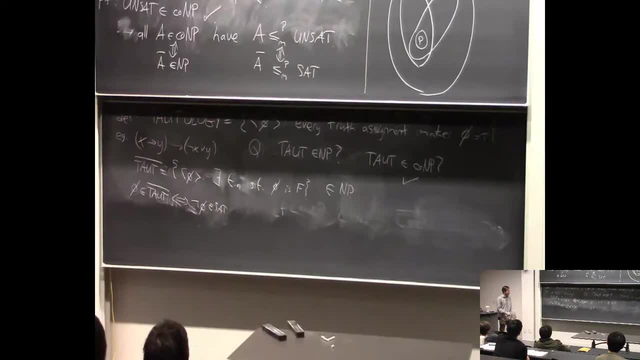 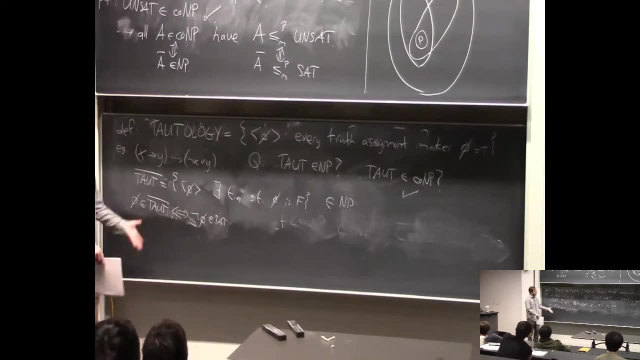 Now there's all sorts of negations going on in every different place, So you may find this confusing, but reflect upon it. I mean, if phi is in top, it means there's at least one way you can plug in for the truth assignment for the variables. 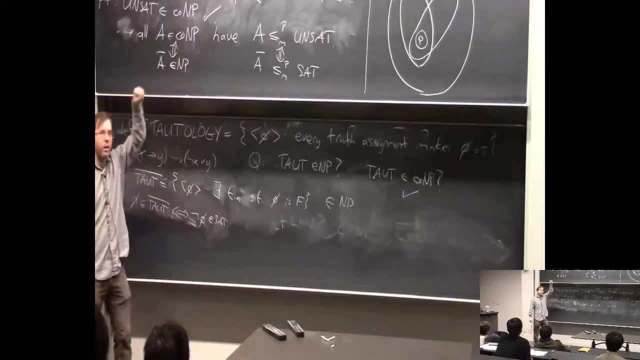 to make the outcome false. If you just replace phi by put a not at the end, that would be like saying there exists a true assignment that makes phi true, which is sat. OK, so there's a very easy reduction from the complement of tot to sat. 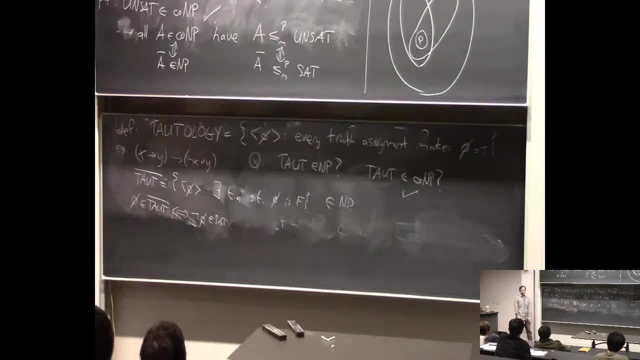 Just take phi and stick a not at the front. OK, So what about this question? Is it in NP? Well, once again, it's very similar, and I'll stress this again in a second. It's very similar to our very starting question. 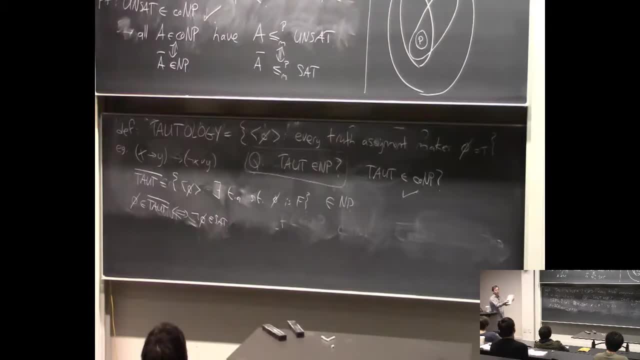 is unsat in NP. It's not clear, right? Suppose I come along and give you a Boolean formula and I swear this is a tautology And you're like: I don't believe you prove it. I'm kind of stuck right. 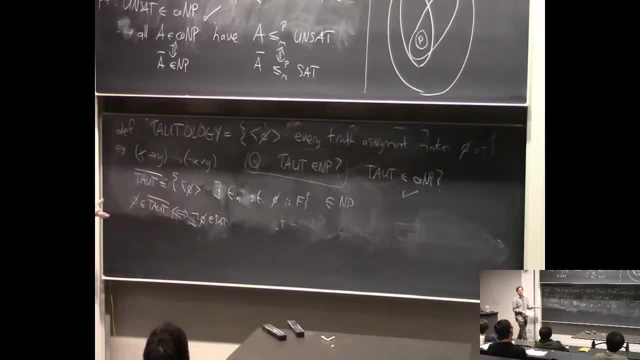 I can't just show something to you that will make you think it's a tautology. At least it's not obvious. I can show you a few truth assignments and be like check it out. they all make this formula true. But you would say, yeah, but I have to prove it. 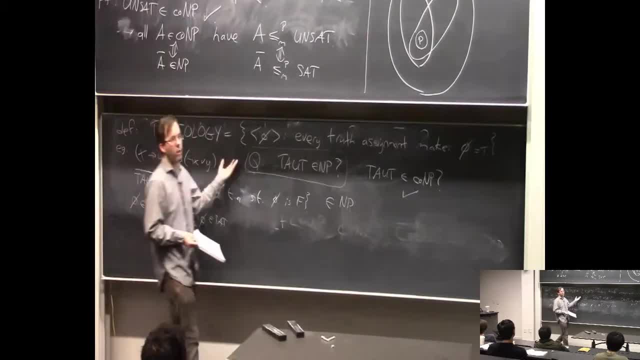 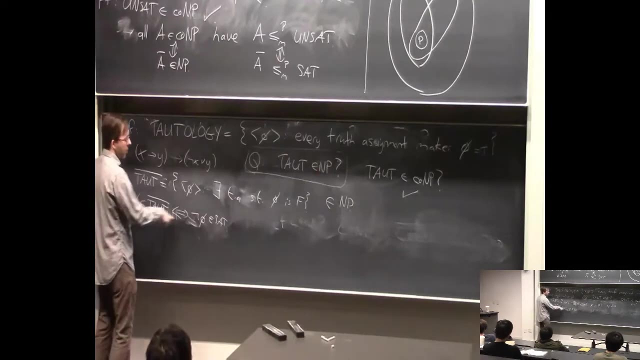 I have to be convinced that all truth assignments make this formula true. It's not clear how I can do that, So because of this fact, there's actually reductions between these two problems. It's easy. maybe I'll call it an exercise. 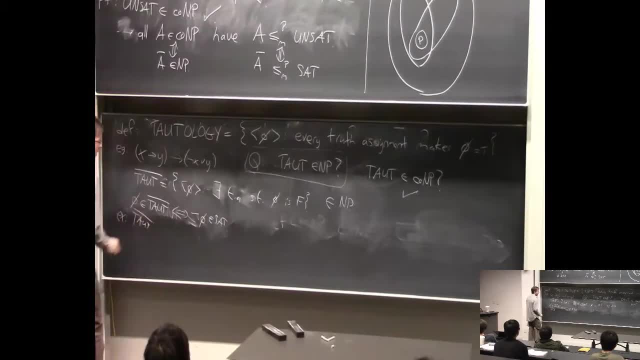 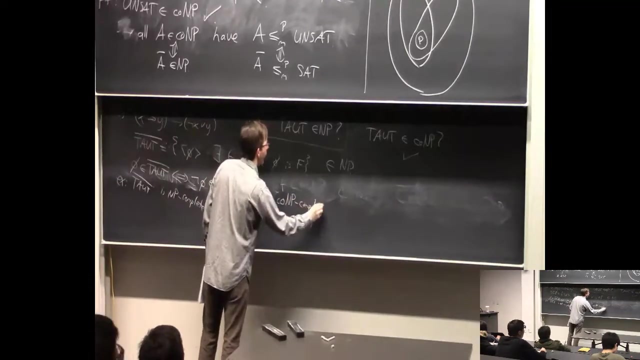 to show that, or you could prove this, that the complement of tot is NP complete. This language is NP complete which, as we know, implies that tot is co-NP complete. So tot is tautologies, is like another language. 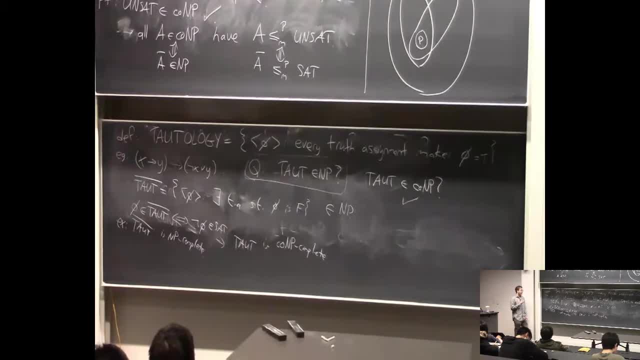 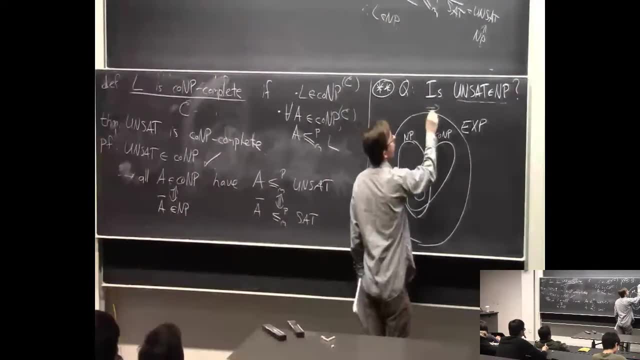 which is co-NP complete. It's like the hardest language in co-NP. Let me just write something here. So So this is equivalent to. we know this is true if, and only if, NP equals co-NP, And so we now also know that this is true if, and only. 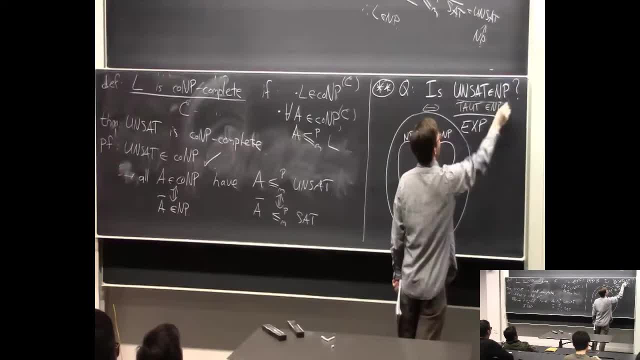 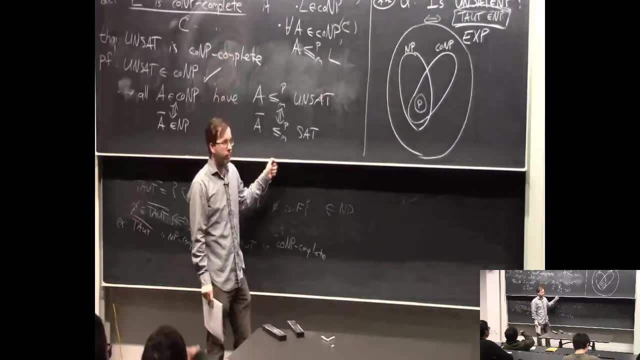 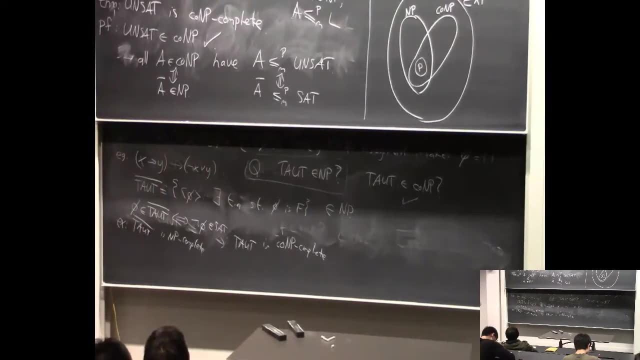 if tot is in NP, because tot is also NP complete, Sorry, co-NP complete. Yeah, Are there methods in the first-order logic where you can back out the steps or something like this in a fridge diagram? Yeah, so the question is, you could try to. 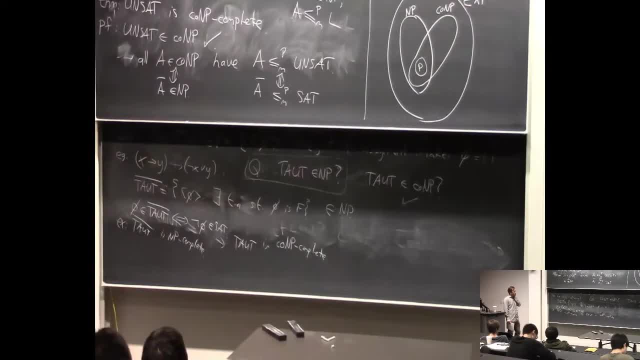 if I give you a Boolean formula, I could try to like convince you that it's a tautology. I mean, one thing I could do is I could just write down the truth table for you and be like check it out. 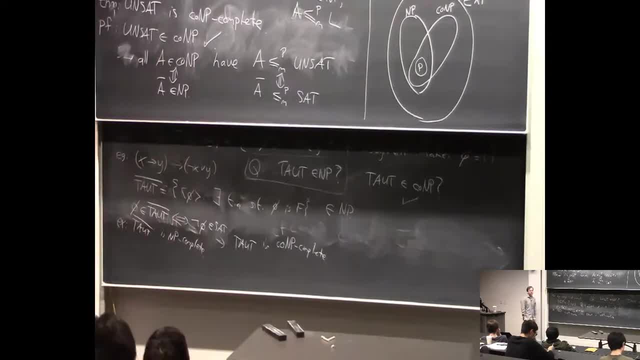 I wrote down the truth table. It's like all truths in the truth table. But that would not help you show that it's an NP, because that would be like an exponential length certificate. I could also try to prove it for you like. give it a proof using rules of first-order logic. 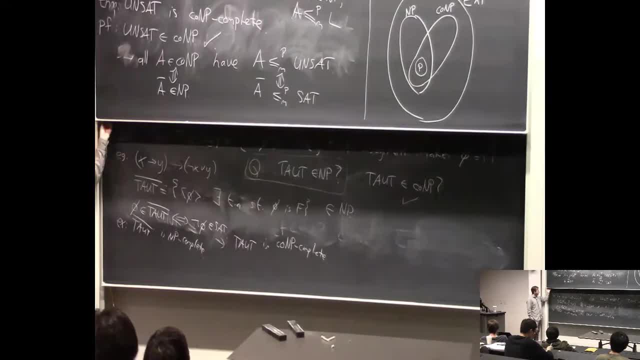 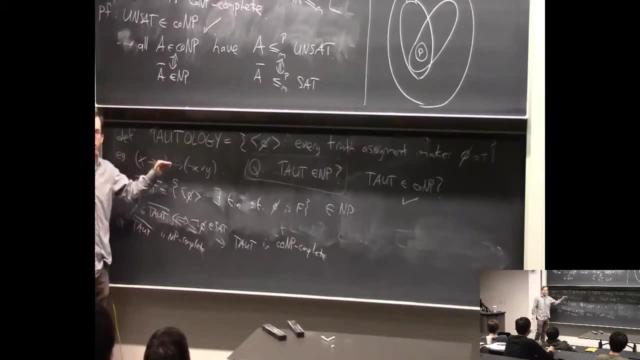 depending on when you took 251.. We might have talked about that, Like You know, like modus ponens and stuff, But like it seems to be just a fact that there are tautologies where, even though they're true, 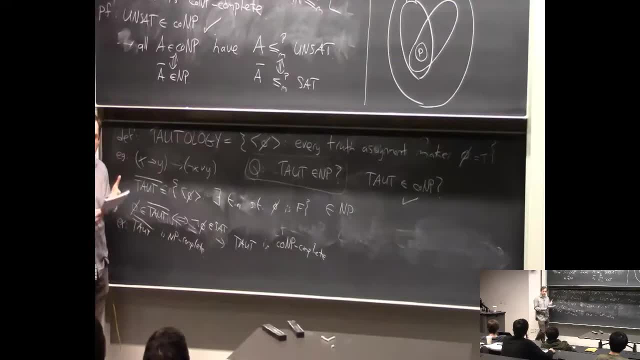 like there's no short explanation of it, Like there's no short derivation of it in like a system of first-order logic, seemingly Yeah. So I mean, this exact question is why I mean I think co-NP versus NP is very, very interesting. 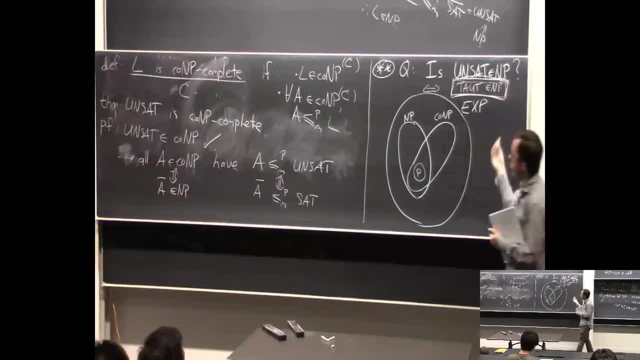 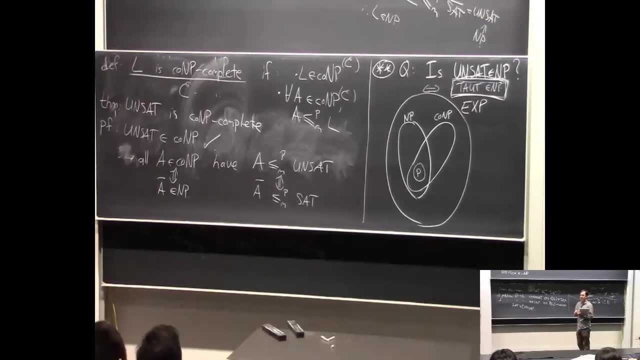 As I said, it's the same as this question And this is really. I mean it gets to your question. I mean it's a very fundamentally interesting question, Like if you think of the language tautology as like the set of all Boolean formulas, that 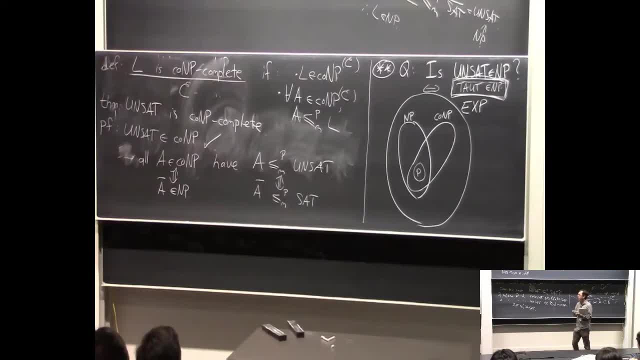 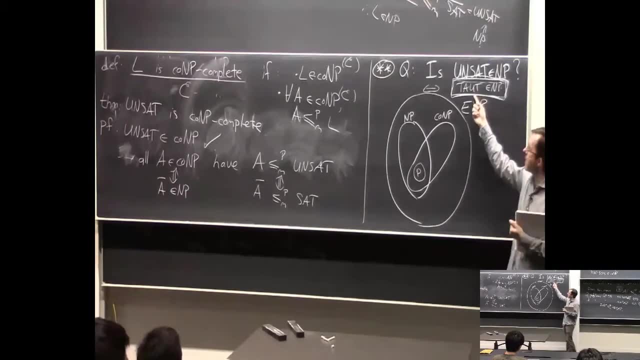 are like fundamentally true, in the sense that, like they're universally true, it's no matter what your interpretation is. like phi is true, And this is really like saying like, if you have like a fundamentally true statement, is it the case that it also has an efficient proof? 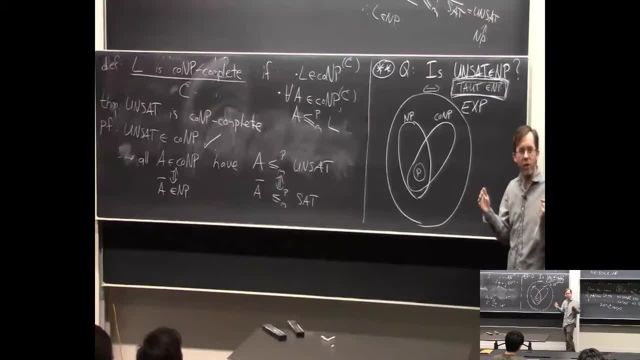 that it's true. Like a short polynomial length certificate, that it's true. It's almost like saying, like does every theorem that is true have a short proof? That's somehow like the real idea about co-NP versus NP. Like, does everything that's like fundamentally true? 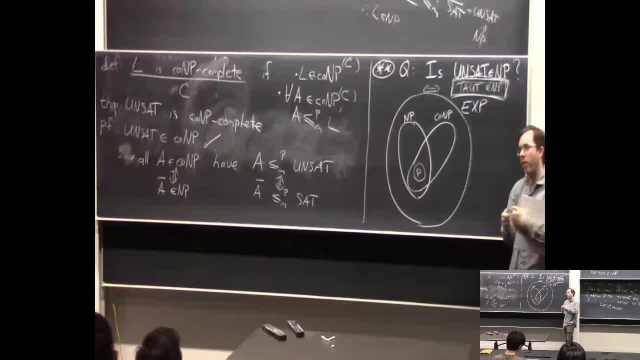 have like a succinct certificate that it's always true. So as opposed to just literally checking all the cases, I'd be like writing down the whole truth table. Can you always come up with some like short certificate of a proof of a theorem that somebody could check? 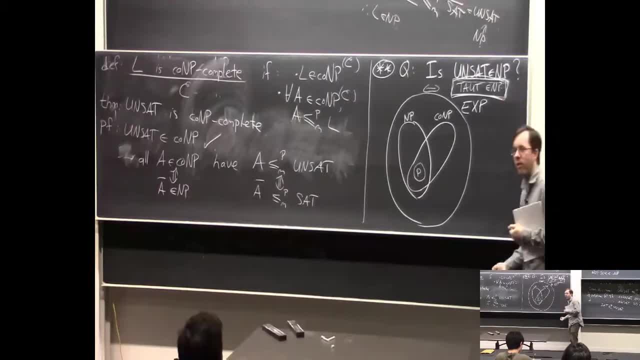 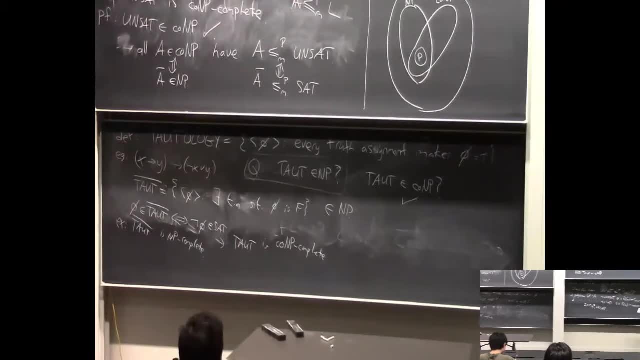 OK, So that's one reason, at some of like a philosophical level, why these questions of NP and co-NP are interesting. OK, And let me even kind of um Expand upon that sort of philosophical way of looking at it. I mean, we started with kind of like a boring definition. 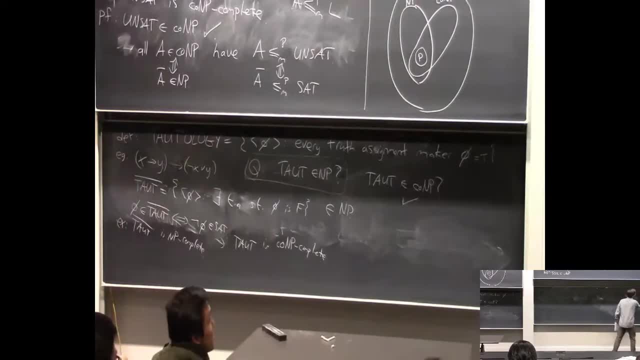 where we said, OK, co-NP is all the languages whose complement is in NP. But an interesting thing to do is just take the definition of NP and like plug in the complement and just see what it looks like OK, And that'll kind of come back to this question. 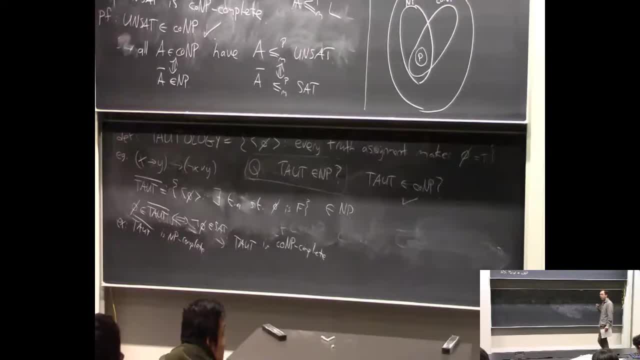 And the original question was like: what's NP, What's co-NP, What's co-NP? And the original statement I had on the board, that co-NP is kind of like all about proving when a string isn't in the language. 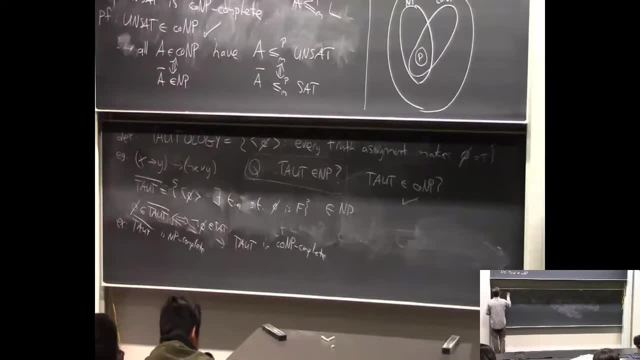 OK, So we know that L is in co-NP if, and only if, Well, there's a verifier, polynomial time verifier, for L bar the complement of L. So, if there exists this polynomial time algorithm, vxy, which is in poly length of x time, 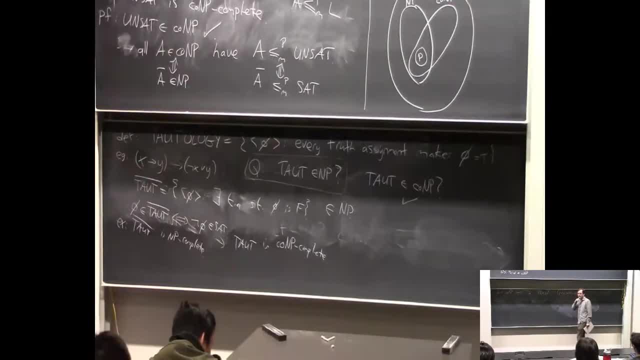 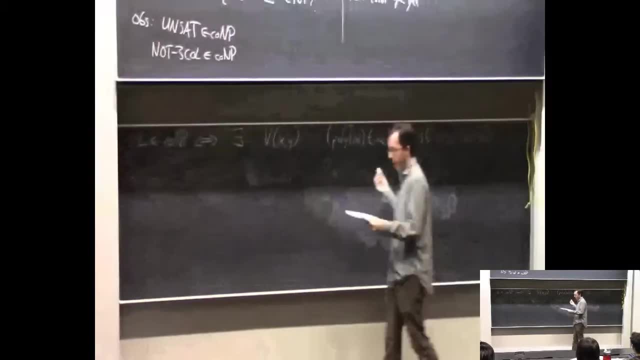 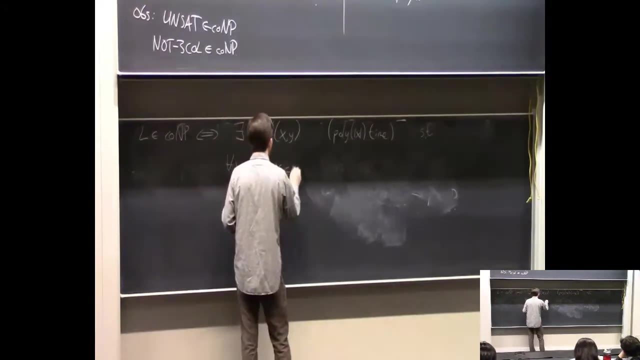 that verifies L bar. L in being a co-NP is the same as saying that L bar is in NP. So let's just write down what that means, such that you verify L bar. Well, it's just that, for all x, x is in L bar if, and only if. 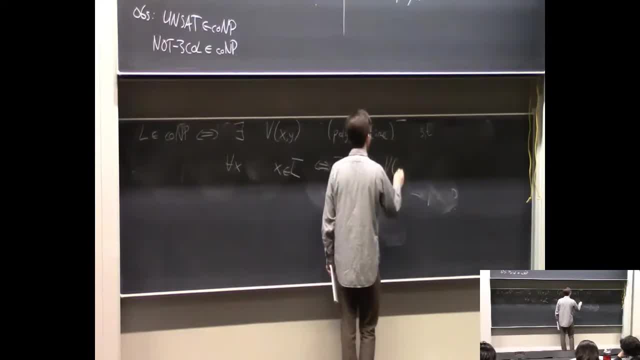 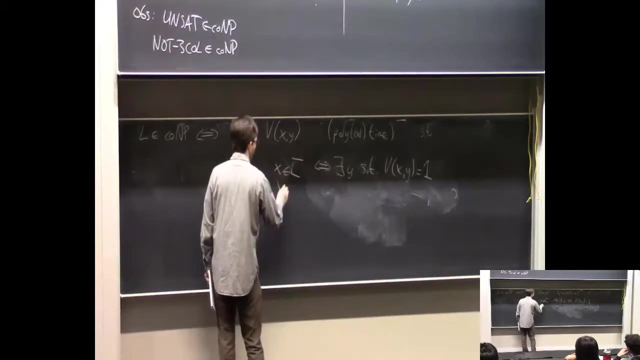 There exists a y, such that the verifier accepts. OK, I just took the verifier. I took the verifier definition of NP and replaced L with L bar. OK, And maybe I'll replace this too: x is in L bar with x, not in L. 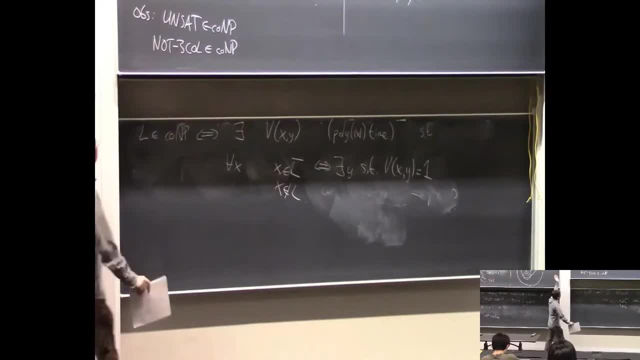 So if you just read this definition, a language is in co-NP, like tautologies is in co-NP. It's the case whenever you can certify to a verifier that a given input is not in the language, So like in the case of tautologies. 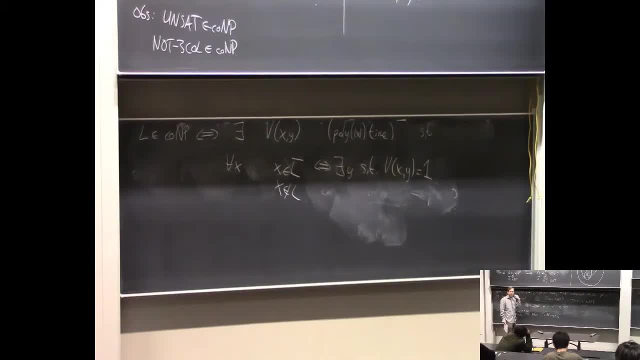 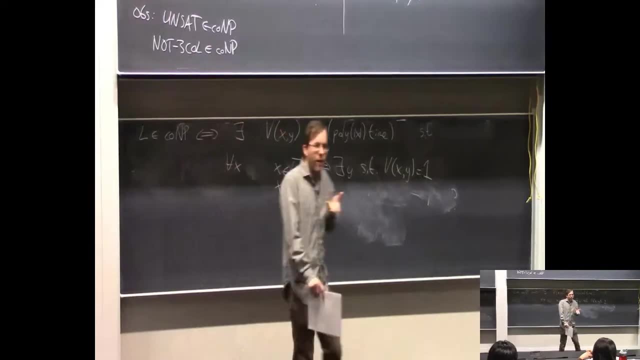 or the strings that are in the language. the languages are the ones that are universally true. We have this property right. When I give you a formula which is not universally true, you can sort of certify that to a verifier by giving a truth assignment where it's false. 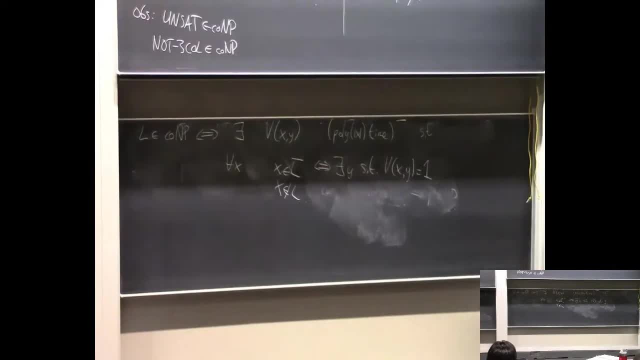 The verifier can check that. So I sometimes call. if I just had L here, this would be the definition of V as a verifier for L. So I sometimes call this. But I actually don't know how to do this. But I actually have negation or a complement of L here. 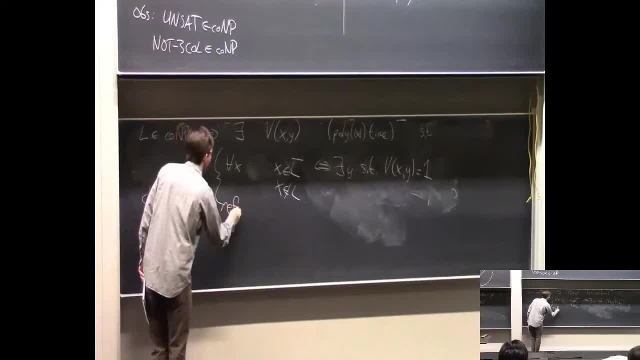 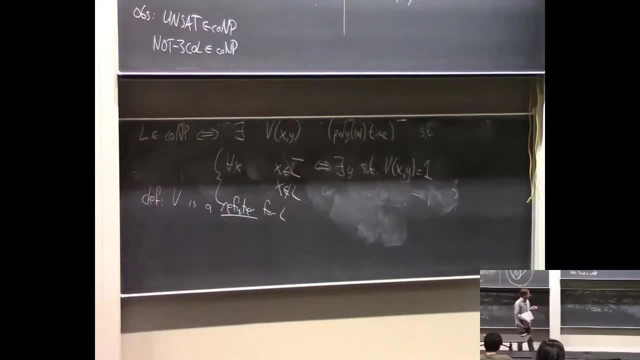 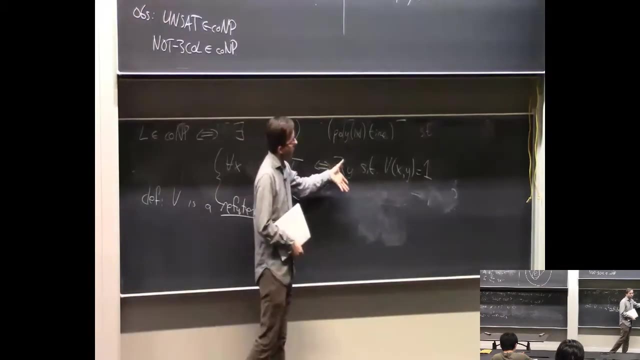 I sometimes call this V as a refuter for L. If somebody comes along and proposes to you a statement like x is not in L, then this refuting algorithm can certify that that's true. OK, So for example, this sort of proving way: 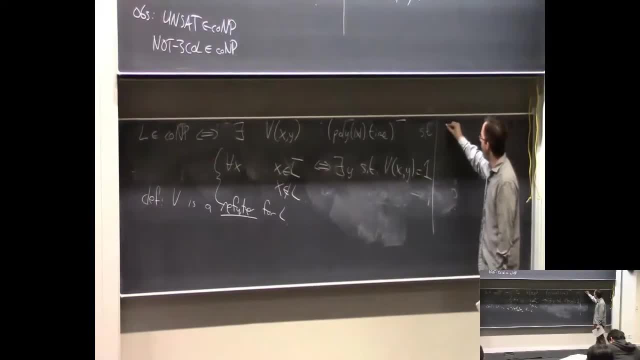 of thinking of things is useful for showing primes. The decision problem- I give you a number- is it prime? This is in co-NP. So one way of thinking about this is just syntactically You could say: well, primes is in co-NP. 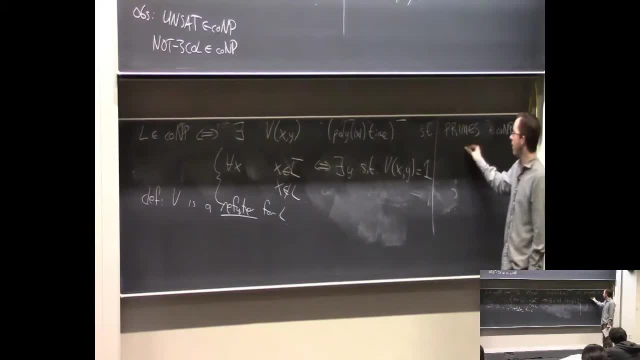 That's the same as saying the complement of primes, which is basically The composites. given a number, is it composite? is in NP, And this is a statement we've seen before Checking whether a number is composite. the problem is in NP because the verifier 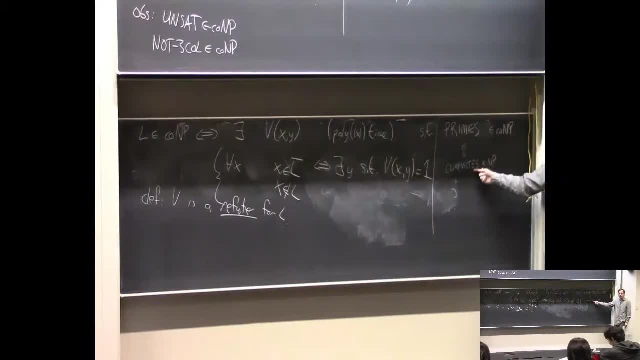 can expect to get a factor, a non-trivial factor of the number, and then it can check that it really is a factor of the number. So you can easily convince somebody who has polynomial time that a number is composite. So that shows that primes is in co-NP. 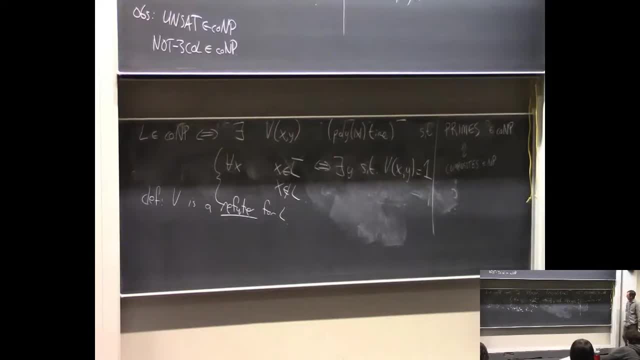 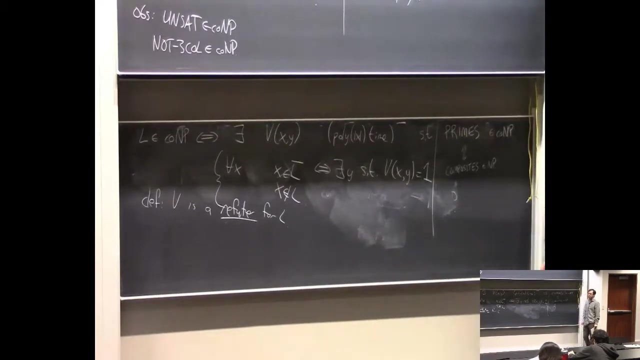 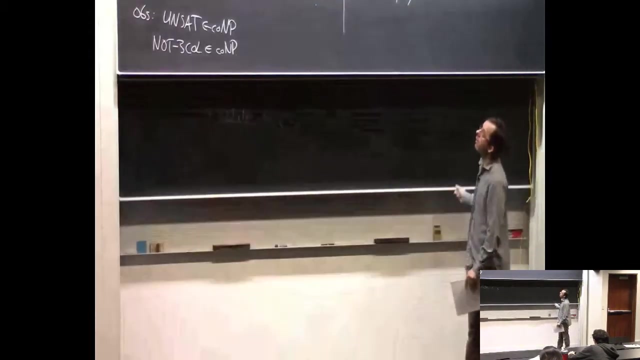 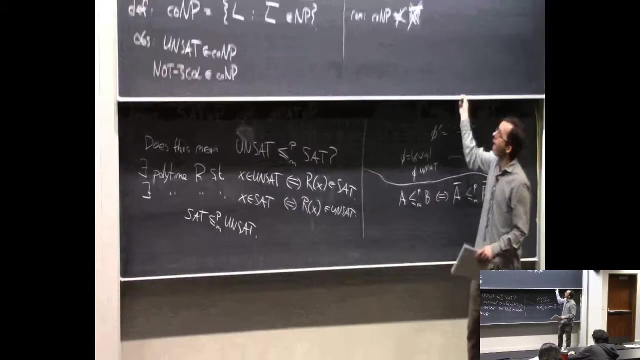 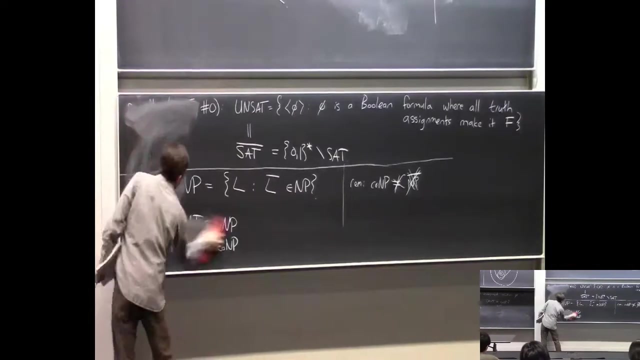 If you think about it This way, if somebody comes along and claims falsely, that a number is not prime, then you can become convinced of that fact. Any questions about this? OK, OK, So coming back to the idea that was at the beginning of the lecture, just to sort of summarize. 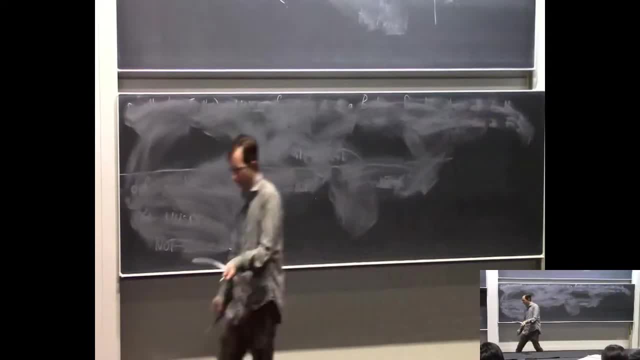 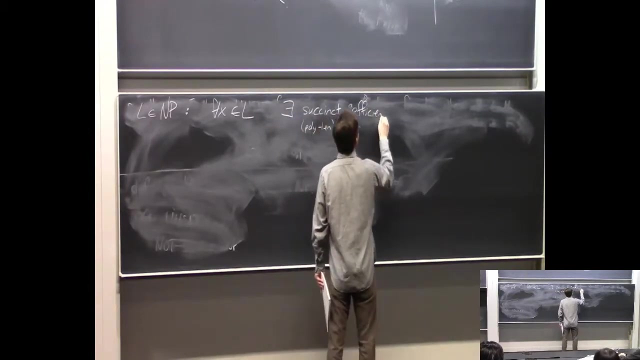 what we know. L is in NP. What this kind of means is that for all x that are in the language, there's like a succinct. this means poly length, efficiently checkable. this means poly time certificate. OK, OK. 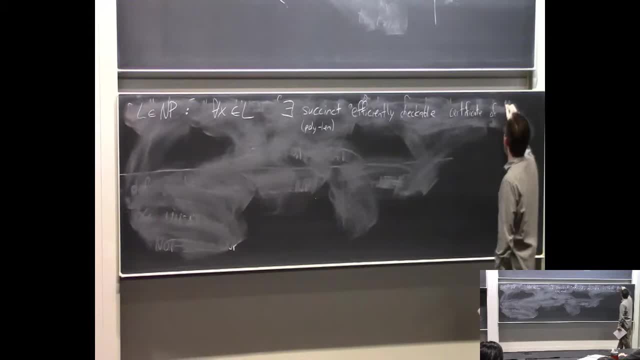 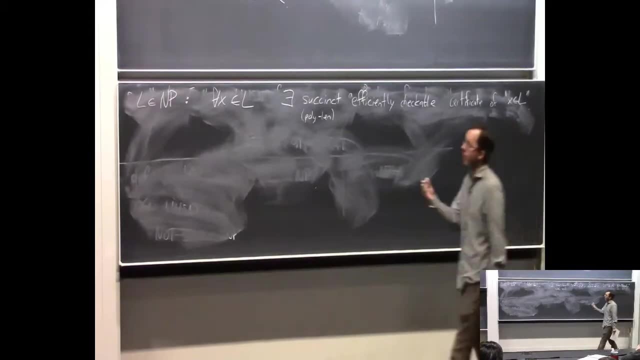 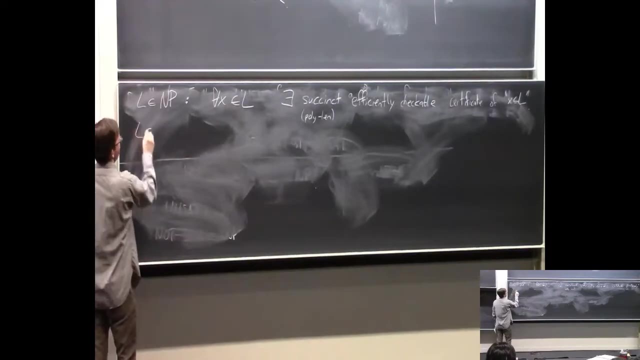 OK, OK, OK. Of the statement x is in the language Like: 3 colorability is in NP. For every graph that is 3 colorable. I can succinctly convince you that it's 3 colorable. I give you the 3 coloring. 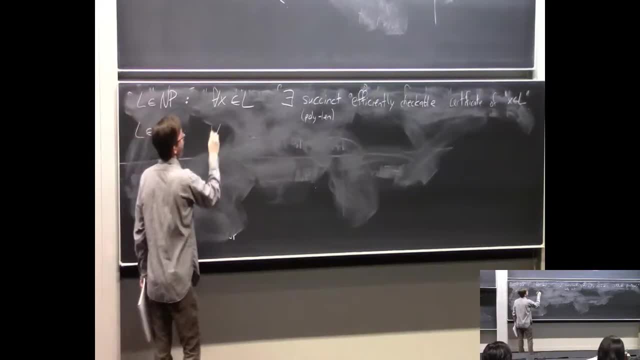 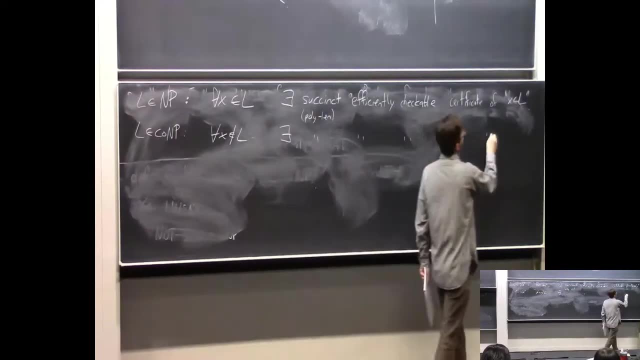 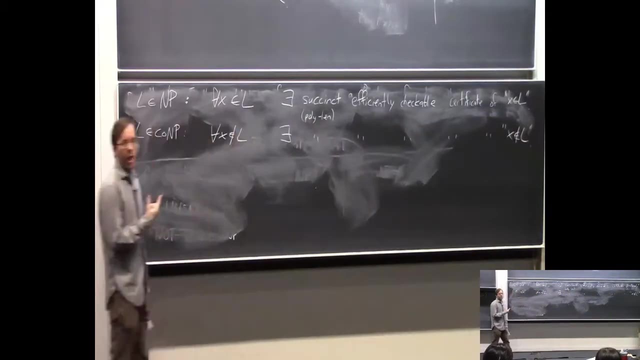 L is in co-NP is exactly. for all x's that are not in the language, there exists a succinct, efficiently checkable certificate of x not being in the language. OK, This is kind of like primes For everything that's not prime. I can efficiently kind of convince a verifier that it's not. 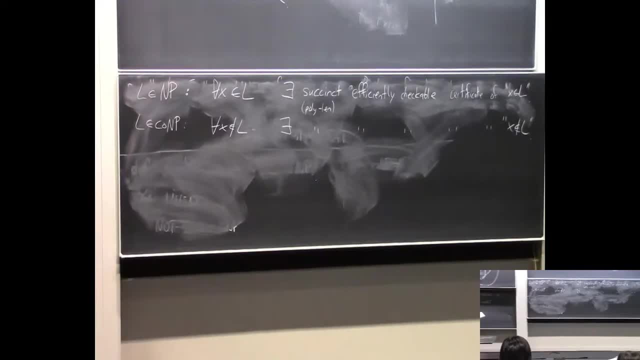 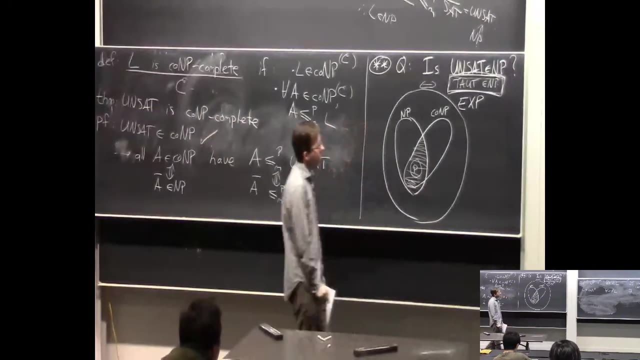 prime I give like a non-trivial factor. And what's very interesting now to think about, which is what we'll do for the last 25 minutes, is think about this, this part, right here, All the languages that are both in NP and co-NP. 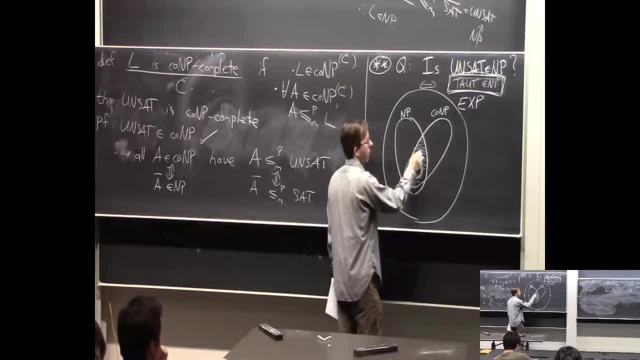 So we saw before that all the languages in P have this property. but there are other languages too that have this property. And what would that mean? Suppose L happens to be in NP and co-NP. I'll give you some examples that are not just hey, a language in P in a second. 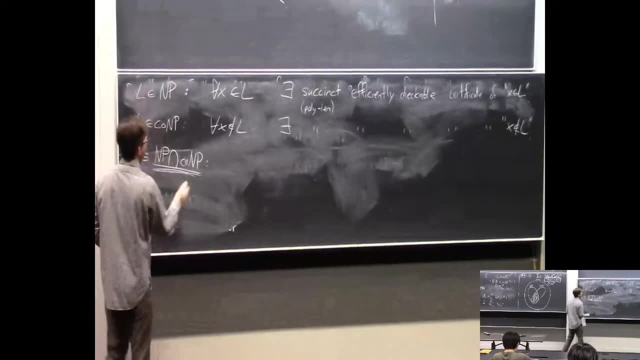 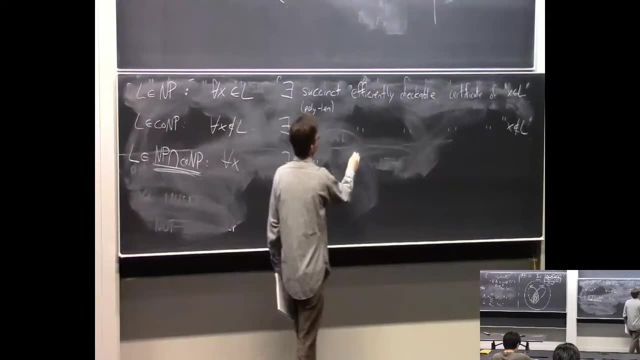 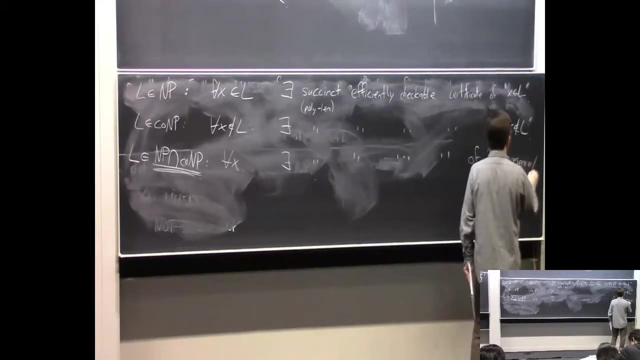 But this is a very interesting class. This is a set of languages. What this means is, if you call strings x, there is like a succinct, sufficiently checkable certificate of its presence absence in L either way. So if a language has this property, it's very interesting. 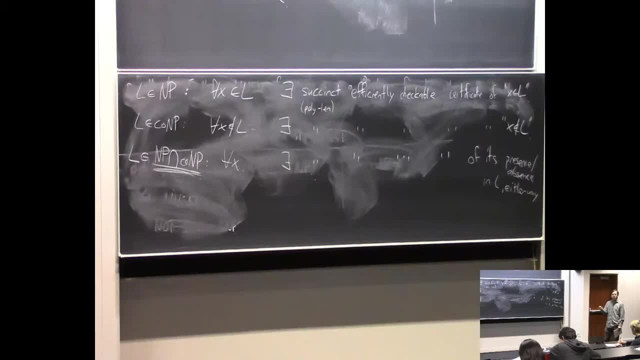 Like a language that has this property. Like somebody proposes a string and you may or may not be able to like efficiently in polynomial time, figure out whether or not the string is in the language, But if it is in the language, there's. 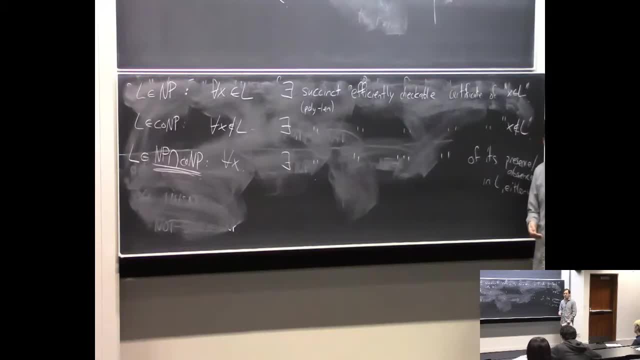 some proof that would make you say, oh yeah, I guess it is in the language. And if it's not in the language, there's also a proof that will make you say, oh yeah, I guess it isn't in the language. 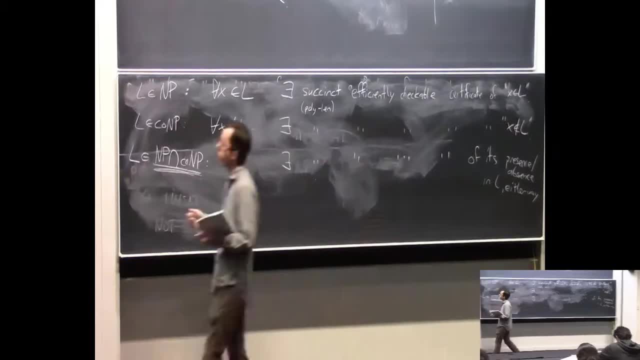 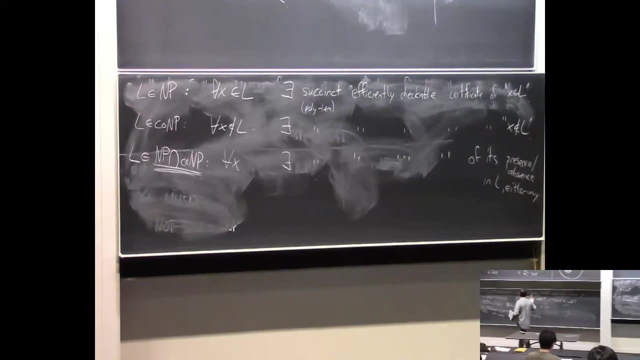 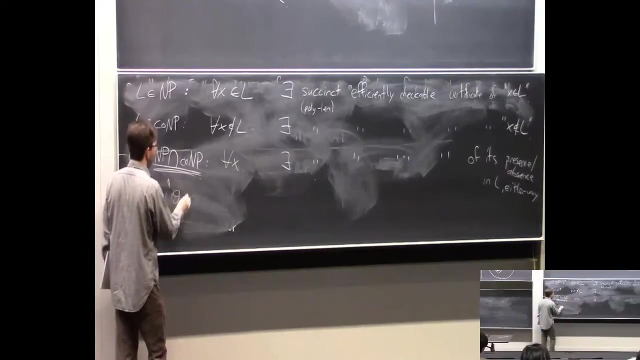 And let me try to give you some examples. So every well, you'll see some properties of interesting things about every language that's in both NP and co-NP. This is sometimes having some people the guy that invented P, Jack Edmonds, he called this. 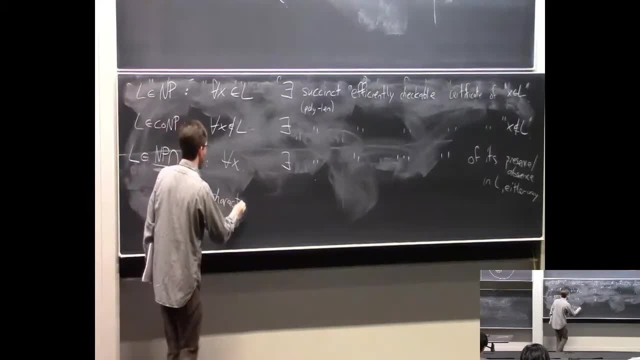 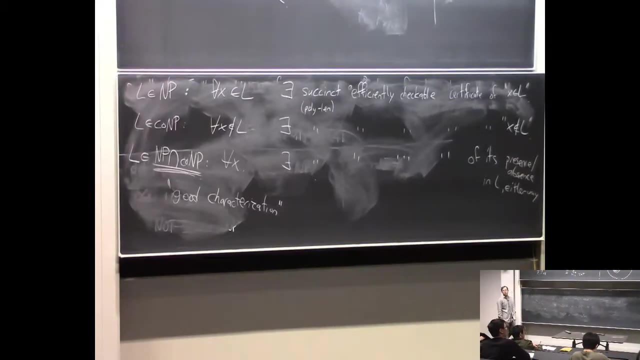 having a good characterization. It's kind of closely connected with mathematical theorems often So let me show some examples. Let me remind you of a problem from 251.. It's the problem of perfect matching. So long I'm going to start writing PM. 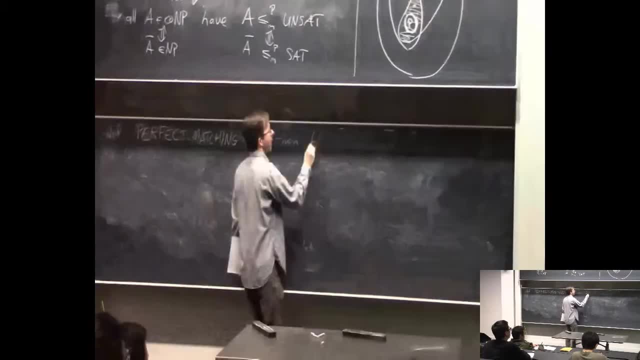 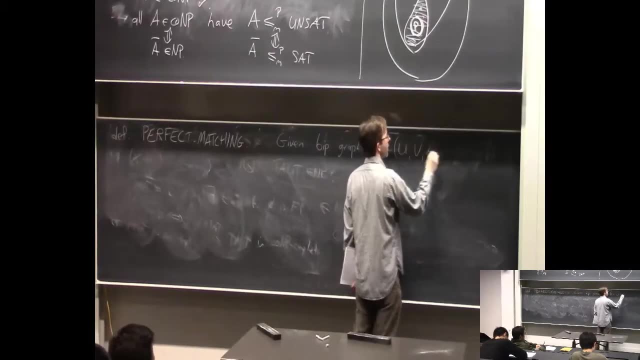 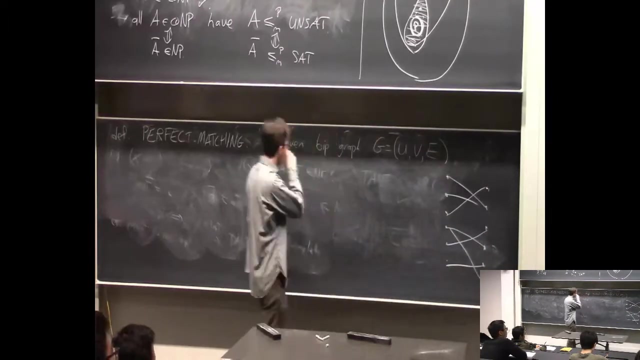 What is perfect matching problem? You're given a graph A, bipartite graph G, Left vertices U, Right vertices V And edges E, And you want to know yes or no. is there a perfect matching? 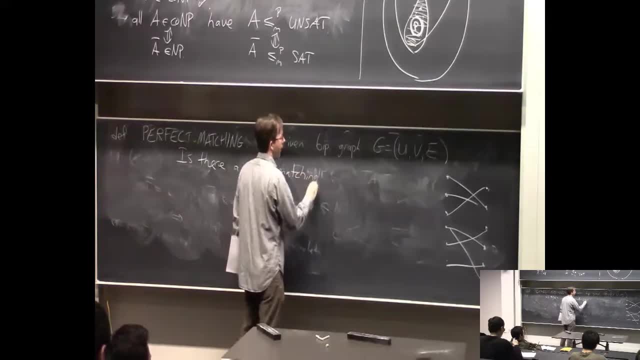 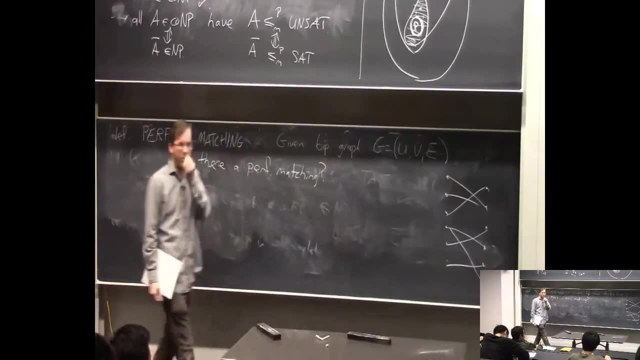 And I'll remind you, A perfect matching, right? It's a set of edges such that every vertex touches exactly one edge. OK, Given a bipartite graph, is there a perfect matching? It's not obvious how to solve this problem. 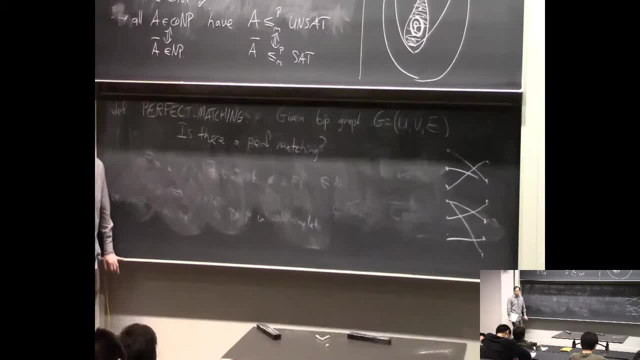 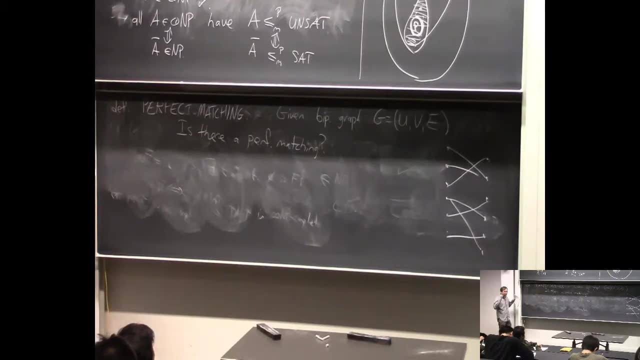 I mean, if you've never seen it before in polynomial time. One thing that is, like, once you know some complexity, a little bit obvious is that this problem is in, you know, in N? P. Can somebody say why that is? 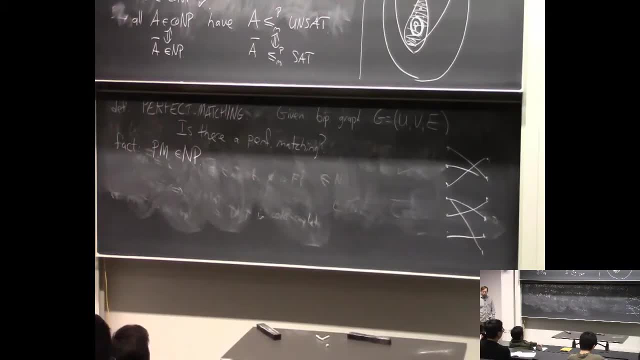 At a high level. Yeah, Yeah, You can kind of just like have a verifier that checks if the matching is perfect like a valid matching. Exactly, Yeah, It's easy to check If a candidate matching is indeed a perfect matching. 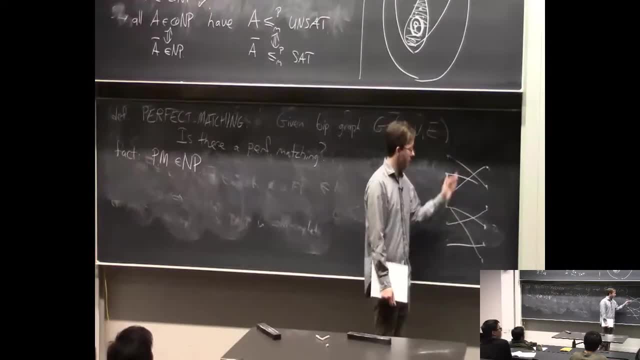 OK, so the verifier just expects a perfect matching and checks that. indeed, like every vertex, is covered exactly once. OK, so this is in N P. Now what I'm going to tell you is that it's also in co-N P, And this requires a math theorem. 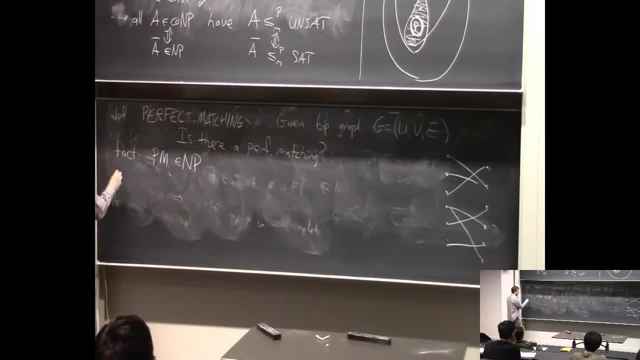 that you may or may not have learned in your life, which is called Hall's theorem. Normally I don't like to do this, but put up your hand if you've heard of Hall's theorem but maybe you forget what it is. OK, only so-so. 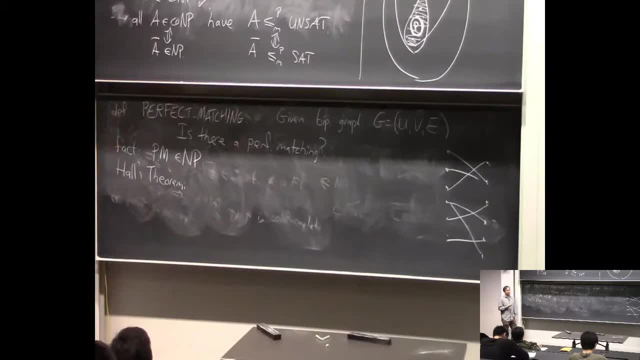 So I'll tell you what this is. This is like a classic theorem you would learn in like a college combinatorics class. I don't know what the what is the combinatorics class here in the math department Three something? 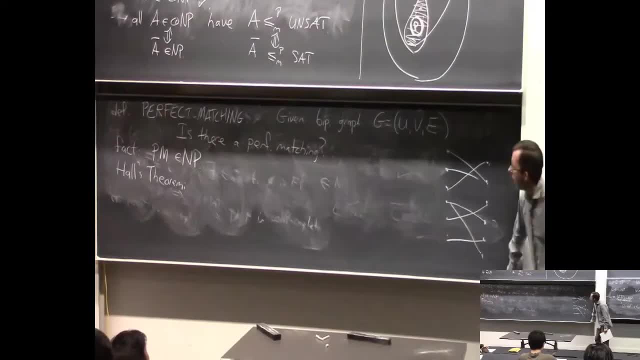 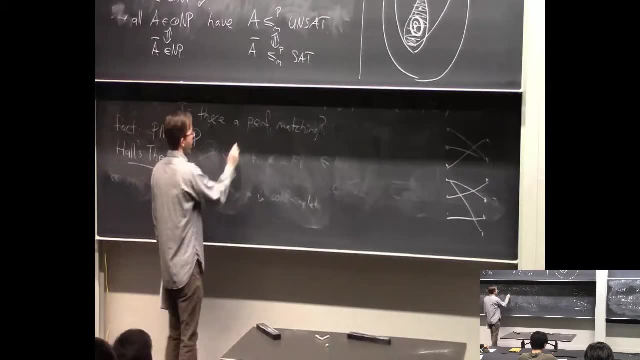 Yeah, I'm sure you learned Hall's theorem in that class. So Hall's theorem is based on the following observation: OK, So this is just like a classic Classic math combinatorics theorem. Suppose you had some. this is just some statements here. 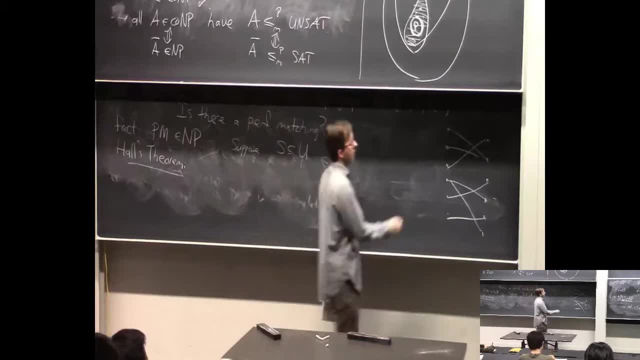 Suppose S was a subset of the left vertices, like maybe these two, hypothetically, And suppose you looked at what's called N of S, the neighborhood of S, That's all the vertices on the right which have an edge into S. Actually, 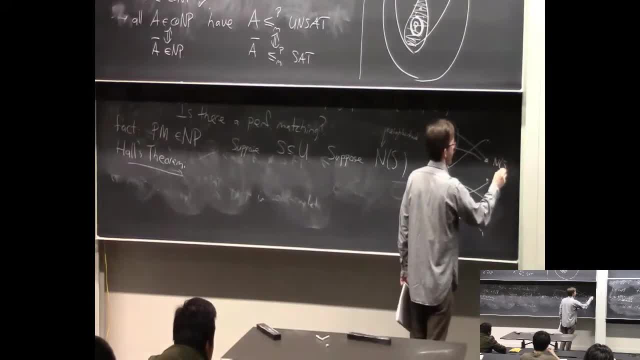 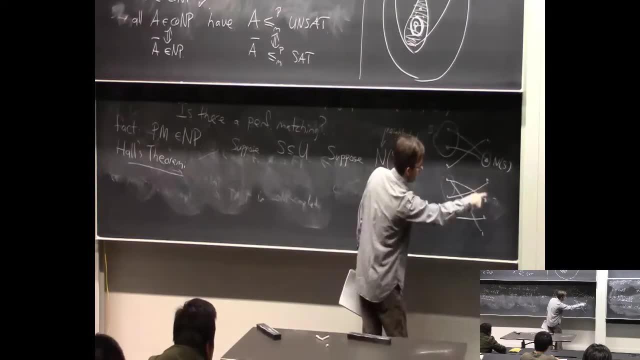 in this case it's quite small, It's just N of S is this single vertex, Whereas conversely, like if this were S, then N of S would be this guy, this guy and this guy. So we say: this is S prime. 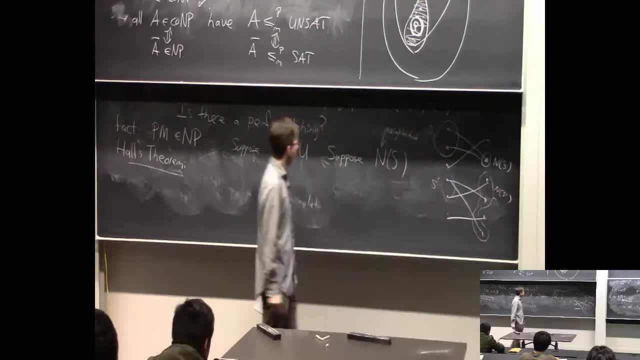 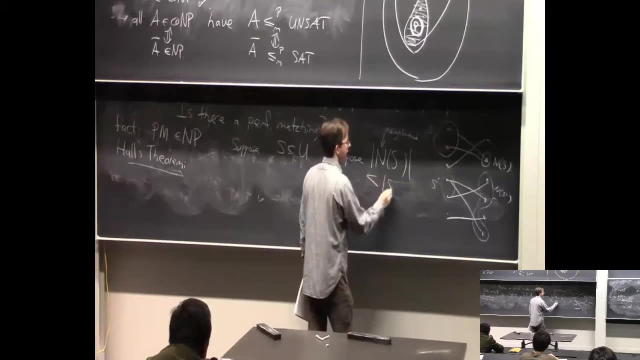 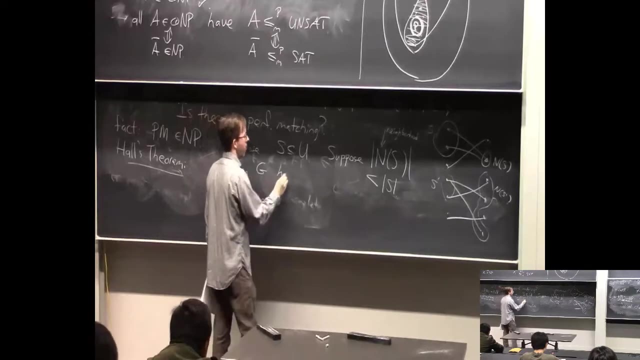 This would be the neighborhood of S prime. Now suppose the neighborhood of S had strictly fewer vertices than S, Then G has no perfect matching. This is not Hall's theorem. This is like a pretty easy fact. 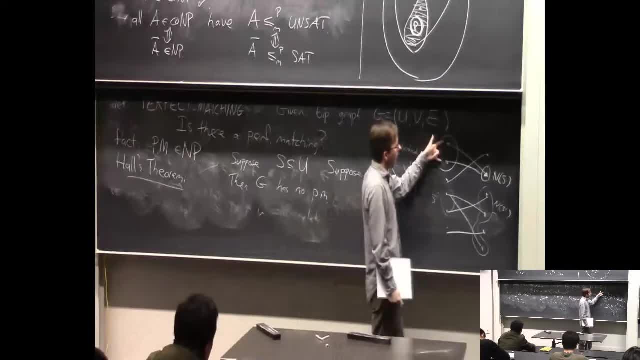 If somehow you have some vertices over here that if you look at how many edges they could go to, it was less than the number of vertices, then there's no way the graph could have a perfect matching right, Because you could not connect each vertex, even in S. 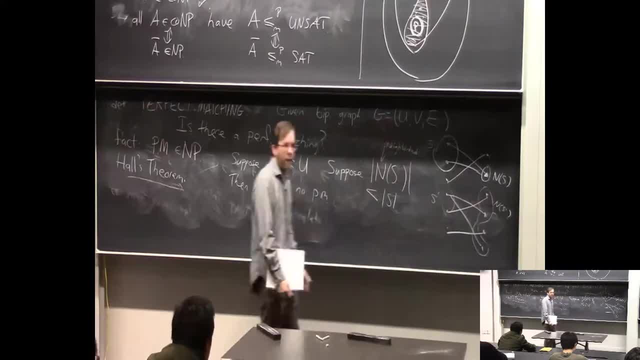 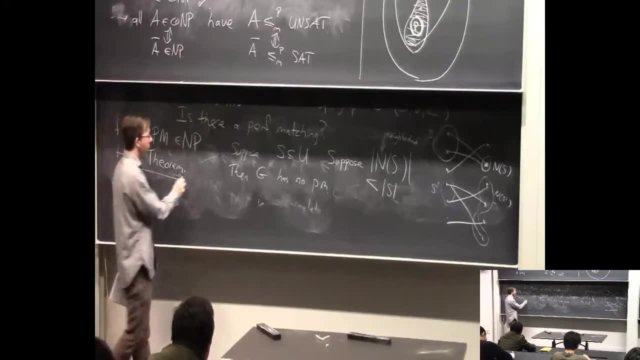 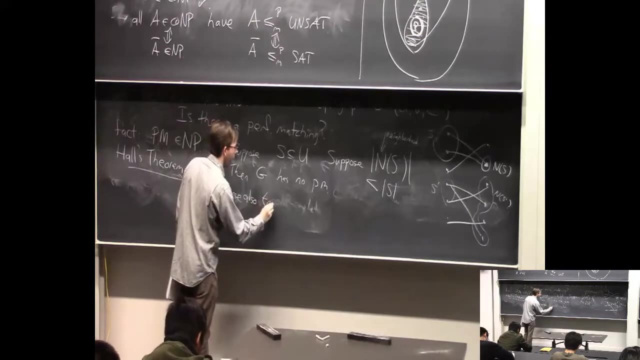 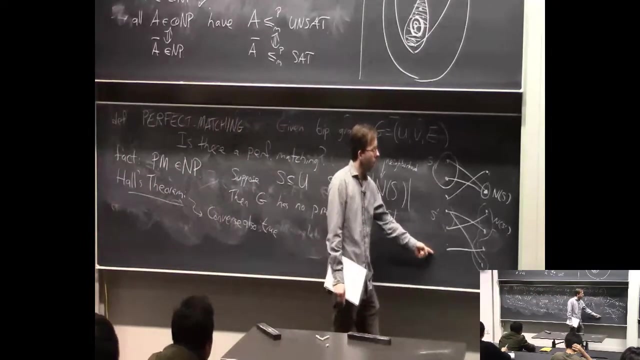 to all different vertices on the right side. Does that make sense? The Hall's theorem is: the converse is also true. It's just to say, if every set of vertices on the left S has, the number of neighbors of S is at least the size of S. 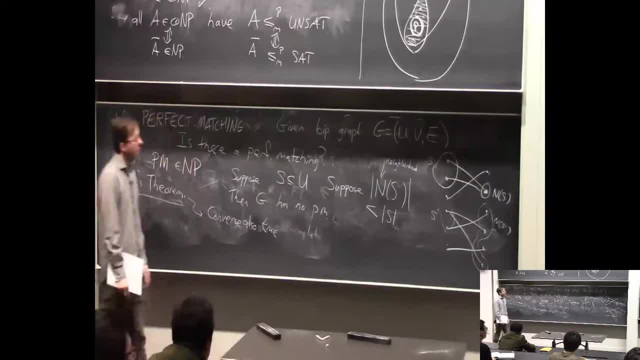 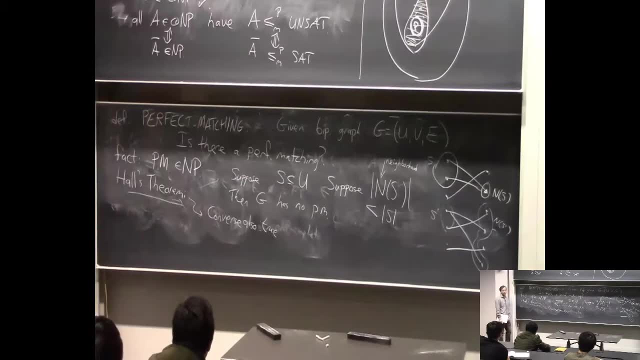 then there is a perfect matching. That's not obvious. It takes like a one-page proof or like a 30-minute proof in a combinatorics class, But it's a famous theorem in combinatorics. Another way to say that is: I mean. 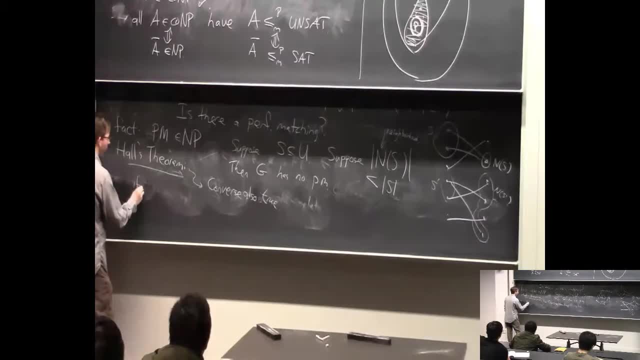 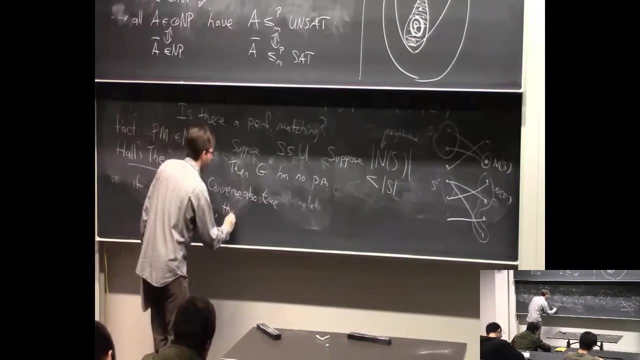 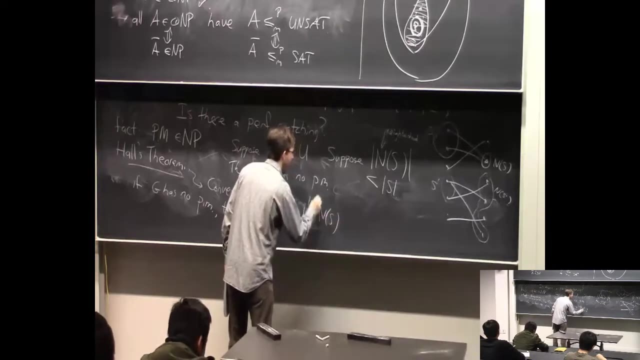 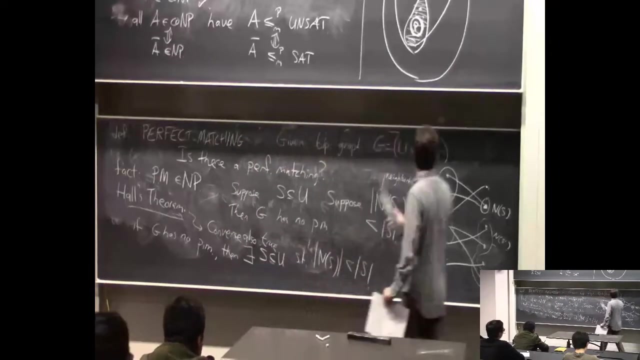 to take. the contrapositive is: if g has no perfect matching, then there exists an s which is a subset of u, such that the number of neighbors of s is strictly less than the number of vertices in s. So this fact is another way to say Hall's theorem. 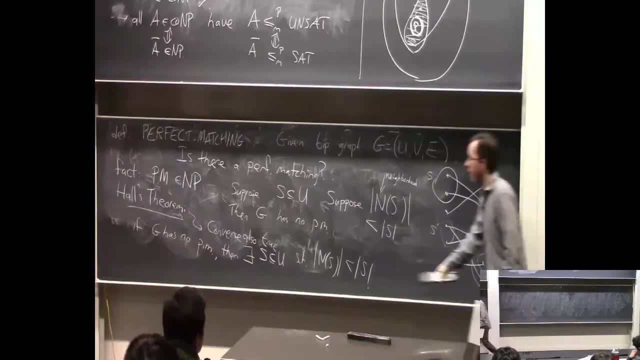 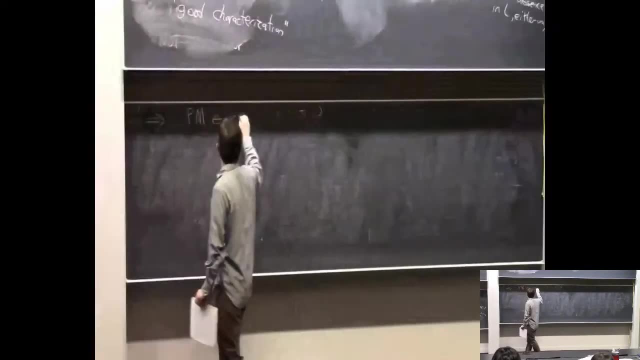 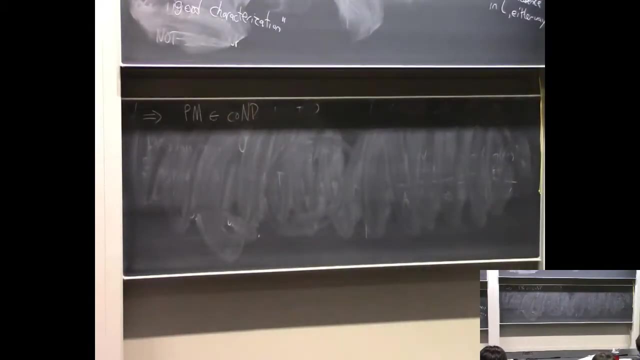 So actually, if you've taken a combinatorics class and you learned Hall's theorem, then I could say that Claim this pretty easily implies that the perfect matching problem is in co-NP. So why is that? Can somebody say Yeah? 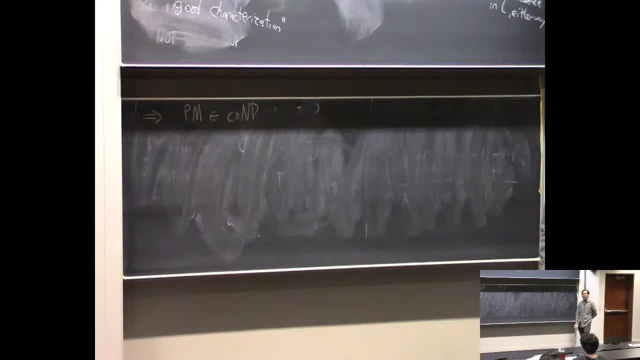 Could you just check to see the number of neighbors strictly Well, you don't have time to go over all subsets s and check whether the neighborhood is of size bigger than s. It's not hard, Given a percentage. I mean you could use a particular s. 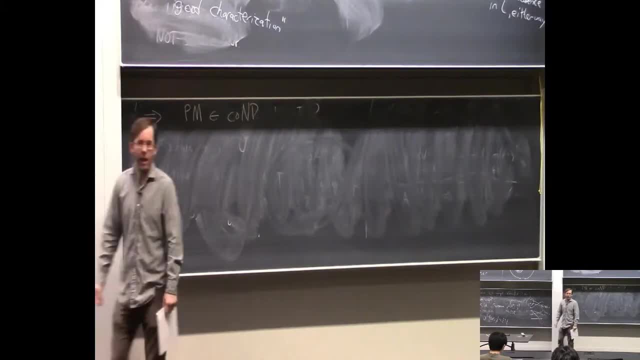 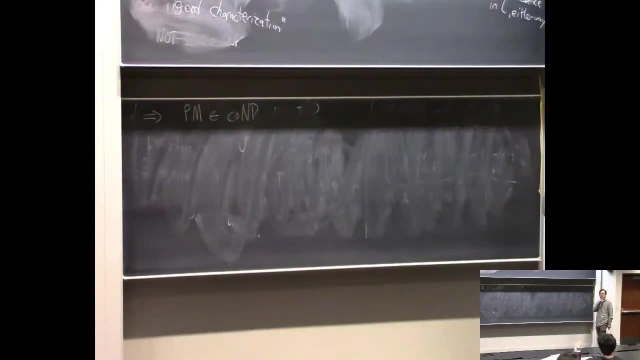 to check whether this condition holds, But there's exponentially many different s's. But you're almost there. The fact that you can check it for a particular s is the key. Yeah, You'd use a subset as a certificate. That's right. 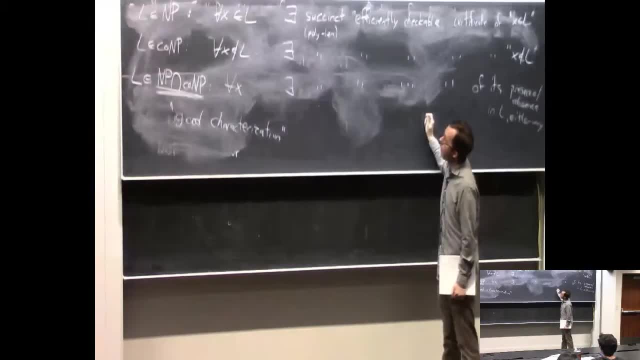 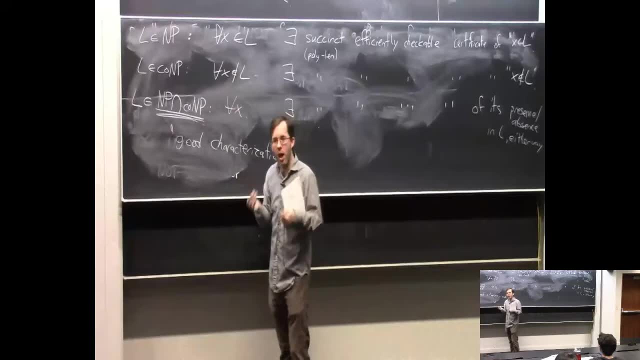 So in the way that, like I mean, if you think about it this way, to show that perfect matching is in co-NP, you want to show that whenever you have an input, a bipartite graph, which is not in the language, 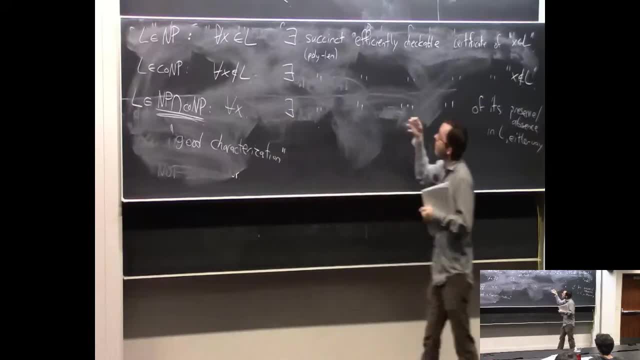 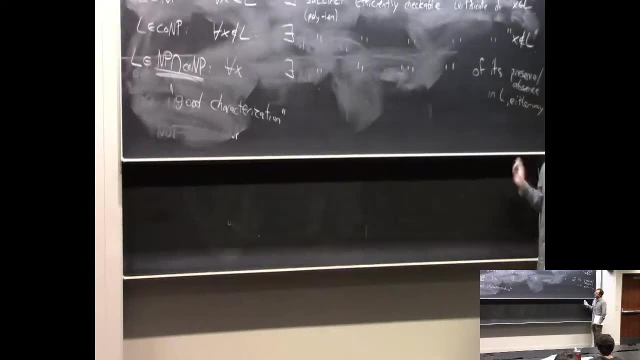 which doesn't have a perfect matching. there's some efficient, succinct way to prove it, like there's a verifier which, when given appropriate proof, will check that fact. Or you can just even think about it as just no perfect matching, as in NP. 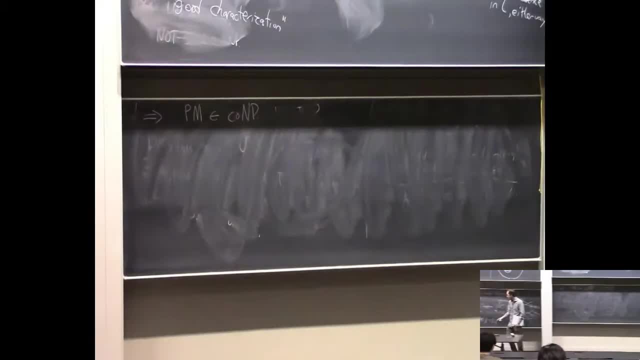 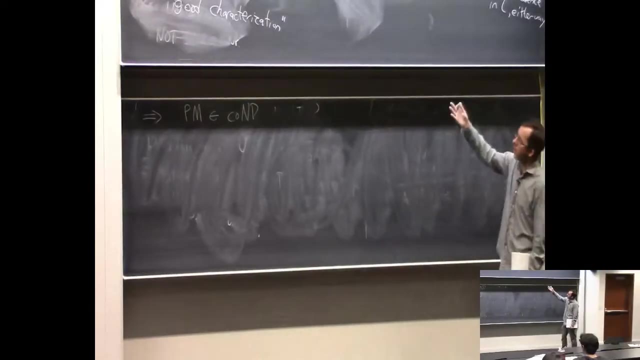 And Hall's theorem gives it to you. The certificate can be the set s which exists by Hall's theorem, And the verifier just has to check that the neighborhood of s has size smaller than the size of s. So that's why it's sometimes called a good characterization. 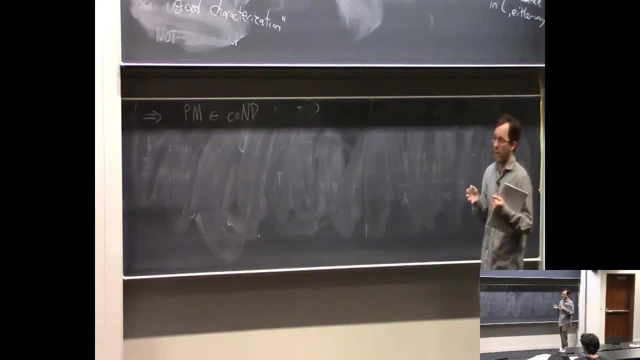 like, if the graph has a perfect matching, then you just here's the perfect matching. If the graph doesn't have a perfect matching, then you just here's the set s on the left whose neighborhood size is smaller than the size of s. 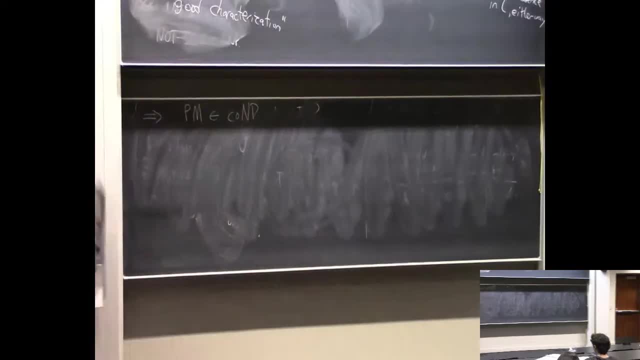 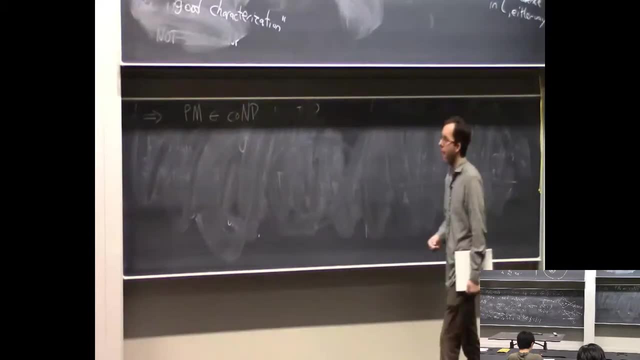 And each of these is easily certifiable. The tricky part is proving Hall's theorem, but once you know that, then you're in good shape. Yeah, So this perfect matching is in P Right. So what we've shown so far? 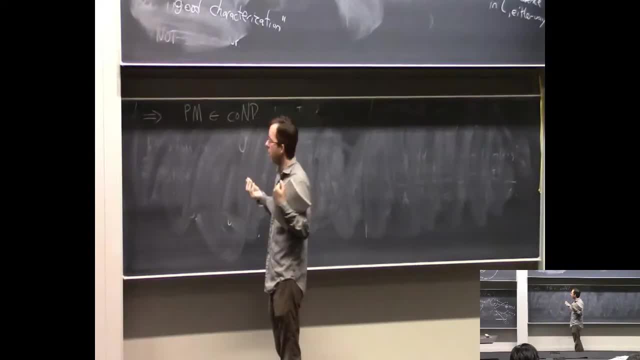 So if you know if you're really hot on combinatorics, then you're like: oh yes, it's OK For anybody, it should be in this class. it should be pretty straightforward that perfect matching is in NP. And if you're really hot on combinatorics, 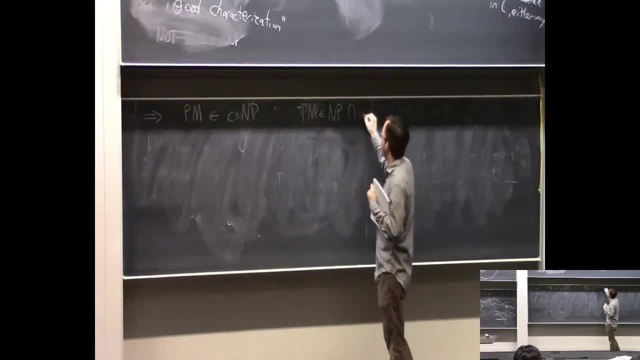 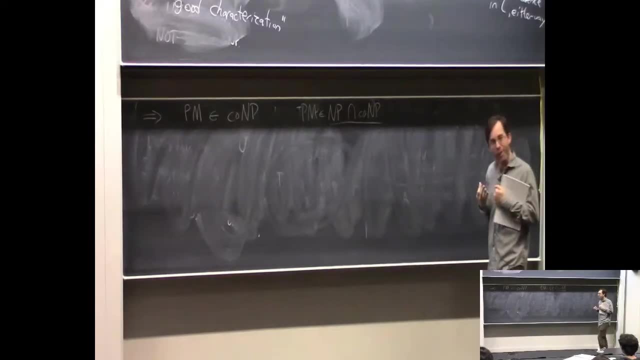 and you know Hall's theorem like the back of your hand. then you're like: oh well, it's quite clear that it's also in co-NP. So it's in this class: NP, intersect, co-NP. Now, actually, if you're also really good at algorithms, 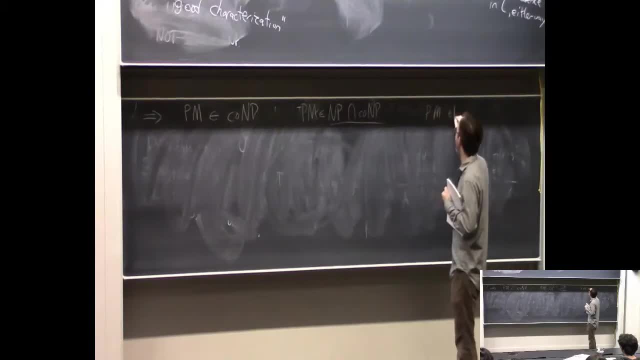 you happen to know that perfect matching is in P, So I kind of wanted to tell you an example, if I could, of a language. maybe here perfect matching- Well, actually perfect matching- was in P, But it's not obvious, right? 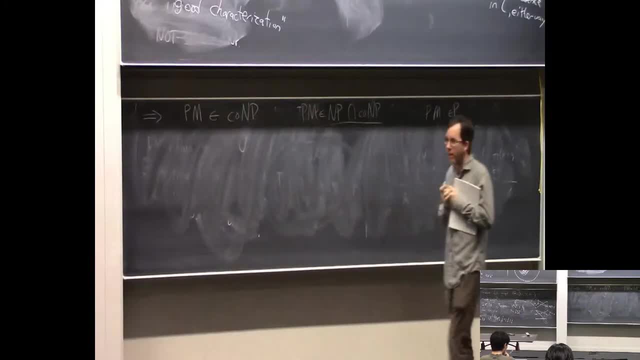 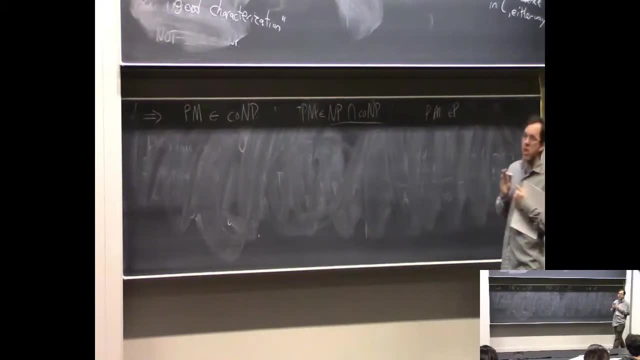 I mean the algorithm for determining if a graph is a perfect matching is not especially easy. You know there's the augmenting paths and everything, So it takes some thought. But this is a very interesting historical phenomenon where people have an interesting algorithmic task. 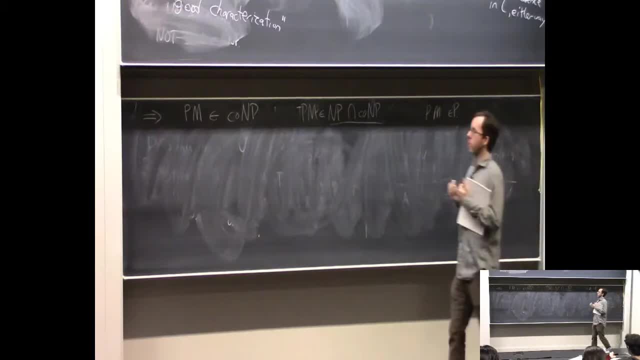 like perfect matching and then they'll first prove potentially that it's in NP and also in co-NP, And then, much later, they'll prove that it's actually in P. So we won't talk about it in this class. 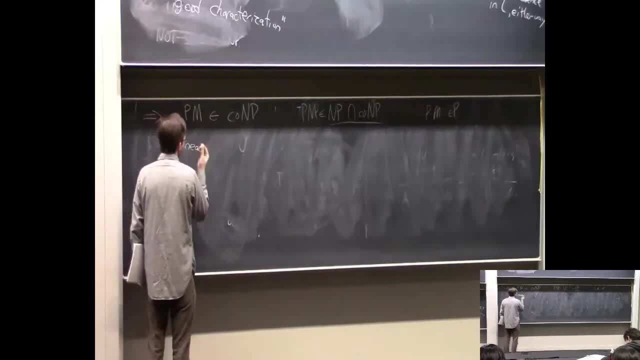 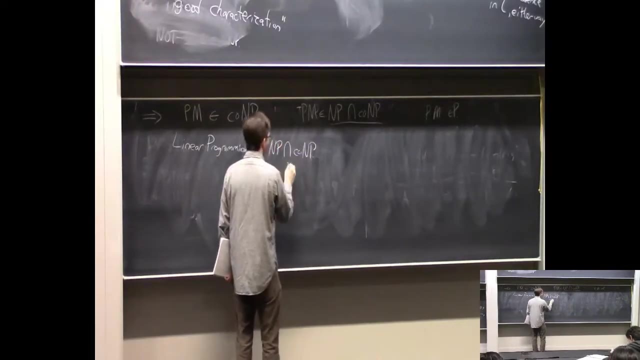 but probably one of the most important algorithmic problems in computer science is called linear programming. Hopefully you'll learn about it, maybe in 451 or something, And in a sense people proved that this was in NP and co-NP in like 1948 or something. 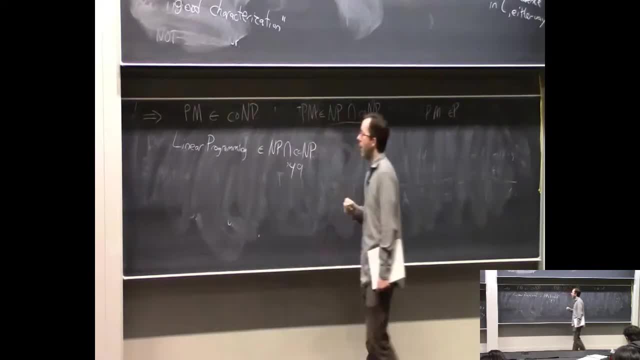 Yeah, So it's in NP And it's in co-NP in 409.. So, whatever this problem is, it's basically whether or not a system of linear inequalities has a solution or not. You know about linear equalities having a solution or not. 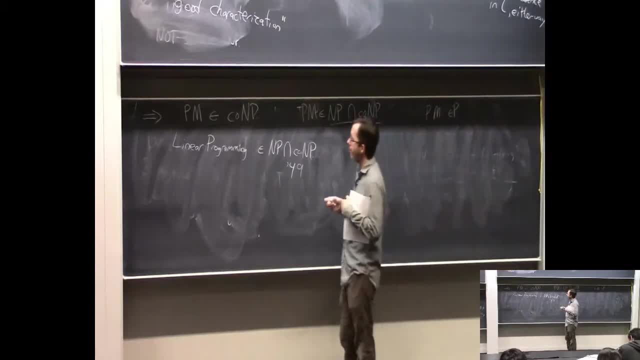 You can solve that efficiently. But whether linear inequalities have a solution or not, it's a good question. It's in NP because you can just show a solution. It's in co-NP for some other reason. that people figured out is also in P, And they proved that in 1979, so 30 years later. 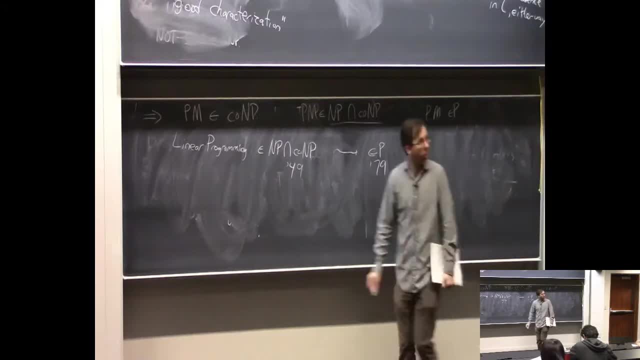 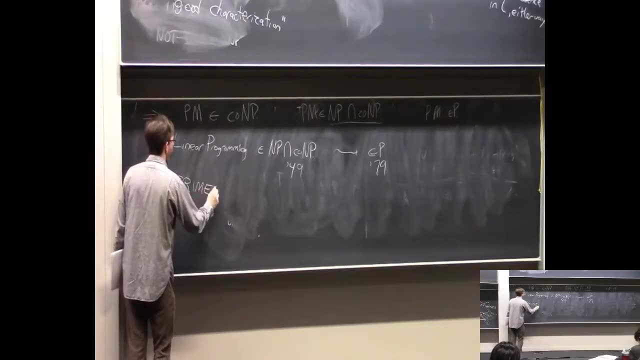 And there's another example of that which I guess we'll talk about right now: Primes. That's one of the most famous problems of all in algorithms. I give you a number: Is it prime or not? So this problem primes. 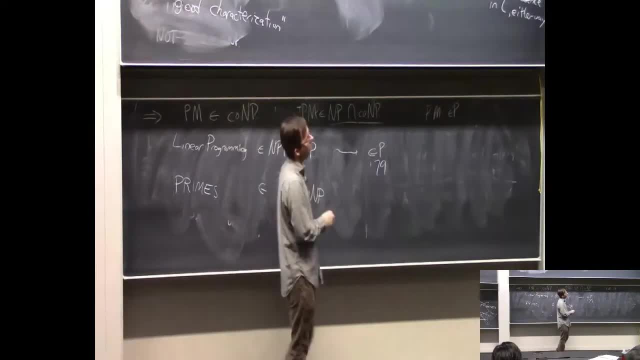 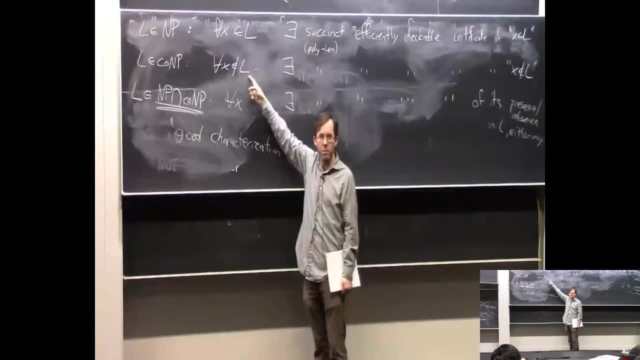 It's in co-NP. That's not hard. If I give you an input, a number which is not in the language of primes, it's easy to certify that It means it's a composite number or it's 1 or 0.. 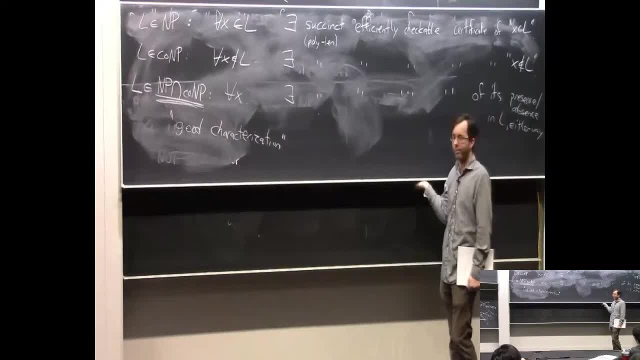 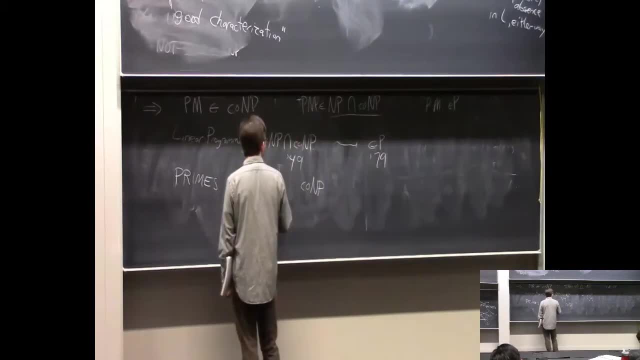 So you can just show a factor of it And the verifier can check that that's a factor. So in 1975.. It was shown to be in NP by a person called Pratt. So just think about that for a second. 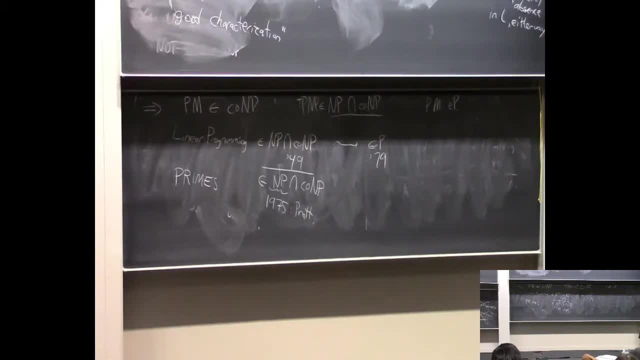 Pratt figured out a way. If I give you a super long number- and again this is like a problem where the input is a number, So you should think of n as the number of digits. So you get some 10,000 digit number and somebody comes along. 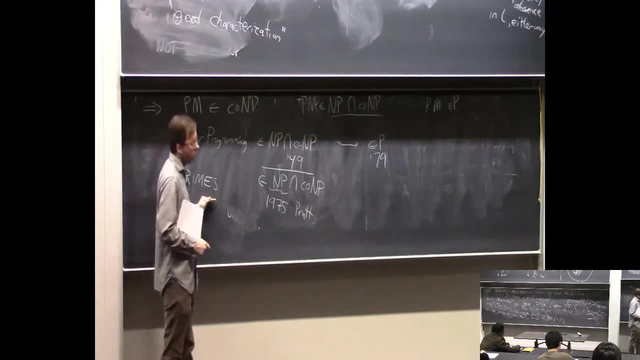 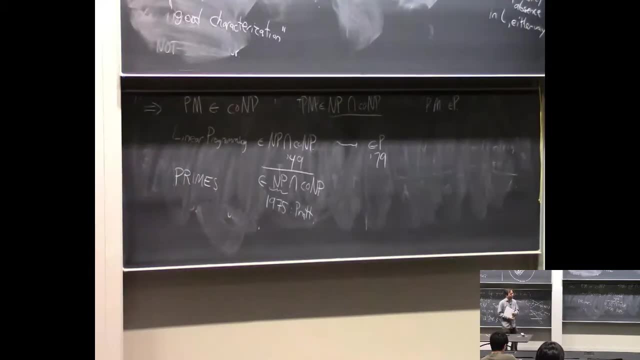 and says: I swear that this is prime. I swear it's in the language. Pratt showed a way like a system whereby you could efficiently verify that If somebody gave you an appropriate certificate of primality, whatever that could mean, it's checkable. 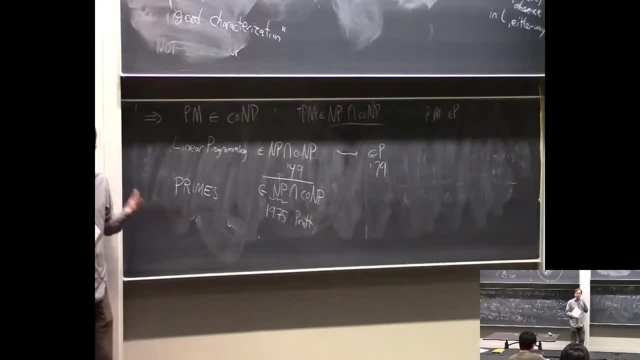 And this is a case where a language being in NP is super, not obvious. I mean, how can I quickly certify to you that some 2,000 digit number is prime? It doesn't look so easy, right? I can't just say: I swear it's prime. 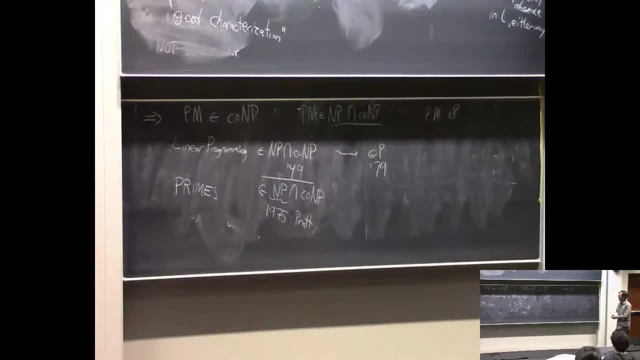 And you're like, I need it, I need a little more than that. And you could say, well, 2 does not divide it. I mean, yeah, it's not clear, But he did it and it uses much like Hall's theorem needed. 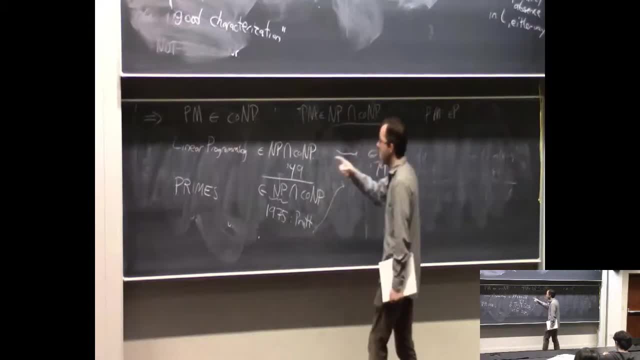 like a little theorem in math or some theorem in math. This thing about linear programming uses another math result about convex sets called Farkas. Lemma Pratt uses like some theorem about number theory And it's the kind of theorem that you could have. 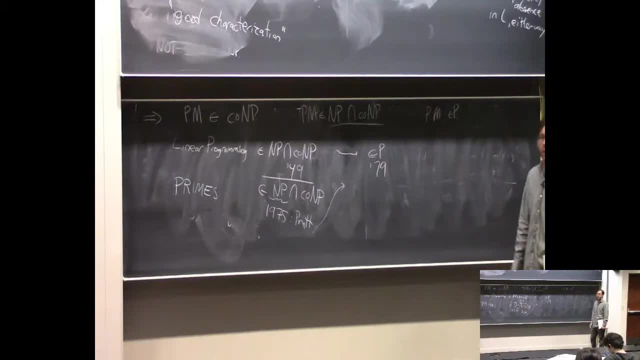 proved at the end of 251.. It's not very advanced number theory. It's about cyclic groups- Maybe you talked about groups or maybe not- in 251, and repeated squaring like exponentiation, mod of prime and all that stuff. 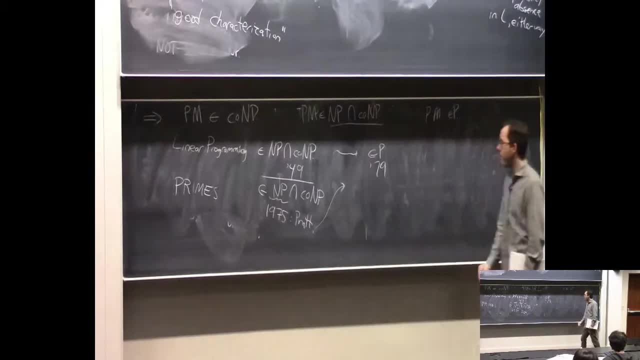 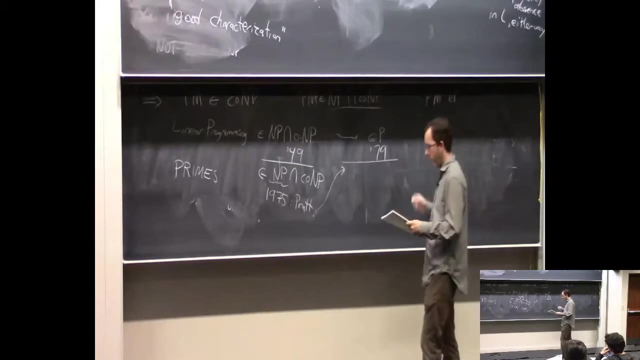 So I'll even tell you a little bit about it, but not all of it. So if I had like half an hour, I could prove this to you: that primes is in NP. I don't have half an hour, But let me give you some idea. 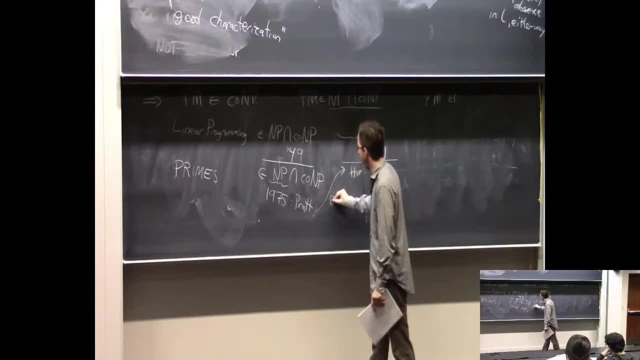 Here's a theorem that's like a 251 level theorem, if you remember all that stuff. So a number b is prime if, and only if, there exists a number a, let's say between 1 and b, such that a, a squared, a cubed. 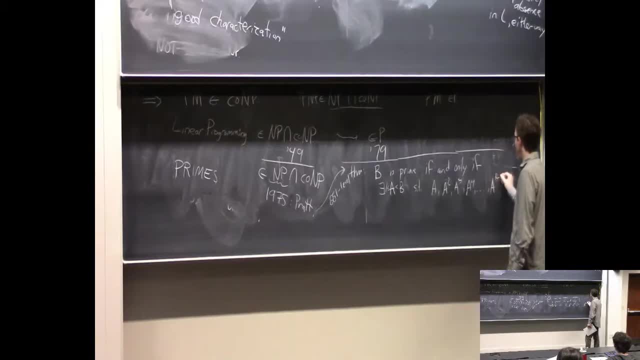 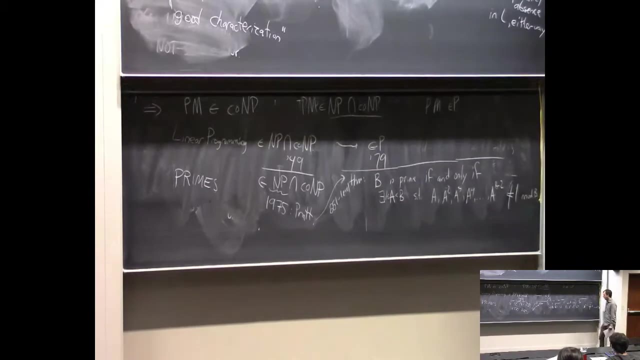 a to the fourth, all the way up to a to the b minus 2, are not equal to 1 mod b. That's a fact. You put together all the number theory that you learn in 251, with enough help, you could prove this. 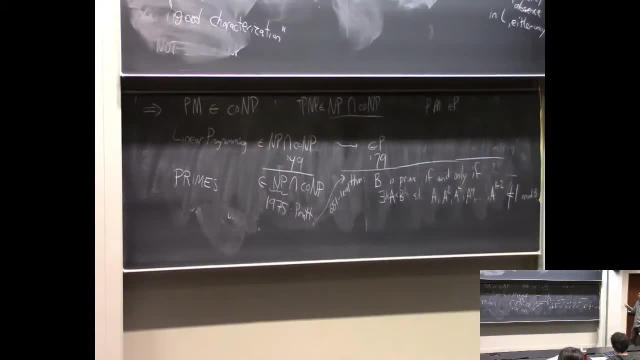 That's a fact. This fact is not enough to prove that it's primes is in NP. But I don't have half an hour so I can't do that. But I hope it'll slightly, and I'll explain why in a second. 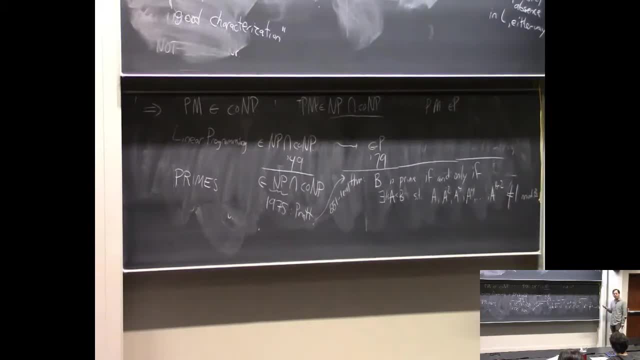 I hope it'll slightly give you the flavor of how you might start to imagine that it's possible that primes is in NP. So the trouble with directly trying to show that primes is in NP, it's like I have to convince you that a statement of the form. 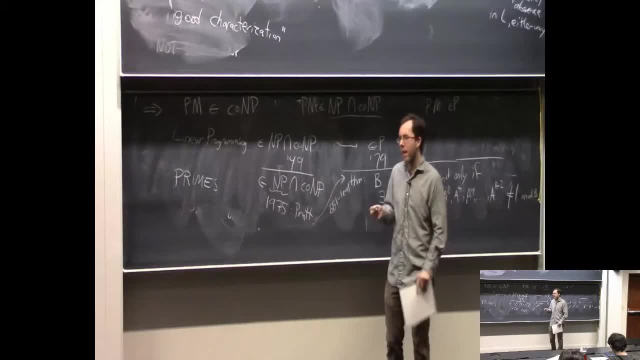 for all something is true. Primes is like really saying to say that b, b is prime is to say that for all numbers less than b they don't divide into b evenly. So if I'm the prover I can say: well, look, 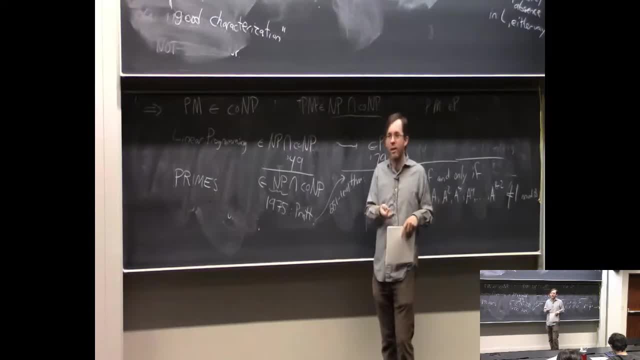 2 doesn't divide into b and 7 doesn't divide into b and 10 doesn't divide into b. But to be convinced that b is a prime, you really have to know that all the numbers less than b don't divide into b. 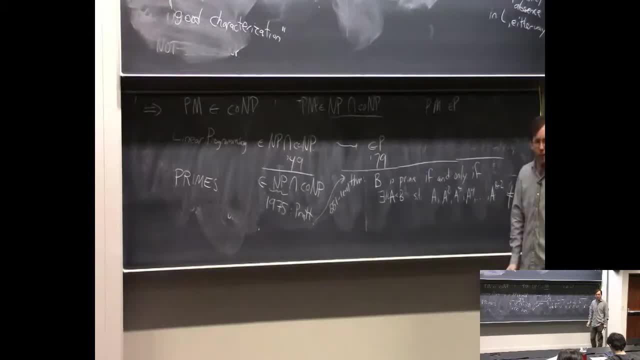 And it's hard for me to prove that. It's hard to prove a for all statement, as you know from life, But this theorem is quite nice because it's telling you that there's sort of a definition or like an equivalent statement about primality. 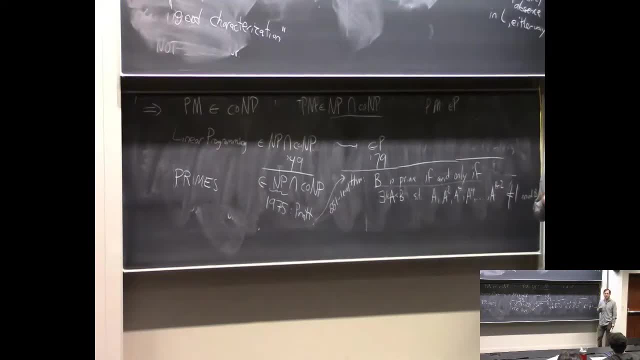 that's there exists kind of statement. So b is prime if there exists a number a such that some arithmetic stuff holds And that can put a smile on your face if you're trying to show that primes is in NP, Because you can imagine the prover saying: 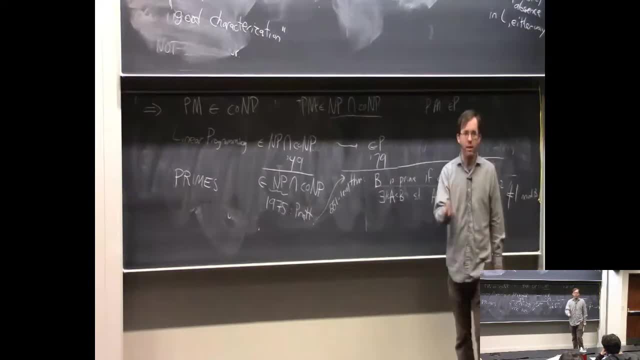 hey, you were curious what this magic a is. I'll just tell it to you. The prover can send this a. It's part of the certificate for the verifier to check Now. unfortunately it's not enough, Because for any of these statements, 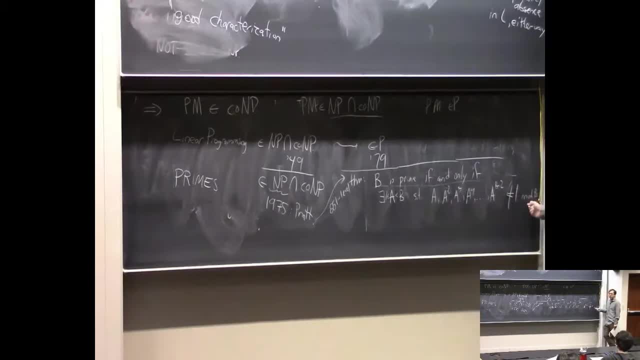 like whether a to the power of 4 is different from 1 mod b. you can check whether or not that's true in polynomial time, But in this theorem to really check that this a does the job, you'd have to check all of these statements. 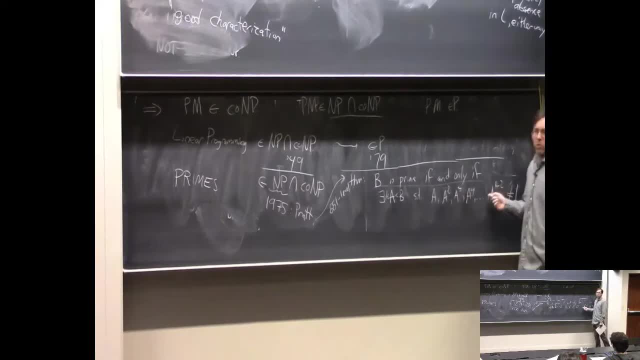 if you're the verifier And there are b minus 1 of them, And b is not like the length of the input, b is like the actual input, Which is like some 1,000 digit number, So you can only in exponential time. 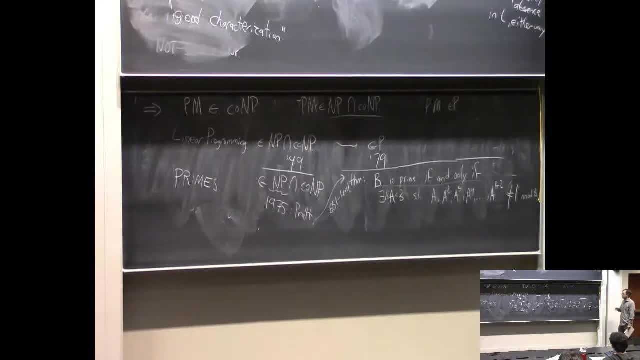 check all these statements, But Prath adds a few more ideas on top of this and turns it into a proof, So maybe I'll put on some stuff about it on Piazza, But at least maybe this helps us show the start of the idea. 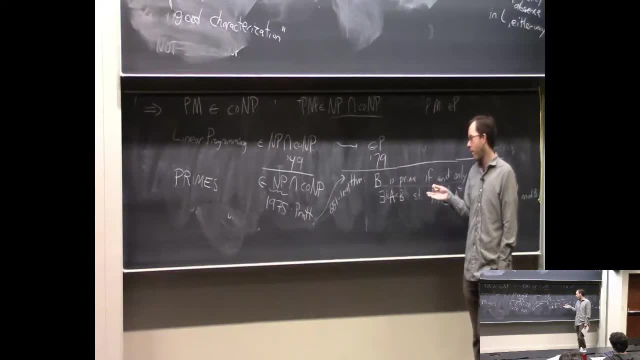 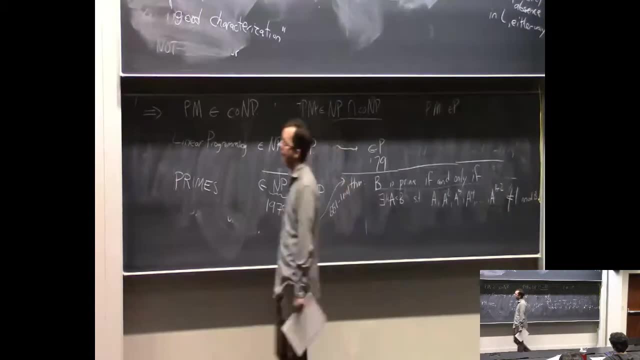 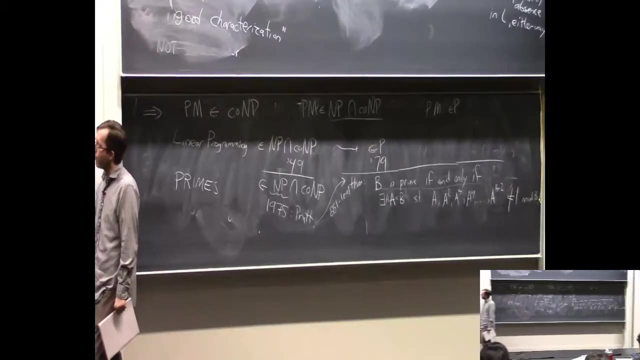 that we've converted a definition of being prime from a for all kind of statement to a there exists kind of statement. Just like in the perfect matching case, we showed that the problem of no perfect matching, given a graph that doesn't have no perfect matchings, is in NP. 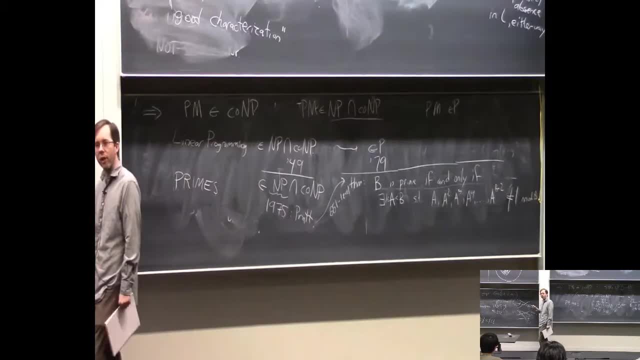 To have no perfect matchings is also like a for all statement. It's like saying for all candidate matchings: they're not perfect, But like Hall's theorem tells you, oh, it's actually equivalent to a there exists kind of statement. 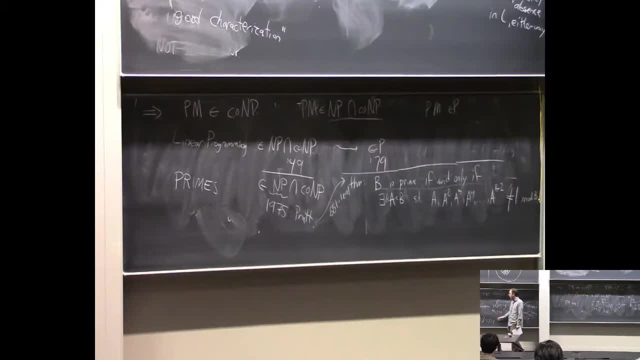 Having no perfect matching is equivalent to the existence of this kind of blocking set S, which doesn't have enough for all kind of matchings. So that's the problem. OK, Let's see if we can get some throughput. OK, So it's a fact that primes is an NP. 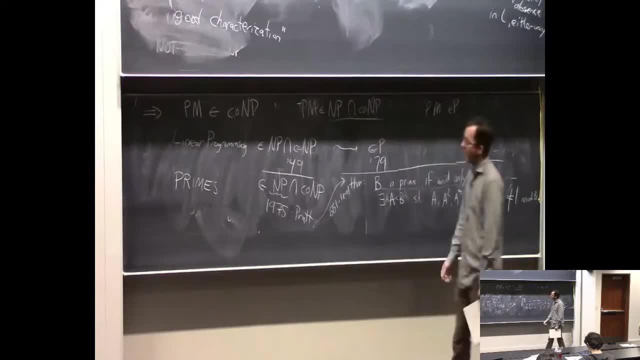 And when I was a student- your age back in the day- University of Toronto- it was common to prove this theorem in complexity classes, because it's an awesome theorem And you'd spend the 30 minutes to do the number theory. 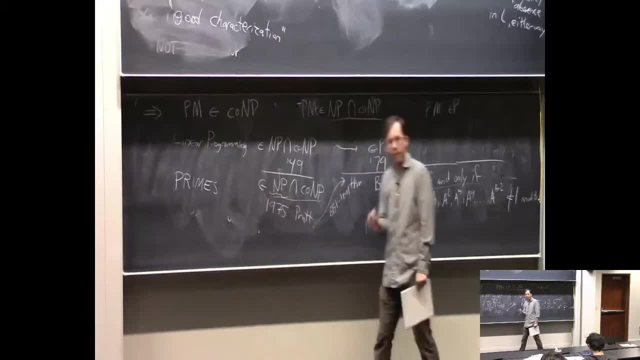 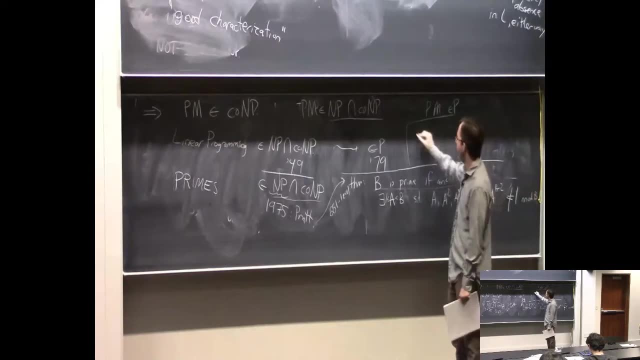 And then you would get that primes is an NP, intersect, co-NP. And that was an awesome fact And people would be like man: it's a very good question: Is primes NP or not? And then they proved that A couple of undergraduates and their advisor. 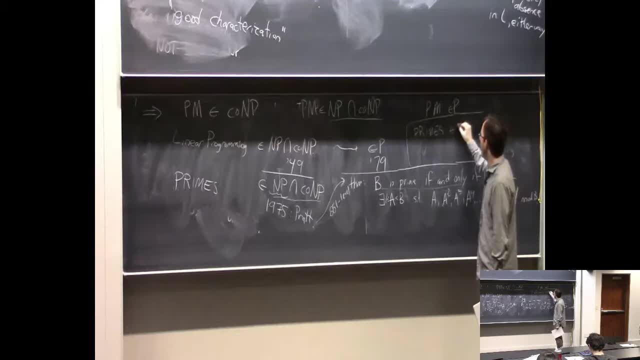 Manindra Agarwal proved this, that it's NP. This was 2002.. So it's another example of first showing that a problem has a good characterization. You can prove when something is prime. You can prove when something isn't prime. 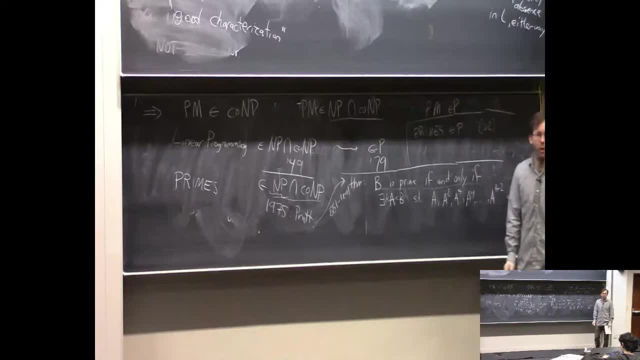 And finally they showed that you can just directly check if a number is prime in polynomial time. But it again took like 27 years or something Great. So we've seen a lot of problems that first were in NP, intersect, co-NP. 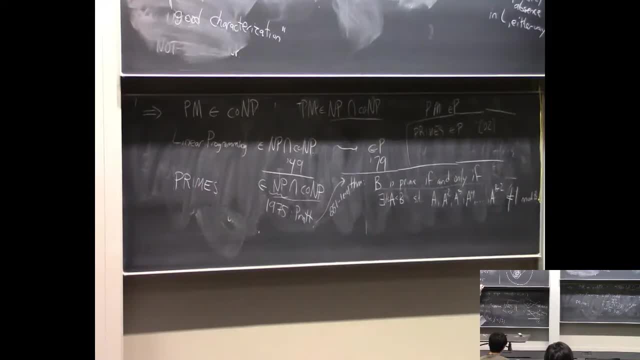 And then eventually they were shown to be NP. I'll now tell you one more problem that's in NP intersect co-NP, And whether or not it's also in P is not known. It's very interesting And it's even a problem that you've seen before. 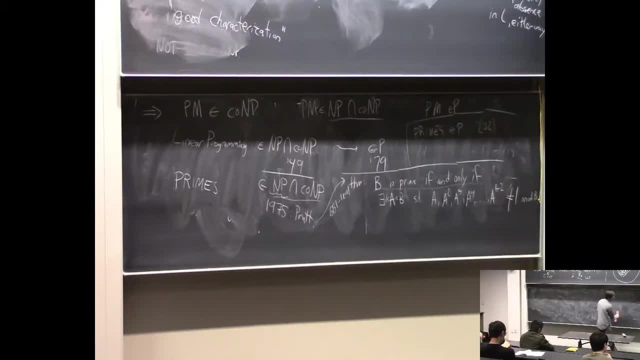 It's on homework one, It's factoring. Well, here's the theorem: Factoring is in NP, intersect, co-NP. Actually, as stated, this is a little bit wrong. So when I say the factoring problem, you normally think I give you a number. 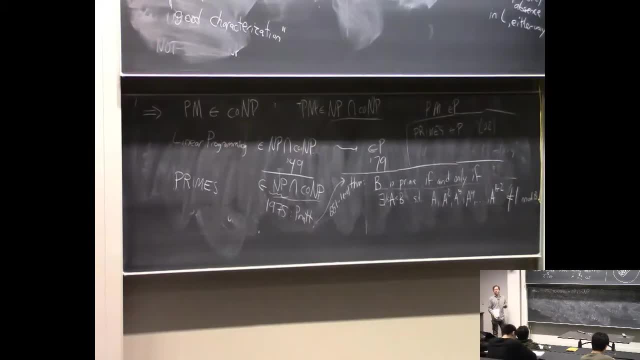 You give me its prime factors. That's a function problem, though It's not a decision problem. So technically it cannot be an NP or co-NP, because NP and co-NP are just decision problems. languages, However, if you remember homework one: 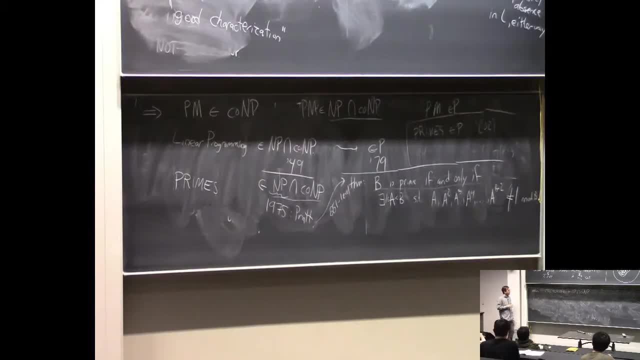 there's kind of a language version of factoring that's sort of equivalent to it from the point of view of polynomial time, So let me scratch this out and call it factor. This was the language, this was on homework- of all the numbers like, let's say, x, a and b. 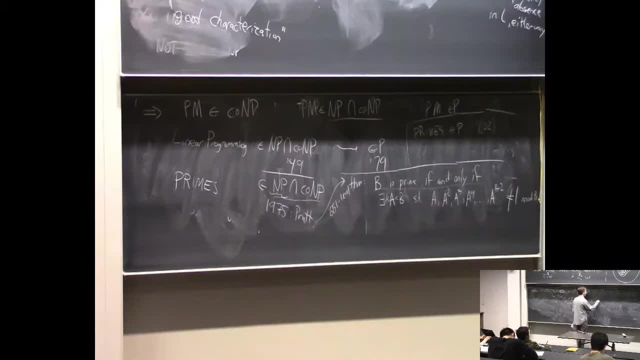 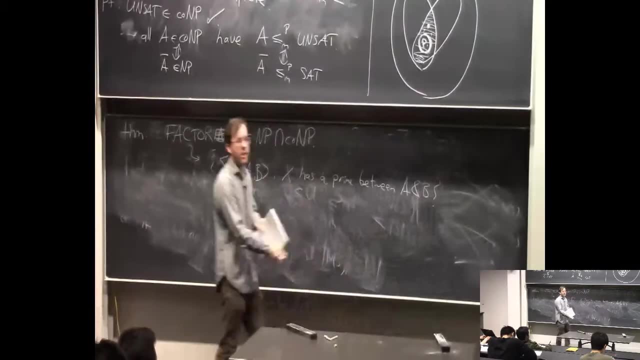 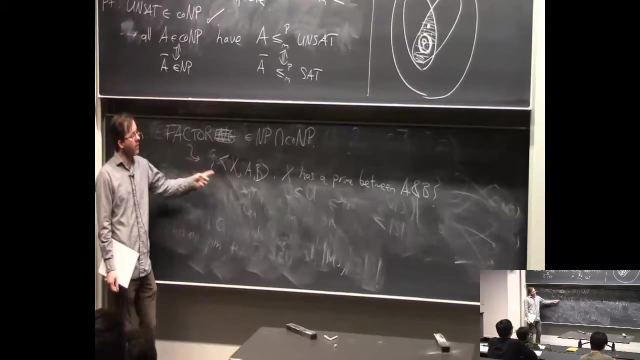 such that x has a prime factor between a and b. And this is a language. it's kind of like an artificially designed language to kind of convert the factoring search problem into a decision problem On homework. we show that if this language is NP, 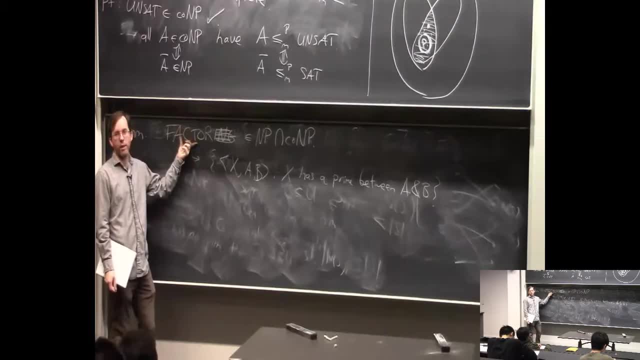 in fact, this language is NP if, and only if, this problem- factoring- can be solved in polynomial time. If you can solve this problem in polynomial time, then you do a binary search and you can find all the factors of a given number. OK, 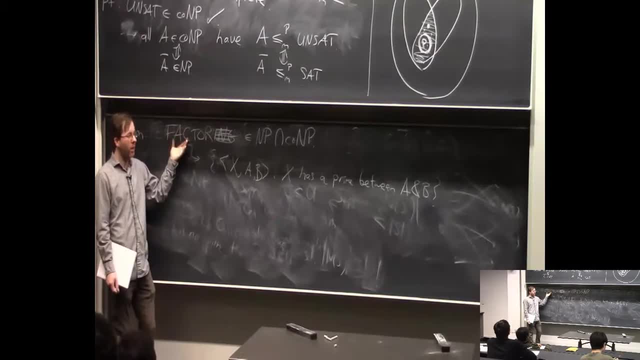 So if you're curious about whether factoring can be solved in polynomial time, it's the same as whether this language can be solved in polynomial time, And you should be very curious about that because the assumption that it cannot be solved in polynomial time 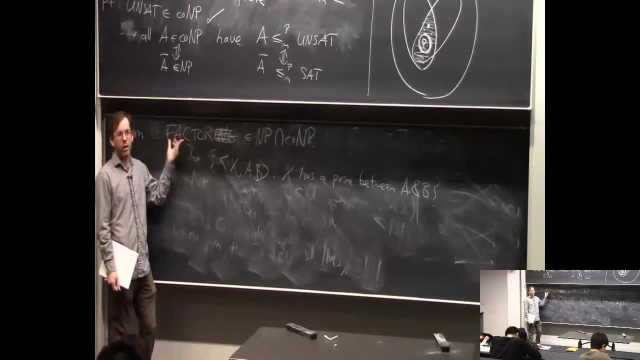 is the basis for almost all cryptography right now, Like RSA, and every time you type HTTPS into your web browser it does some RSA stuff, And the fact that it's secure is based on the assumption that there is not a polynomial time algorithm for factoring. 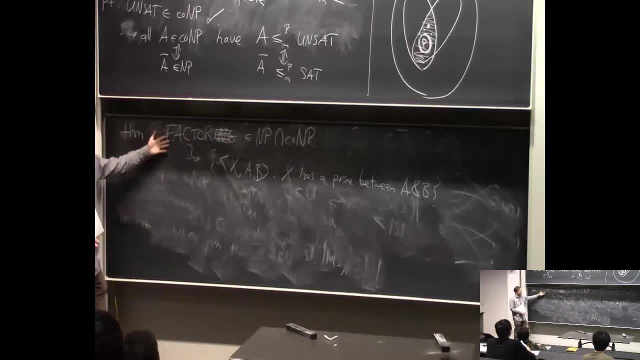 But, as I'm about to tell you, it's not, It's not, It's not. So in a few minutes, it's not that hard Factoring or the factor problem is in NP and it's in co-NP. 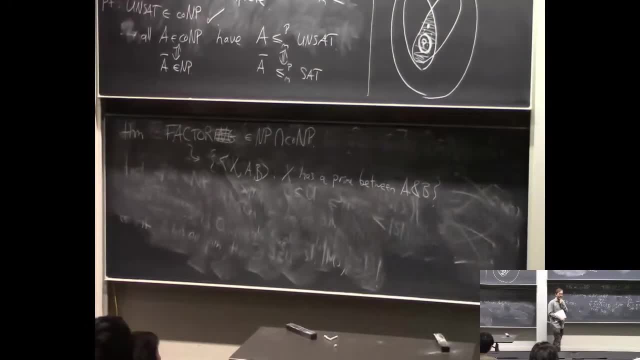 So if you look at the historical record, you might be like, hmm, every time that's happened before the problem eventually, like 30 years later, was shown to be in P. So that's very interesting. I mean, I feel that most people believe the same thing about 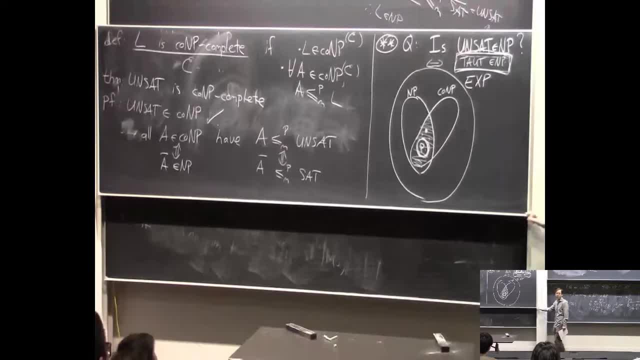 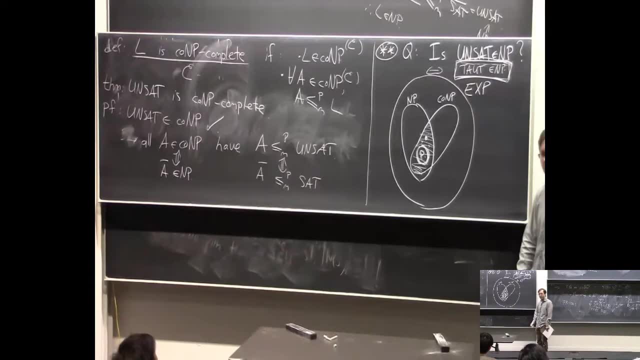 whether or not P does not equal NP, But I'm not sure most people believe the same thing about whether or not factoring is in polynomial time. I think most people believe factoring is not in polynomial time. At least they're putting their money where their mouth is. 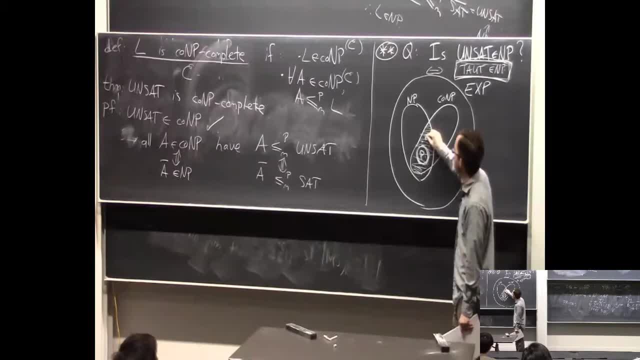 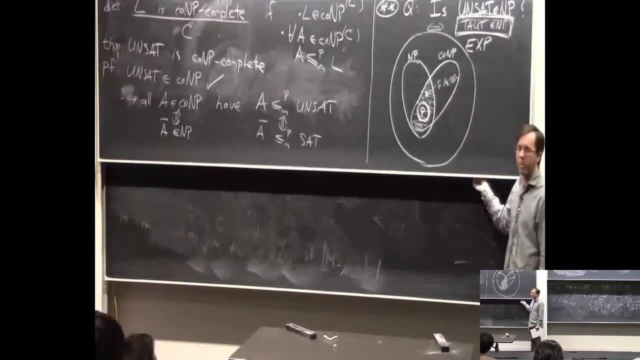 when they're buying stuff on the internet, Because the cryptography is based on the assumption that factoring is not in here. But we'll see. Maybe we'll wake up tomorrow and a couple of undergrads from CMU will have proved that factoring is in P. We don't. 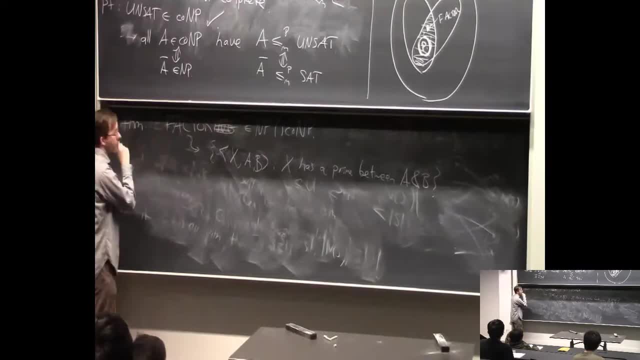 know, But OK, I have two minutes left. I'll show you that factoring is in NP, intersectionally, Intersect, co-NP. It's quite a nice proof. So let's first show that it's in NP. This one's a bit easier. 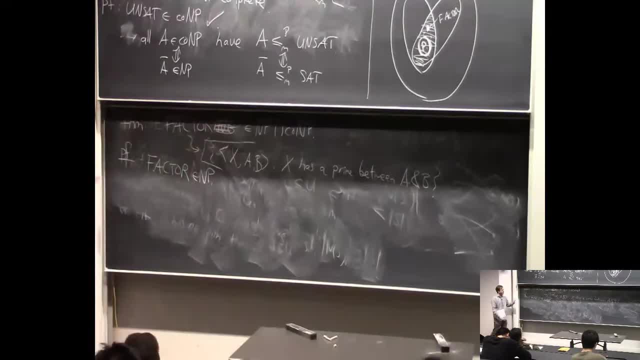 So this language, I claim it's in NP. I give you x, a and b. You want to know, is there a prime factor of x between a and b? So why is this in NP? Yeah, So the certificate is the P. Now, actually there's a few. 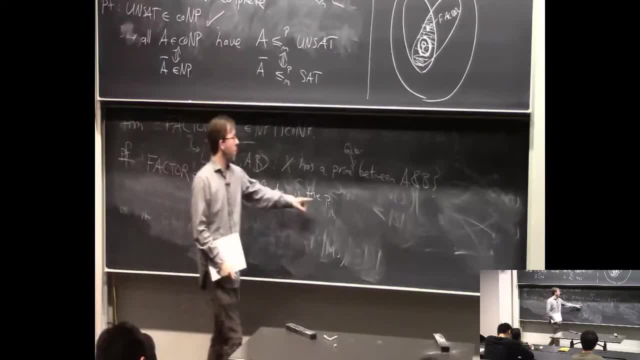 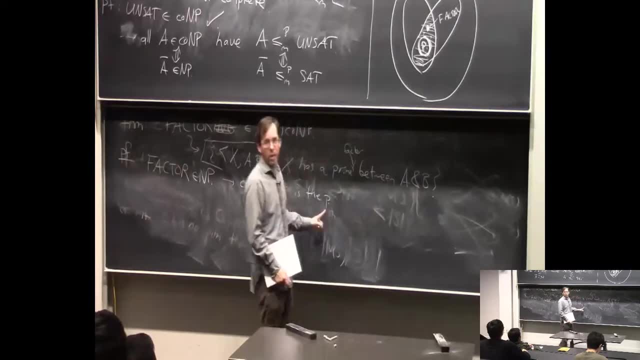 things that the verifier has to check here. First it has to check that P divides x. That's OK. That's a division problem. It's polynomial time, That P is between a and b, That's easy. It also has to check that P is prime. 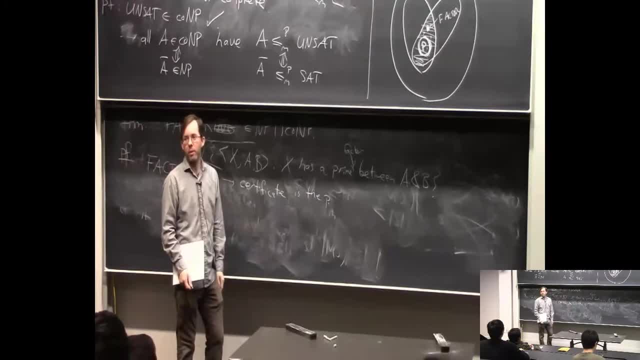 Now we know actually now that a verifier can check if P is prime in polynomial time. But it was actually even fine back in the olden days, Because back in the olden days we knew at least the primes by Pratt was in NP. 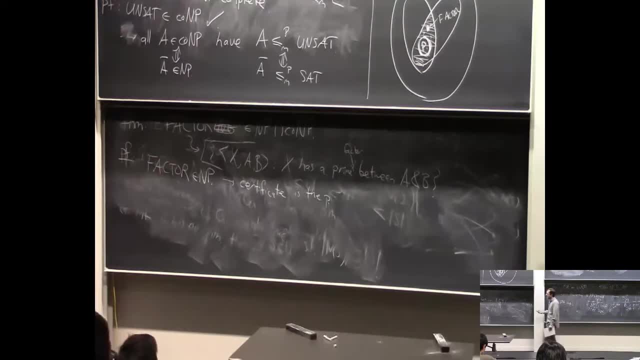 So there was a way to certify that a number was a prime. So in the olden days you had to not only give P, but you had to give the Pratt certificate that P is a prime, which is fine. Now, in this modern age, we can just say: well. 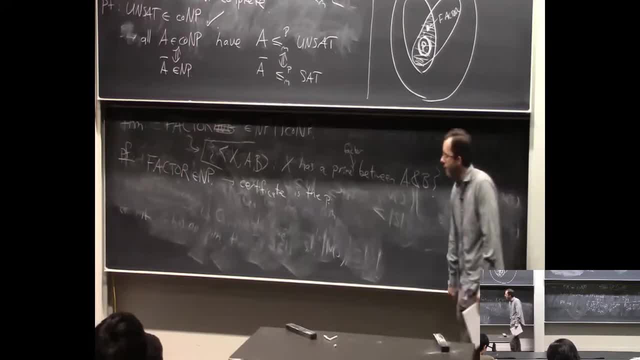 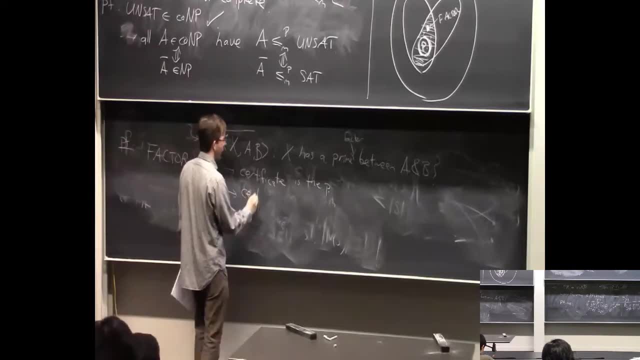 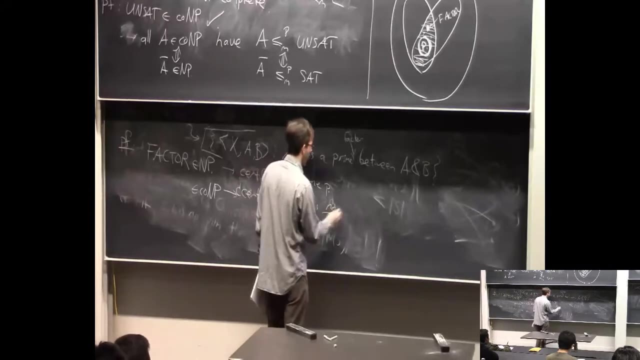 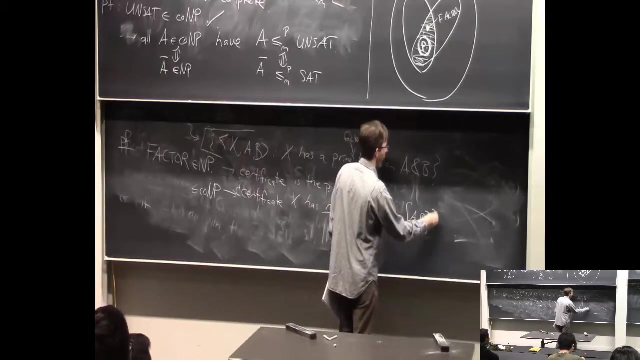 you can check yourself. verifier that this number is prime. OK. And why is it in co-NP? So right here we have to come up with the certificate that x has no prime factor between a and b. Can somebody say why this is in NP? 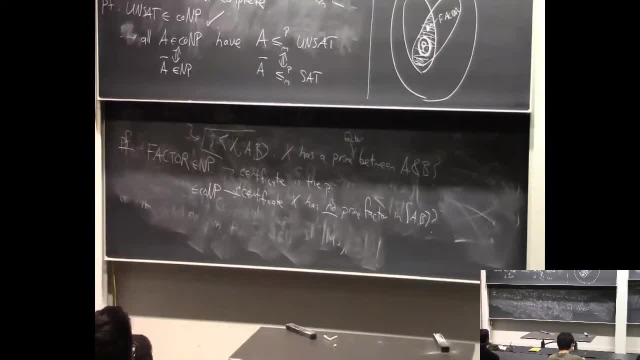 Like how you can certify this If I want to convince you that some number does not have a prime factor between a and b. At first it looks tricky. OK, I'm out of time so I'll just say: At first it looks tricky. 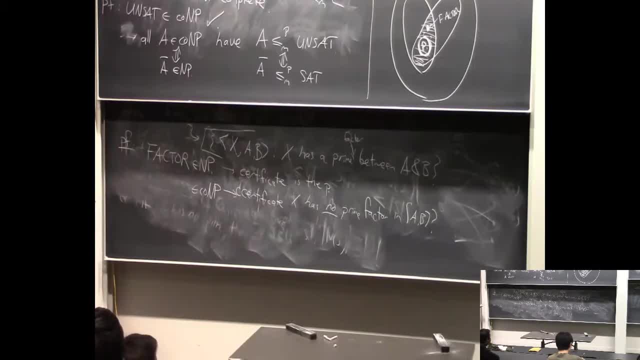 Because you're trying to claim that, like there's all, the numbers between a and b are not prime factors of x. But you can remember a theorem from elementary school: Every number has like a unique prime factorization. So the certificate you give is just.